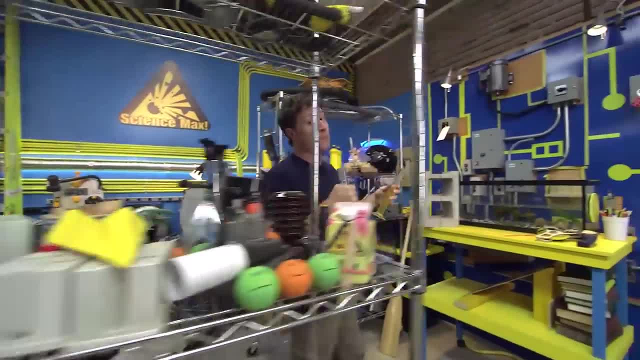 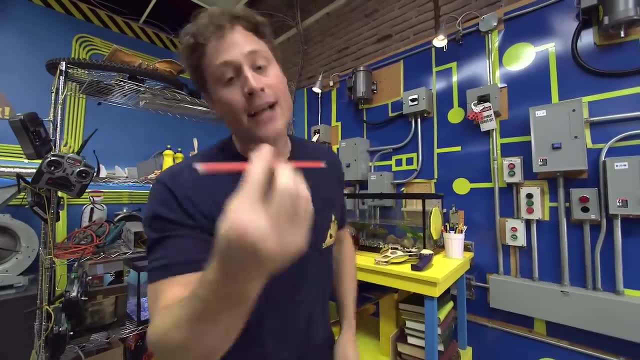 Chemistry is the science of atoms and molecules, the things that make up all matter, and how they interact with each other. Take, for example, this glow stick. Actually, don't take it, because I kind of need it. The glow stick doesn't glow until you. 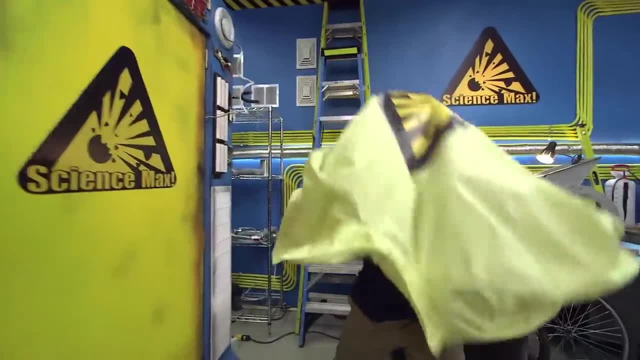 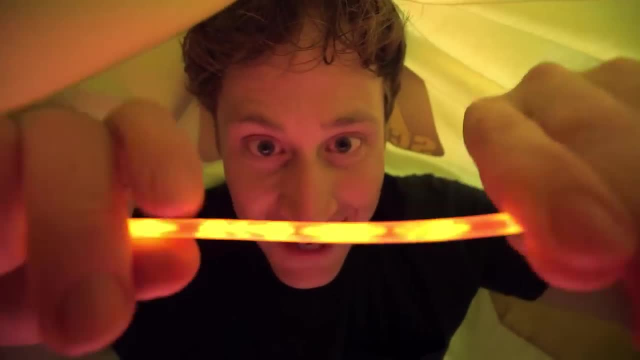 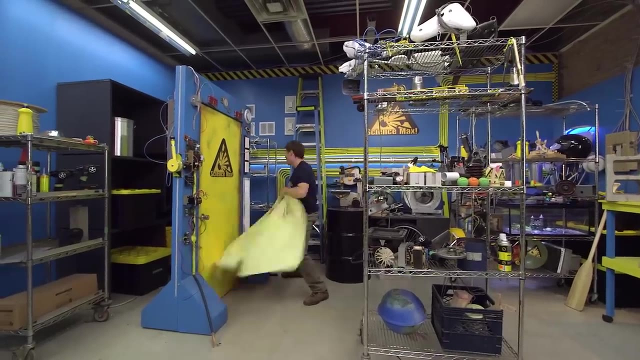 Um, The glow stick doesn't glow until you break the barrier and mix the two chemicals and they start to glow. Huh, Pretty cool, huh? Chemistry. Now, the chemical reaction we're looking at today is the old vinegar and baking soda volcano. 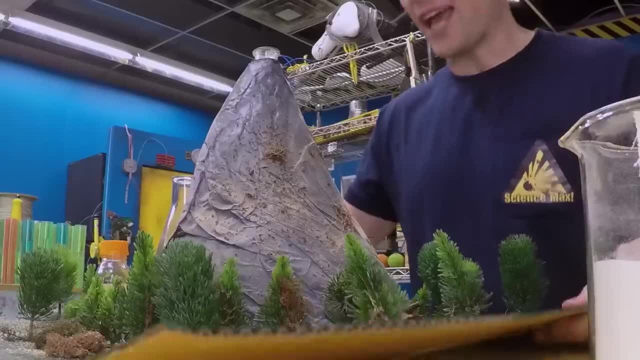 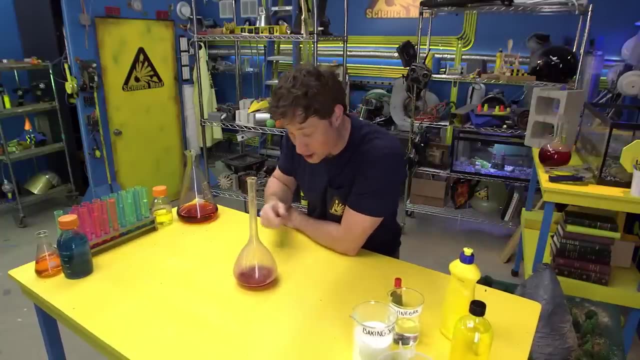 But this reaction doesn't have anything to do with volcanoes, It's chemistry. Now, this experiment is totally safe, but I do recommend you get an adult's permission before you do it, because it's very messy. Uh, Uh, Yeah. 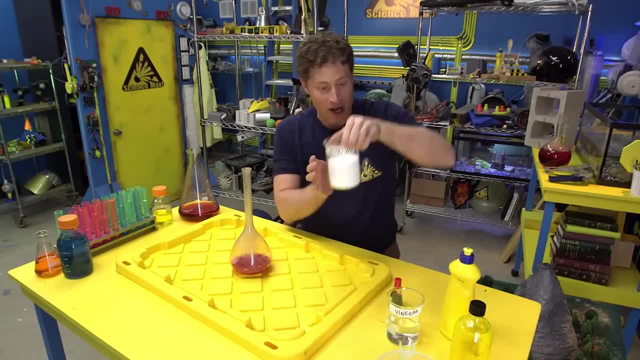 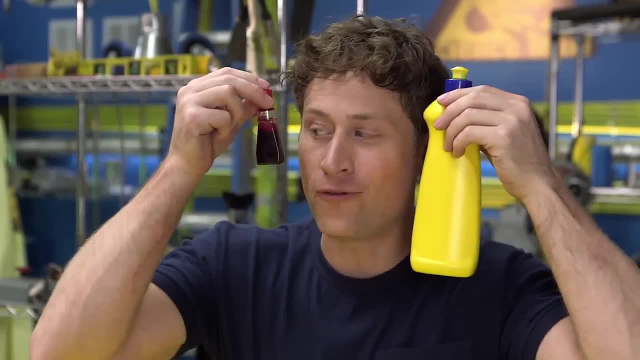 Ha-ha. First, you're gonna want baking soda and vinegar. These are your two main ingredients, But you'll also want dish soap and red food colouring if you want it to look a little bit more like lava. Now I like to mix the baking soda- red food colouring. 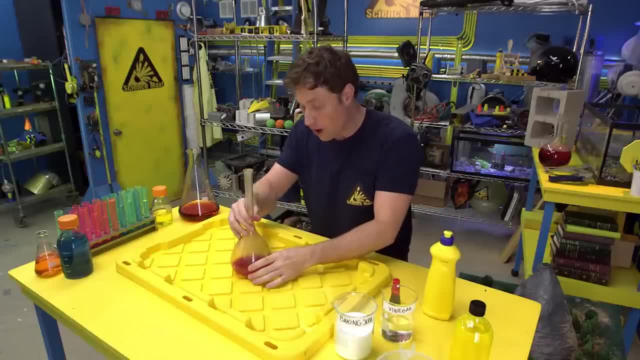 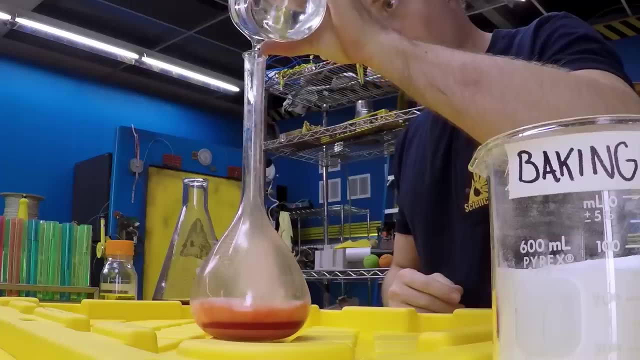 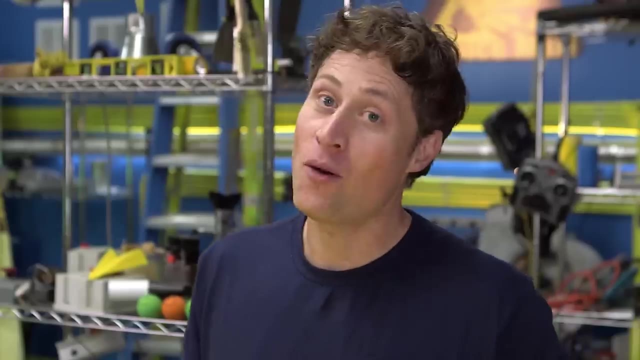 and dish soap together with a little warm water. so all you have to do is add the vinegar, And when you do this is what happens, And there you go: Chemical reaction. Now I know what you're thinking. You're thinking. 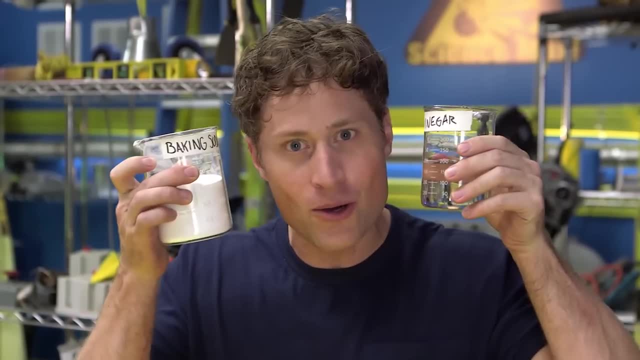 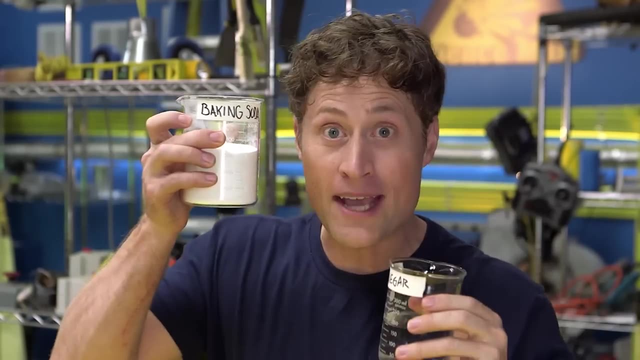 Phil, how much vinegar or baking soda do I use? Well, I'm not gonna tell you. This is where you can be science maximites. Try different amounts. More vinegar, more baking soda, More dish soap- Who knows? Write down the amounts each time you use it. 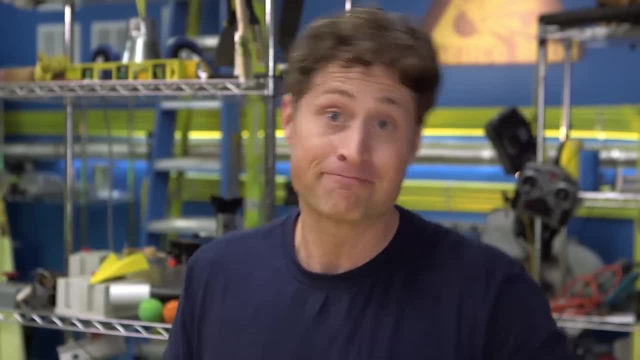 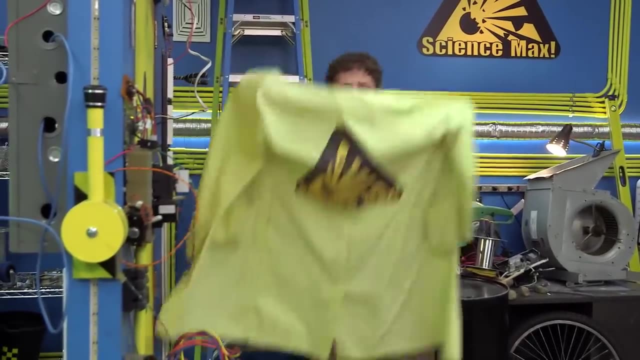 and find out what amounts work best. That's called science And that's what we're gonna be looking at today: Chemistry in all its forms And, of course, because it is Science- Max experiments at large. we're going to max out the vinegar and baking soda volcano. 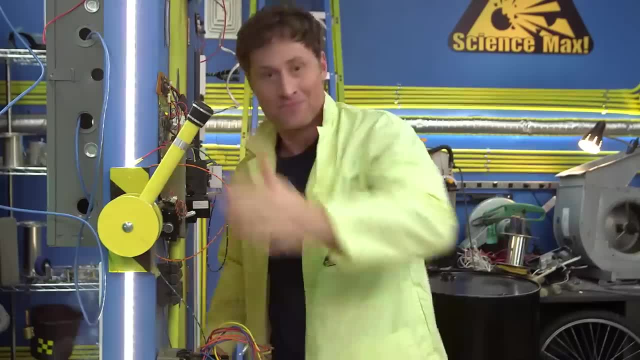 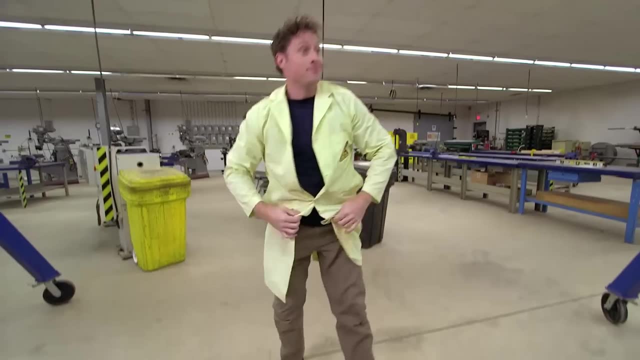 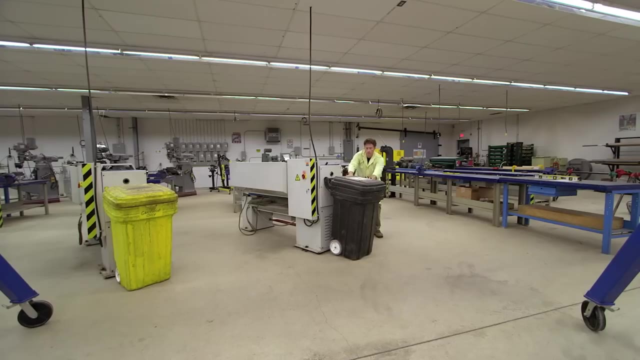 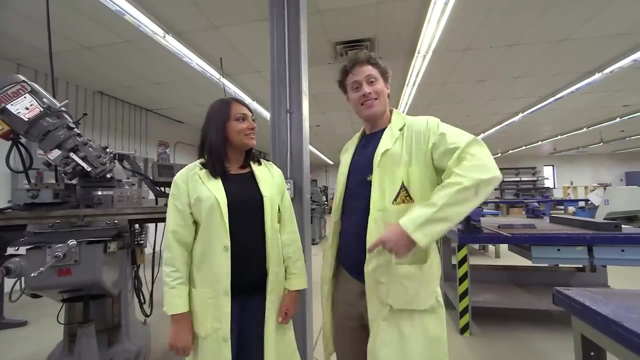 So I'm off to the Centre for Skills Development and Training. Come on, Hey Talena. Hi Phil, How you doing Good? How are you Good? This is Talena. She's going for her PhD in chemistry from McMaster, right? 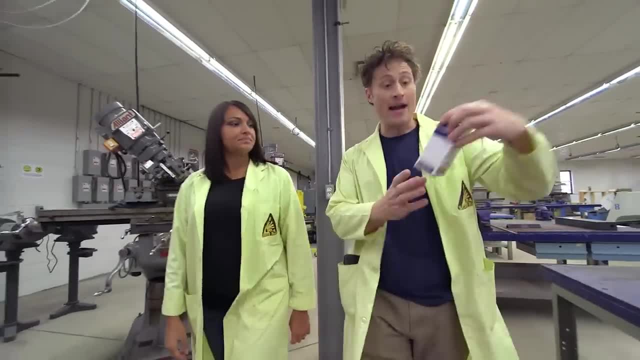 Yep, Awesome, Which means you can help me max out the baking soda and vinegar We need. Can you grab that vinegar And vinegar volcano? So what happens when we mix these two chemicals? Well, vinegar is an acid and baking soda is a base. 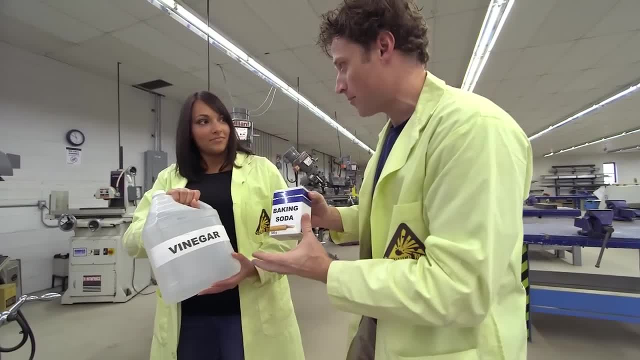 And when you mix them, they neutralize each other to produce carbon dioxide and water as a byproduct. Hmm, So acid and baking soda. what happens when you mix these two chemicals? Well, vinegar is an acid and baking soda is a base. 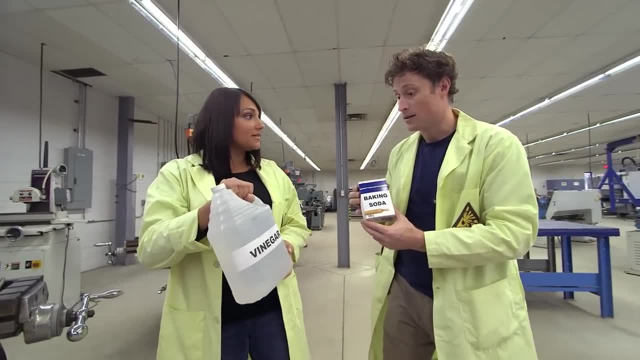 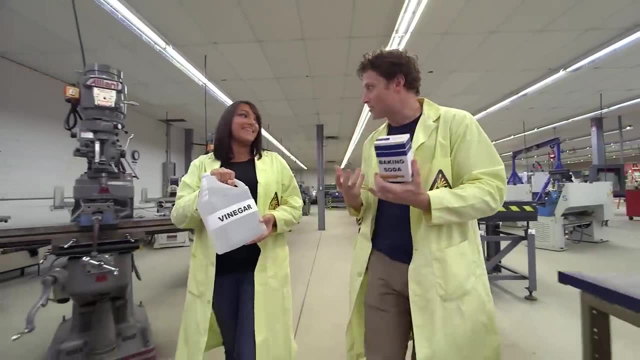 And when you mix them they neutralize each other to produce carbon dioxide and water as a byproduct. Hmm, So acids and bases are kind of like opposites, Yep, So I guess that makes sense. When you put them together, crazy stuff happens. 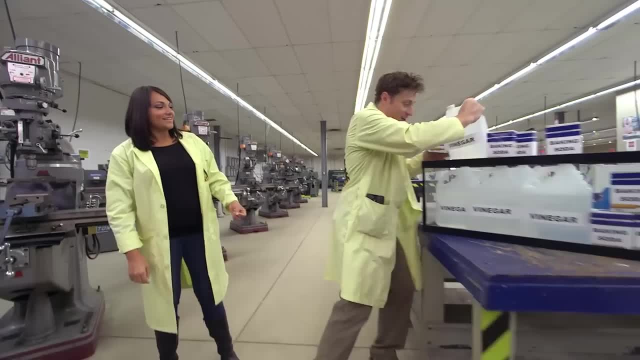 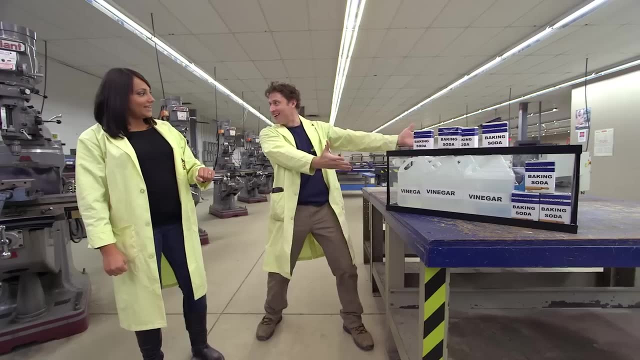 Yeah, Awesome Chemistry. Okay, So I want to use this much vinegar and this much baking soda. What's with the fish tank? The fish tank is where I want to mix it all together. What do you think? Awesome, Maxed out. 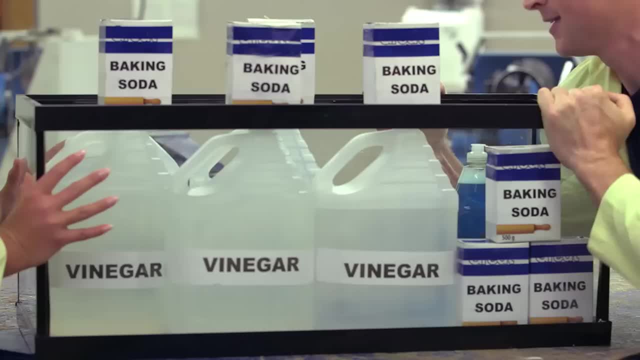 Okay, Let's move the fish tank somewhere where we won't make a huge mess. It's a little heavy with all that. We're going to. No, We're going to have to. No, We're going to have to. That's it. 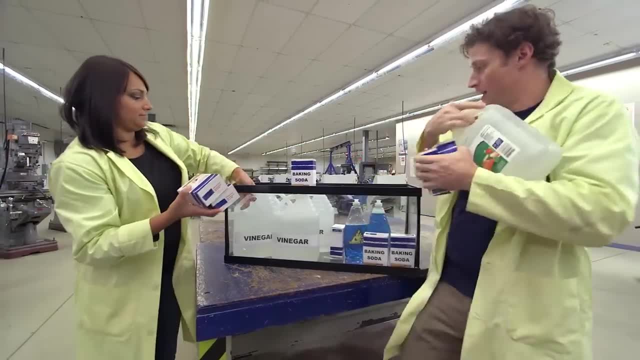 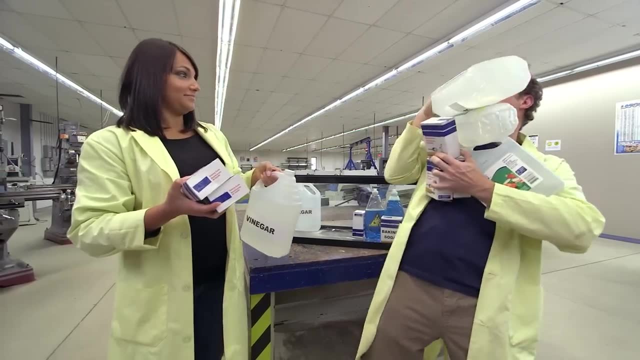 We're going to have to take a couple trips. That's kind of heavy, Okay. So we'll take this and that and then this and then that. No, hold on, I can do it One more. Okay, good, Okay, good. 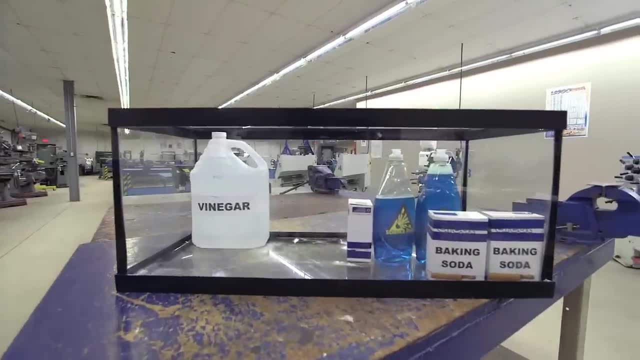 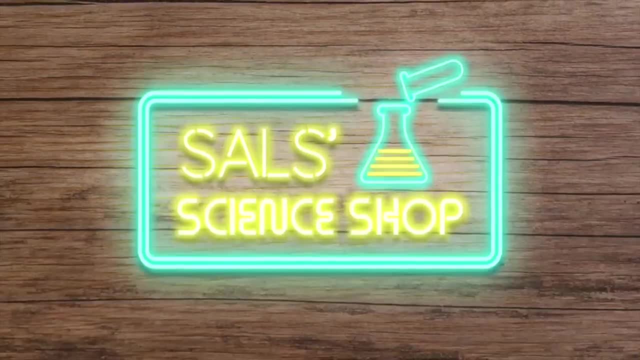 Yeah, I took too much. I took too much. Uh-oh, Uh-oh. That's good, Ramona. Put it in the, Put it in the background, Put the side of the. Put it in the. Put it in the. 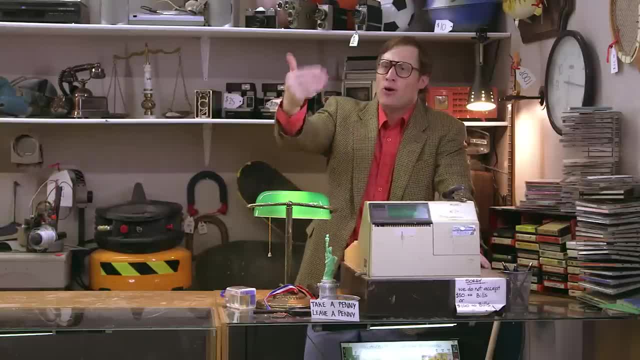 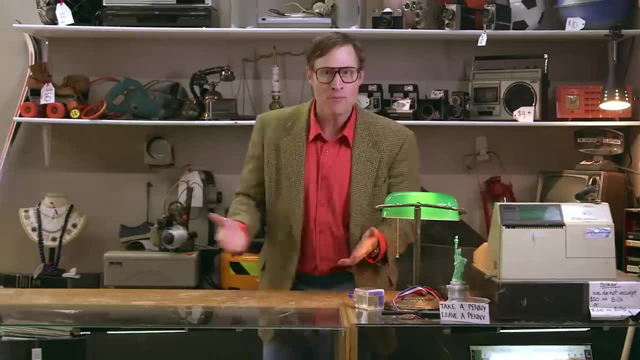 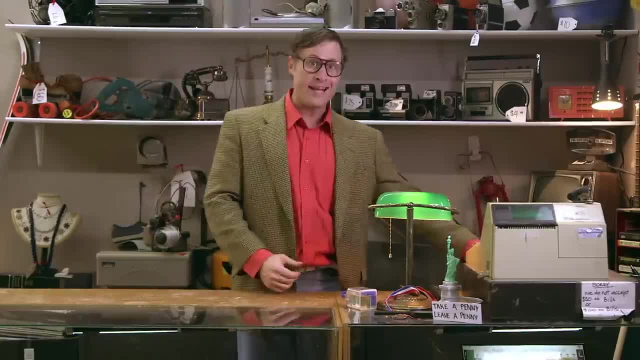 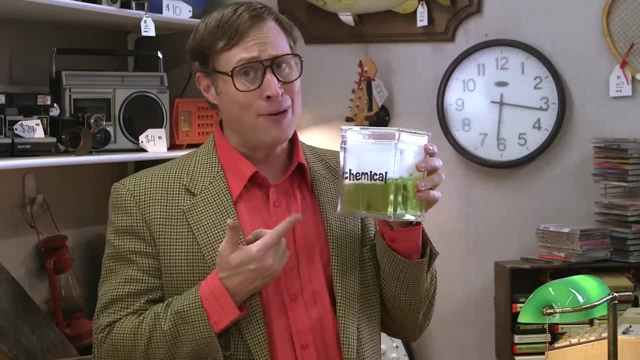 Chemicals, Chemicals- What are chemicals? Are they things you have in a lab, in a jar that say chemical on them? Well, yes, But if that's all you think chemicals are, then you need to know your chemicals. Turns out the stuff. 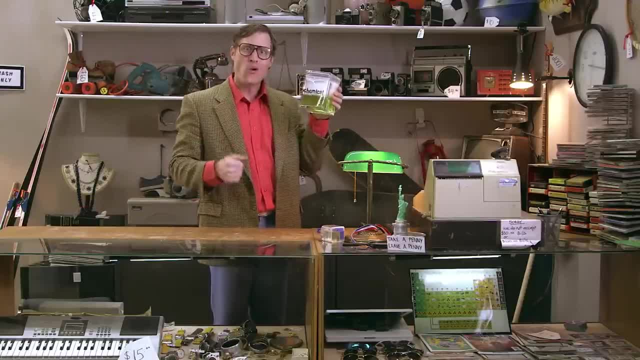 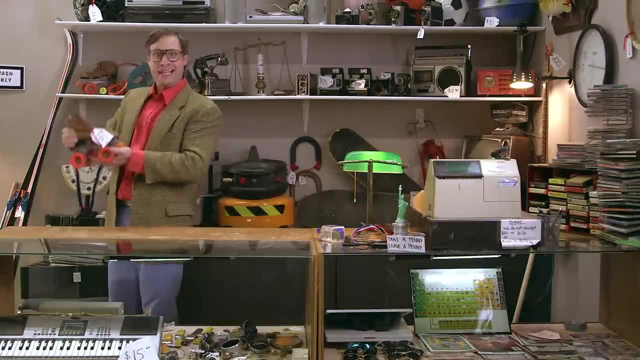 in the jar is a chemical, but the jar itself also made of chemicals. The table I'm putting it on made of chemicals. My lunch: Chemicals- Chemicals. Roller skate Chemicals. My jacket Chemicals. This guitar. 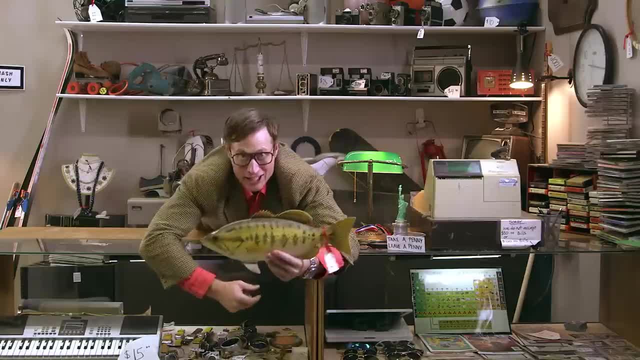 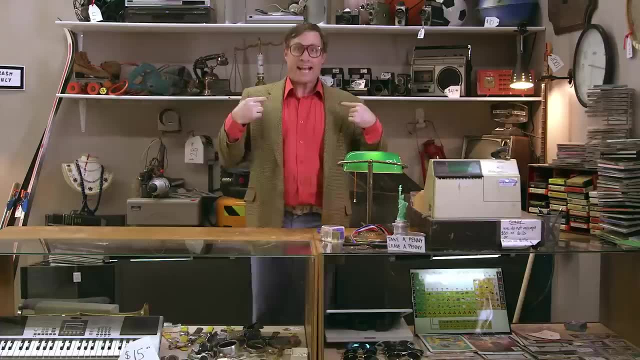 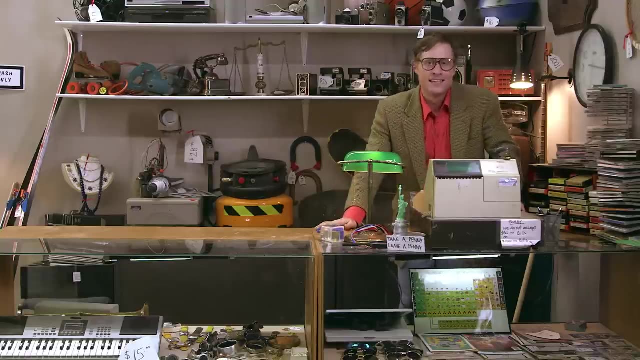 Chemicals: My shoe Chemicals, This watch Chemicals, This fish Chemicals. Chemicals, Chemicals, Chemicals, Chemicals, Chemicals, Me Chemicals, You Chemicals, Ramona Chemicals. 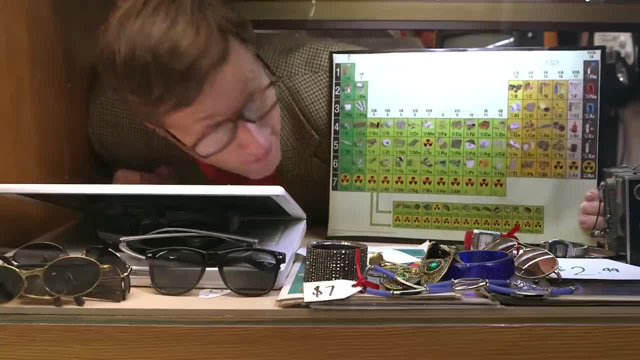 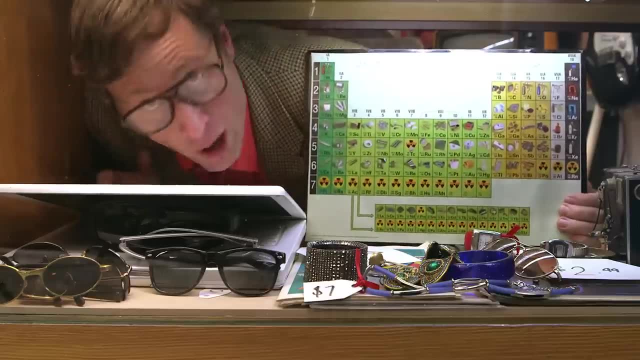 No, I said your chemicals, Chem, Never mind, This is it. The universe is made up of these pure elements. They go together in different ways to make up everything, All matter. Think of it like building blocks. These little atoms are some of the elements. 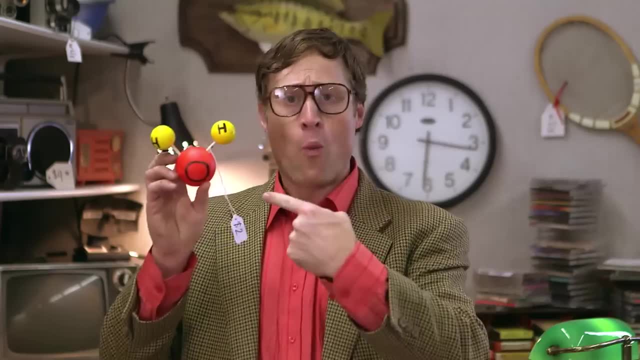 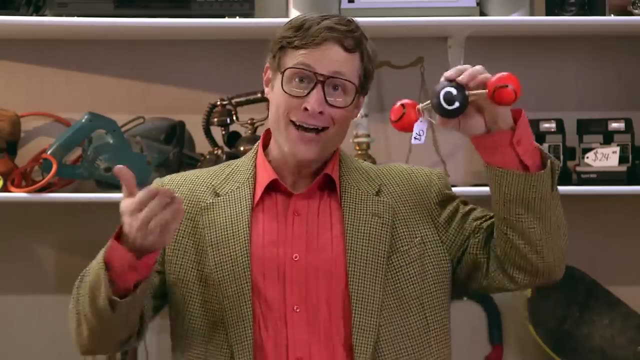 on this periodic table. You got one oxygen, two hydrogen. bam, you got a water molecule, One carbon, two oxygen. hey, it's carbon dioxide. Two carbon, two oxygen, four hydrogen. skadoosh vinegar: One sodium. 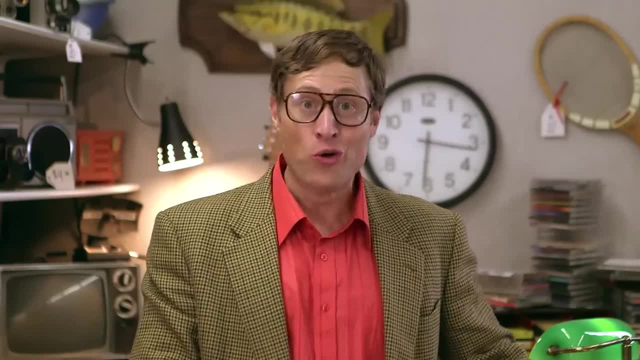 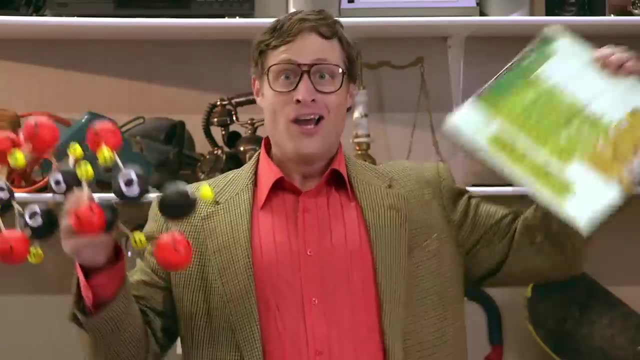 one chlorine. hey, what's up All matter in the universe is just the stuff on here combining into these. And now you know your chemicals. Mmm sugar. Let's take a closer look at what's going on when we mix vinegar. 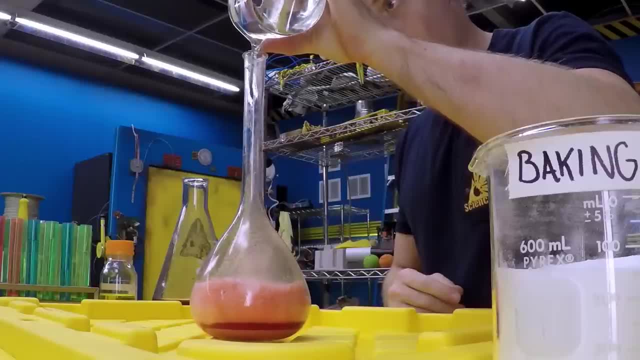 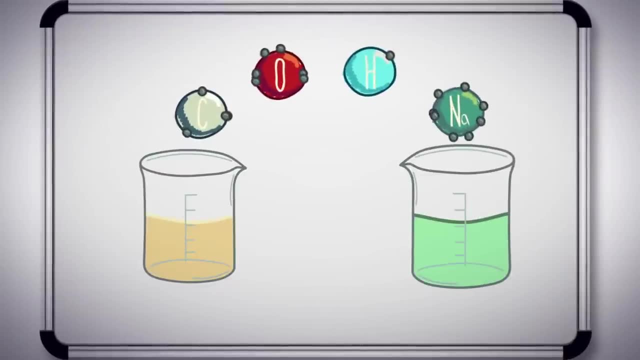 and baking soda. All chemicals are made of atoms. There's only four types in our reaction: Carbon, oxygen, hydrogen and sodium. When we mix hydrogen, sodium, hydrogen, hydrogen and sodium, we get sodium When they go together. 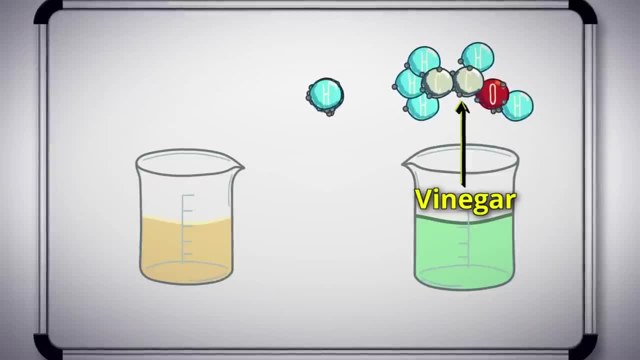 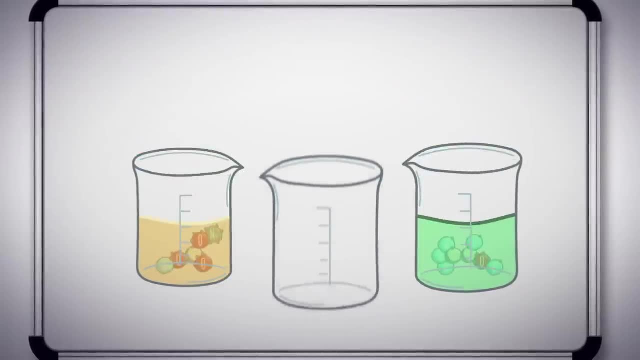 like this: this is a molecule of vinegar or acetic acid And this is a molecule of baking soda or sodium bicarbonate. When chemicals react, they switch atoms. That one goes there, this one goes over here, and then this one. 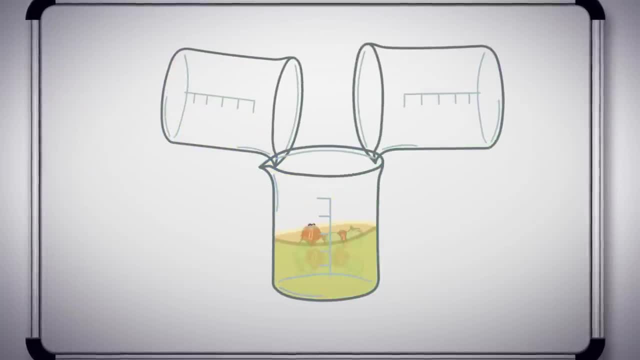 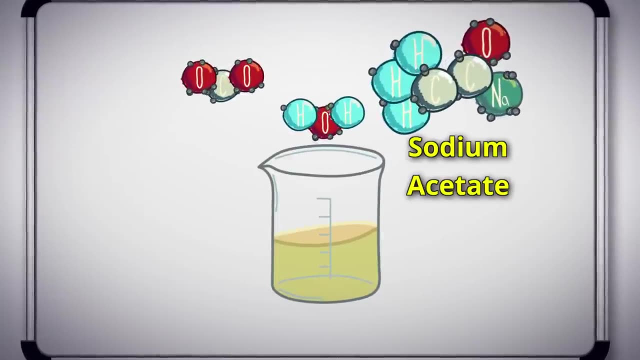 turns into this, and then what you end up with are new molecules. This one is called sodium acetate and this one is carbon dioxide gas, the gas you breathe out. And do you recognize this one? Well, this one is called sodium acetate. 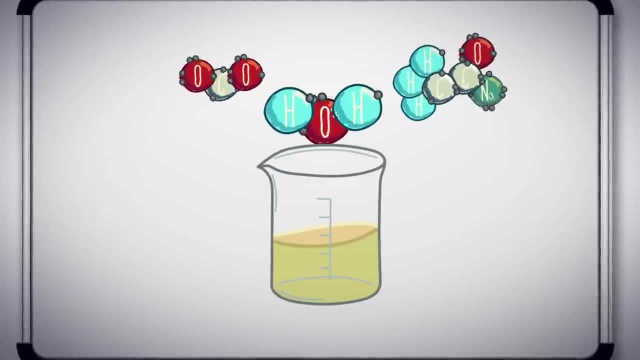 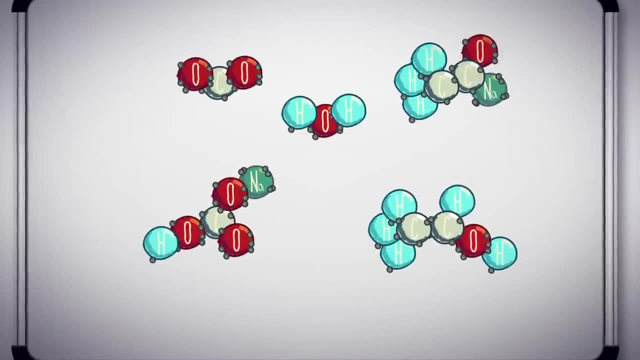 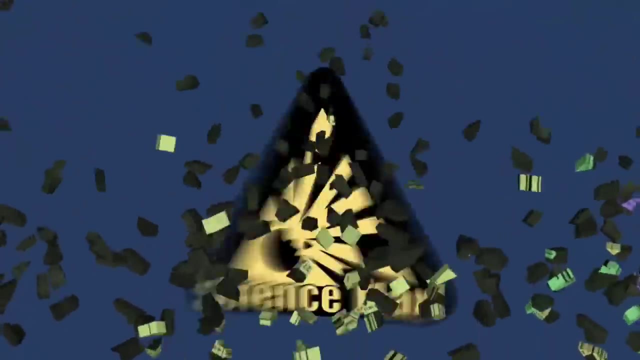 and this one is carbon dioxide gas. and do you recognize this one Right? water, H2O. Why all this happens gets complicated, but the study of chemistry is all about how molecules are built and react with other molecules, All right. 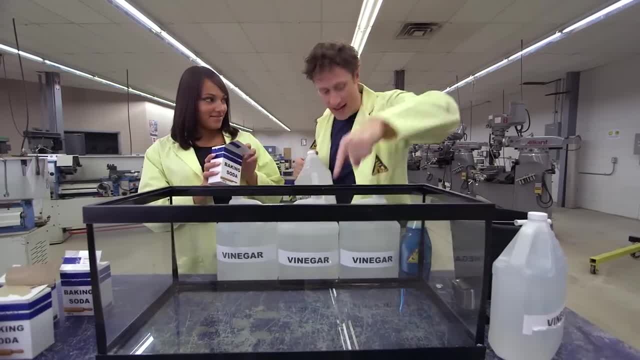 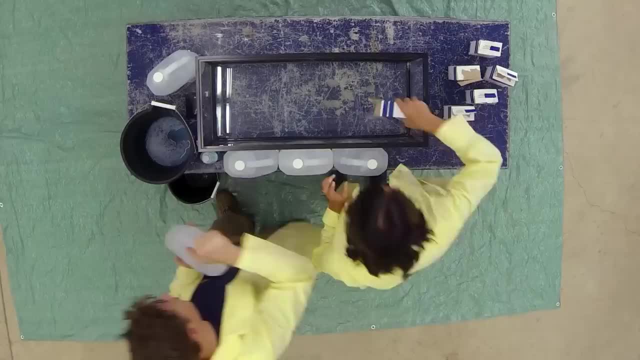 Talena, you ready? Yep. You're going to pour all your baking soda in the fish tank and I'm going to pour the vinegar into this bucket, because you don't want to pour them together right away. Okay, you ready, Yep. 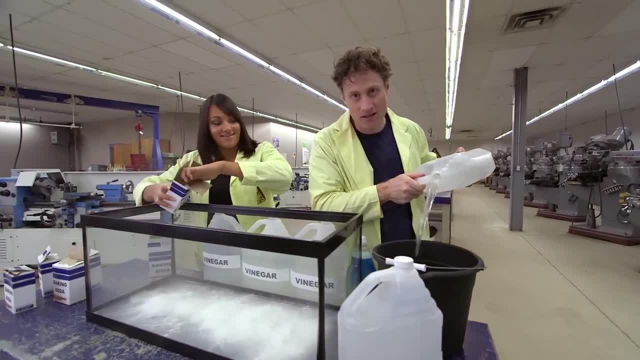 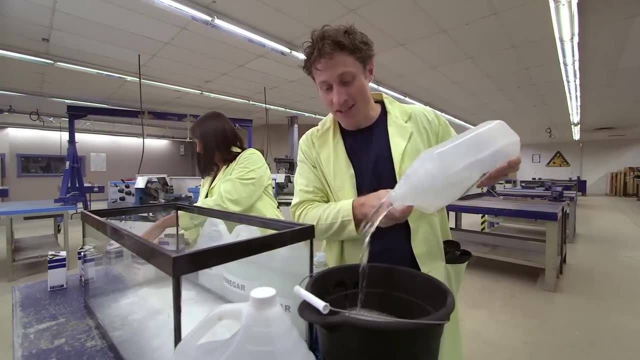 When you're doing your PhD in chemistry, do you get to do stuff like this? Yeah, Really, I get to do a lot of fun reactions in the lab. Oh, that's, I'm jealous. Have you ever done this much vinegar? 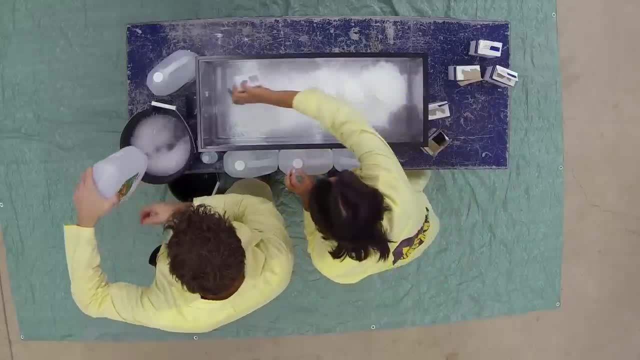 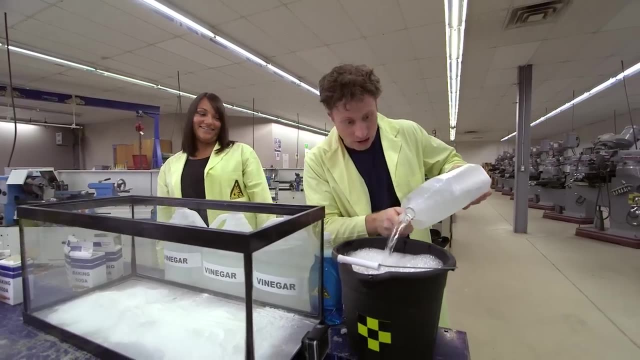 in baking soda in one time. I can't say I ever have. There you go. That's what I like to hear. I already put the soap in the bucket so it would mix with the vinegar when I poured it in. Are you done? 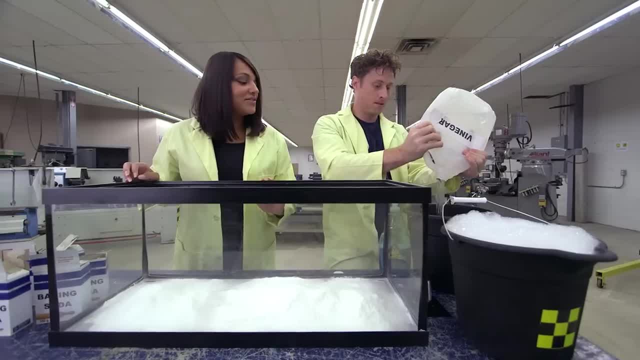 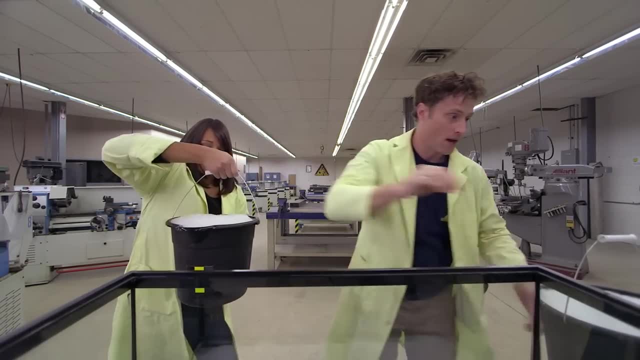 your baking soda. already I am. I'll pour faster, Oh faster. It smells vinegary. I don't want french fries. Okay, Talena, you take this very full bucket of vinegar and dish soap. Thank you, I will take this one. 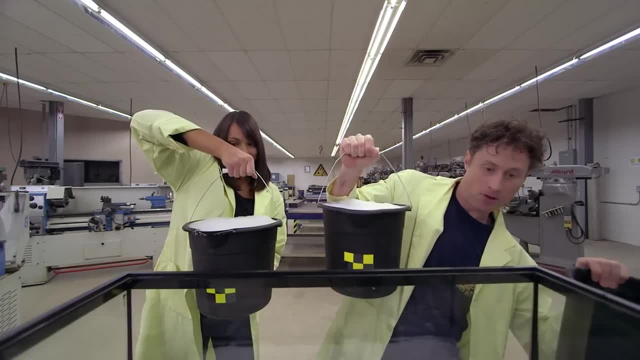 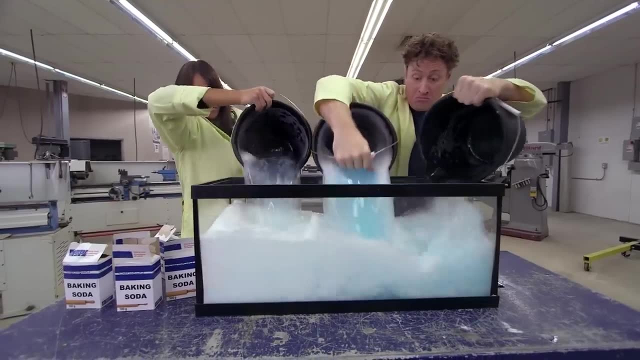 Uh-oh, we still have our third bucket. Okay, I'm gonna. I'll do these both at the same time. Okay, Ready On the count of three. One, two, three, Whoa, Whoa, Whoa. 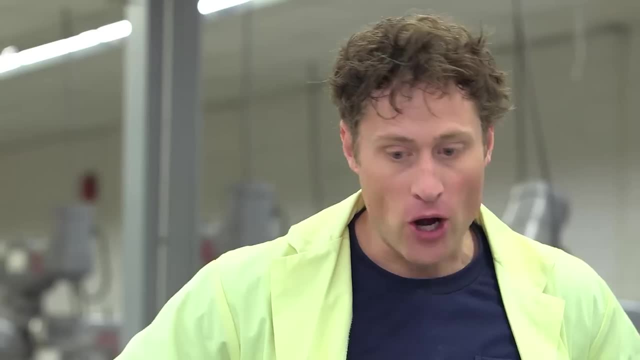 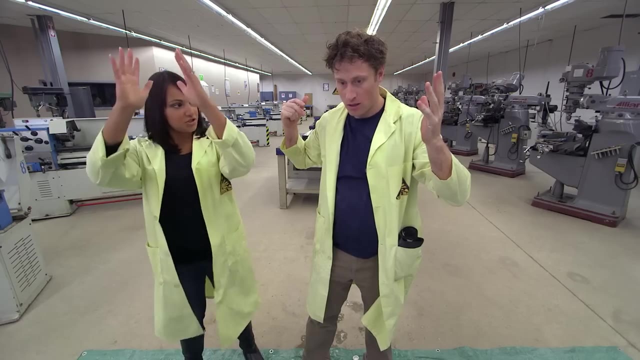 Okay, That's awesome. So the one thing it didn't do: it didn't shoot up in the air, though Yeah, it's because the top is quite open, so you would need to constrict it to get it to shoot up. 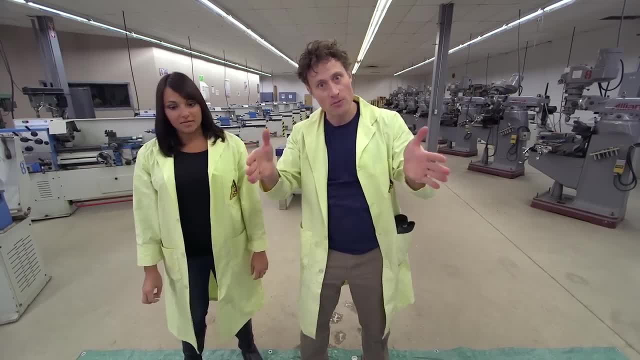 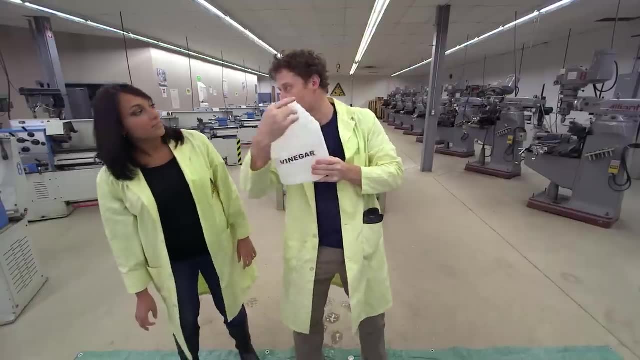 Oh yeah, because we're using just sort of a square Mm-hmm a rectangular prism container. we should get something that's maybe something more like our vinegar bottle. right Yeah, Because there's lots of space down here. 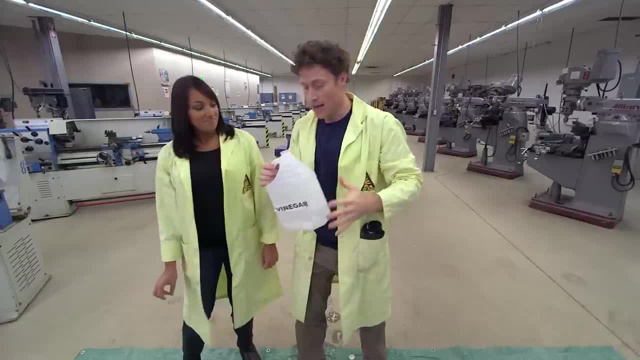 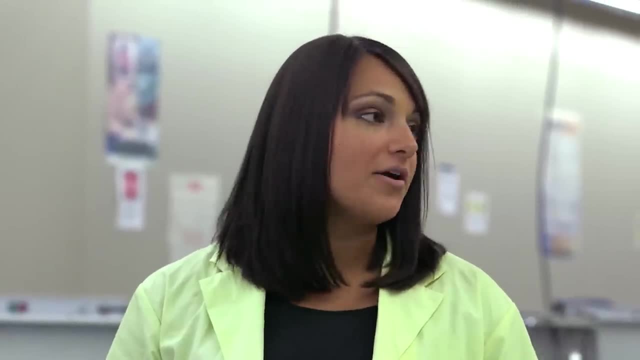 but then it forces it into a tighter opening at the top there, um, like a volcano, Yeah, And what else can we do, uh, to make it even more powerful? to max it out? Well, vinegar is only 5% acid. 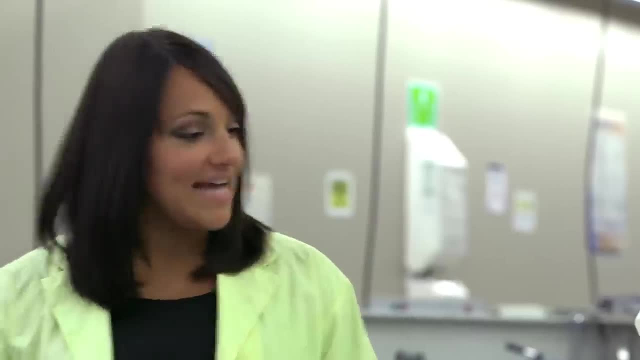 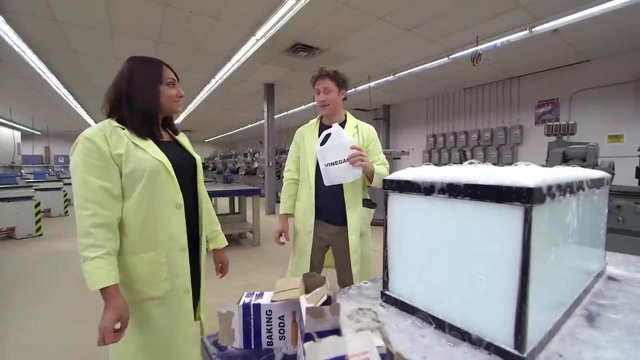 The rest is water, so you could try using 100%. So what kind of acid is vinegar? It's acetic acid. So vinegar is actually only 5% acetic acid, Yep and 95% water, So you can get. 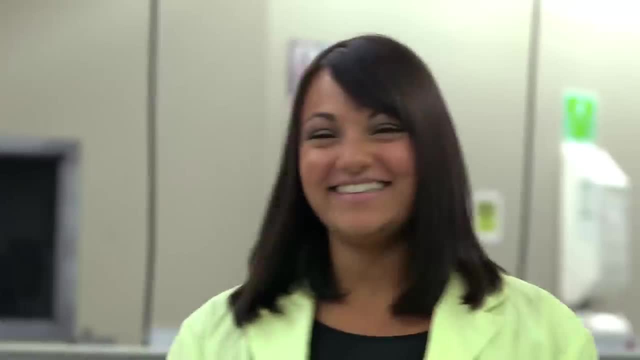 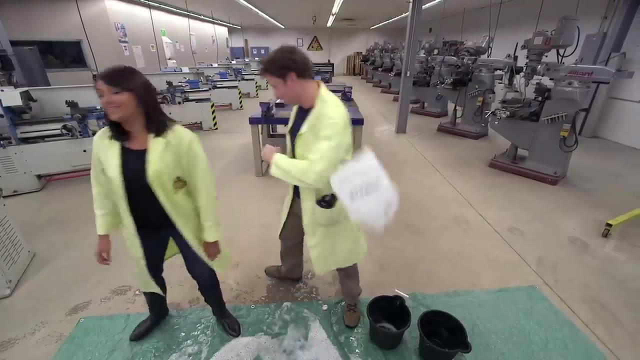 100% acetic acid. Yeah, Can you get 100% acetic acid? Yes, Awesome. Why don't we get a container that's sort of shaped like a funnel, like a volcano? Yep, and 100% acetic acid. 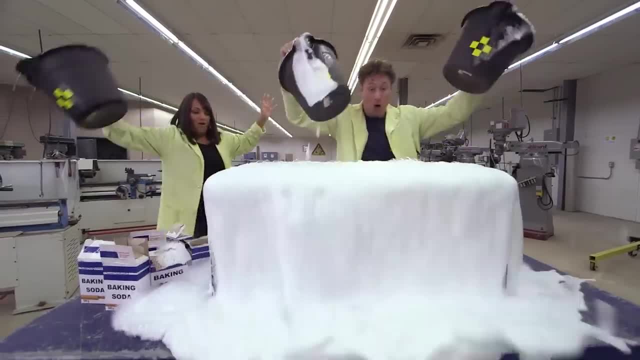 and we'll do it again. Sounds good. All right, let's do it. Our vinegar solution went pretty well, but now we're gonna try it with a much stronger type of the same kind of acid you find in vinegar. Ooh, 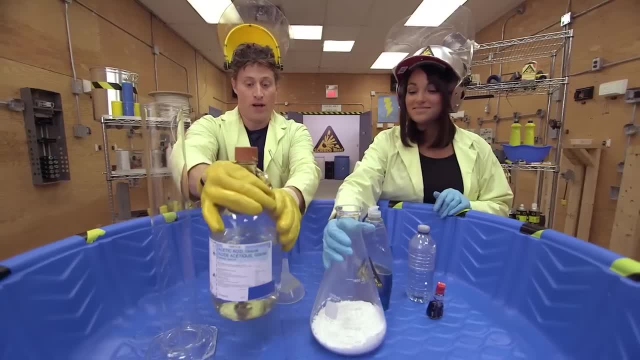 Carefully putting this down And watch out for the baking soda. You never know when it'll get out. And well, I guess that's just baking soda. huh Yeah, that's pretty safe. Yeah, okay, good, So this is. 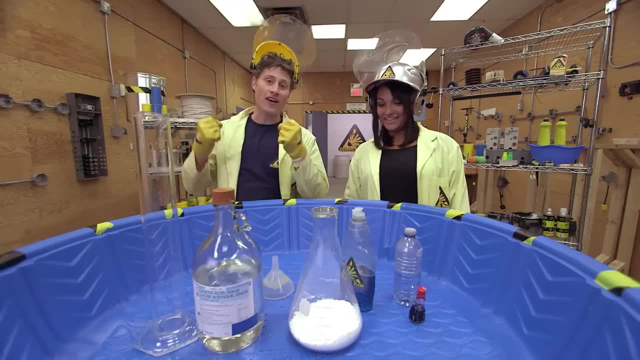 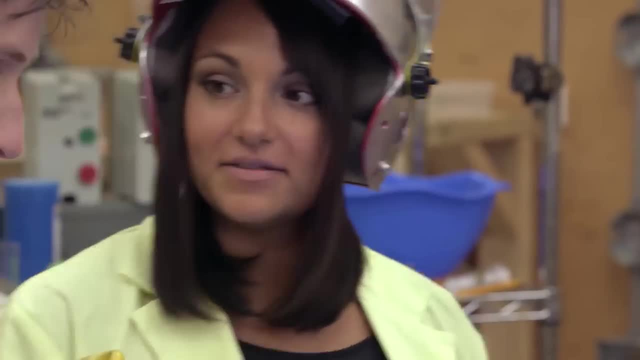 Baking Soda Vinegar Volcano Version 2.. We have this differently-shaped glass. What do you call this? again? That's an Erlenmeyer glass. Why is it called that? It's actually named after a scientist. Did he look like that? 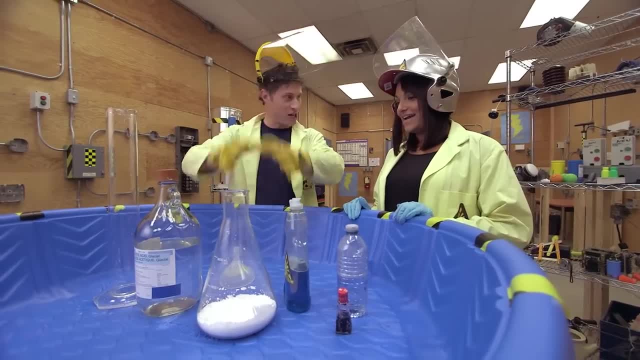 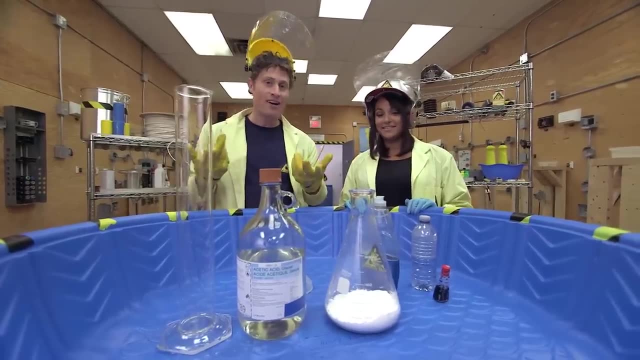 Yeah, It's actually named after a scientist. Did he look like that? Was he sort of shaped like this? No, No, Was he just a good chemist, Good scientist, and I think he designed the glass. Oh see, there you go. 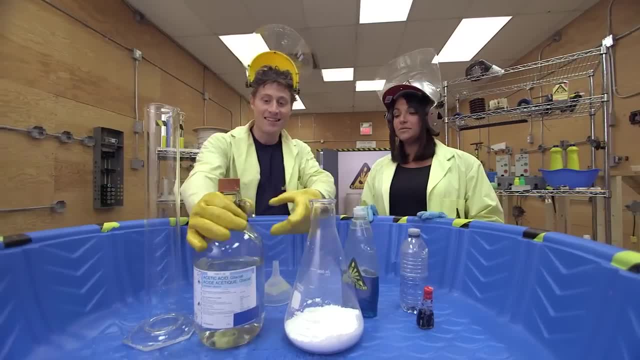 So if you want to have a glass named after you, be a good chemist and design a glass. I want to make a fill beaker. So this is 100% acetic acid. Yep, And what's the difference between this and vinegar? 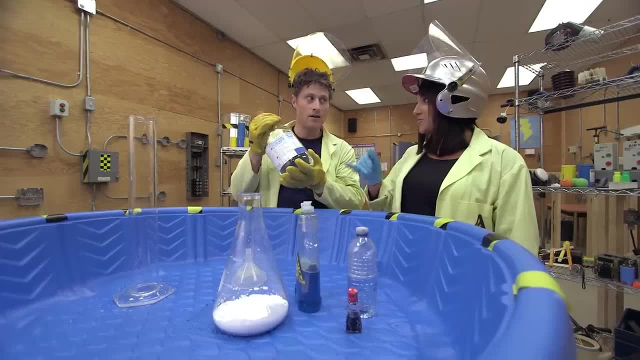 Vinegar has 5% of this and 95% water, but this is 100%, so it's much stronger, Much stronger. Can you put this on your french fries? No, I wouldn't be putting it on your french fries. 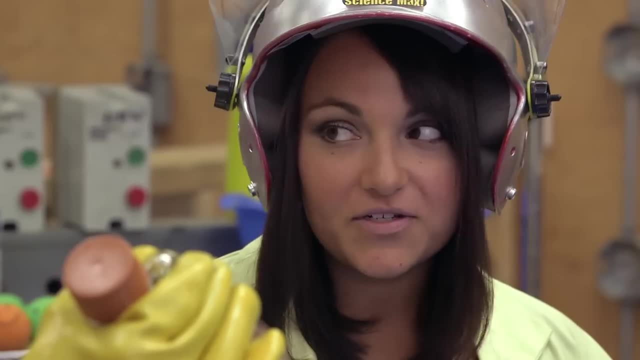 No, How dangerous is this? It's not too dangerous, but you definitely don't want to be breathing it in and you don't want to be eating it Or getting it on your skin. That's why I'm wearing these fancy pants and gloves. 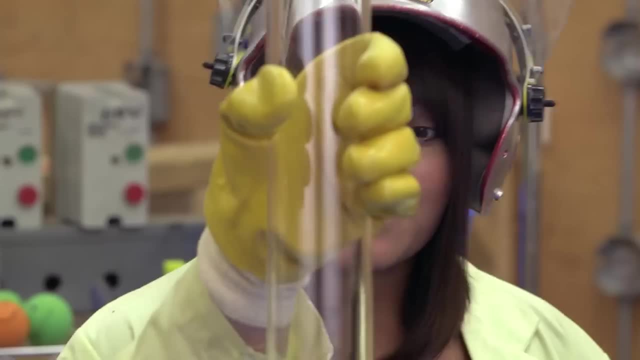 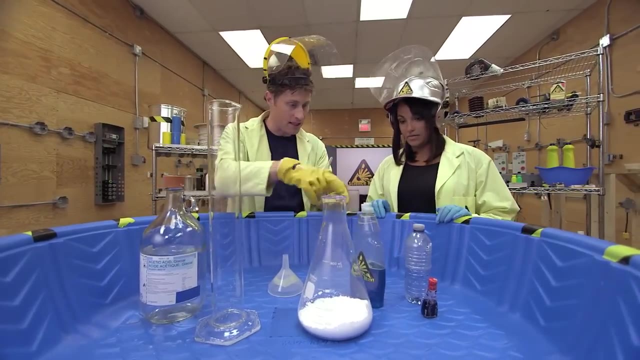 So what I'm going to do is I'm going to pour the acetic acid in this. What's this called? That is a graduated cylinder, Because it finished school, So it graduated. Now you're going to mix water and food coloring and soap all together. 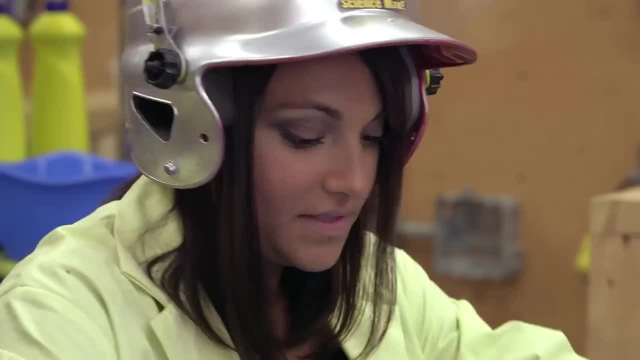 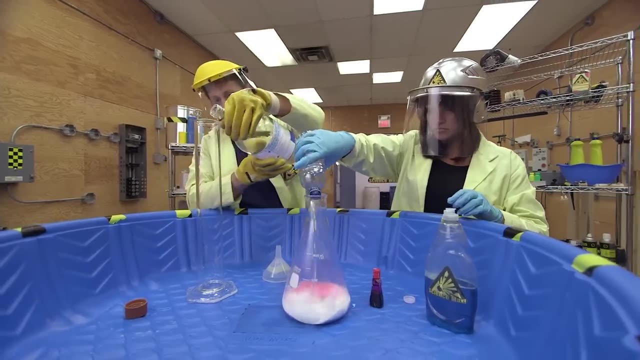 Yep And pour it into there. It'll help dissolve some of the baking soda, so hopefully it'll react better with the acid. Sounds good. Face protection: Oh, All right, That's good. And now when we do it? 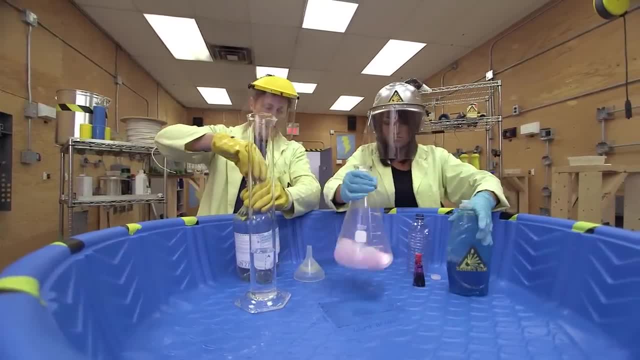 I want to add the funnel at the end to like accentuate the concentration, But I don't know if it's going to go so fast that I won't be able to get it in there. but we'll try it, Try it. 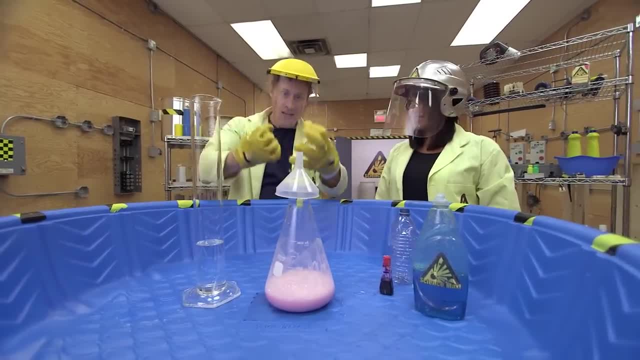 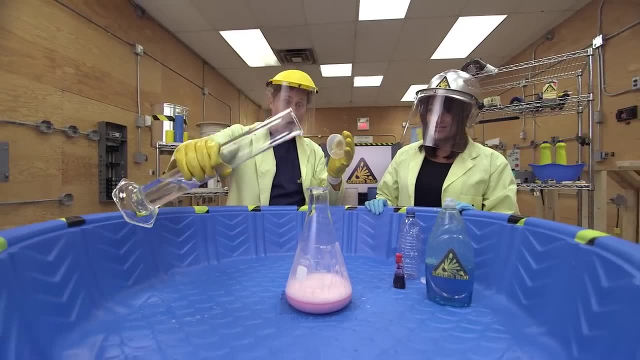 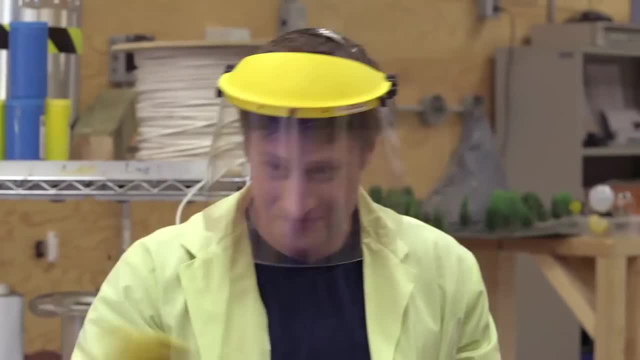 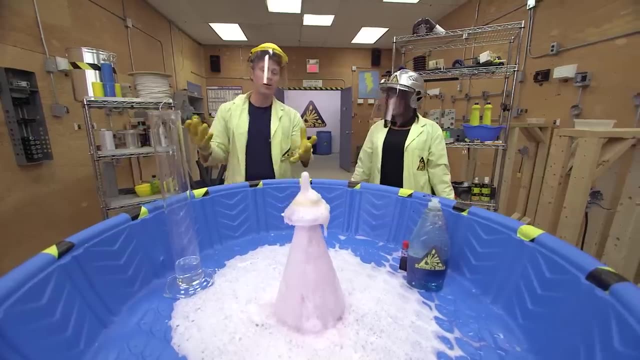 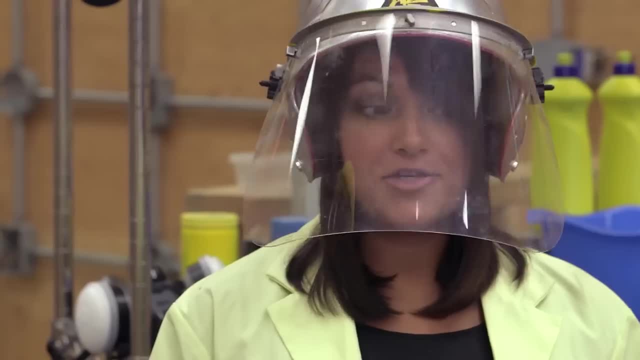 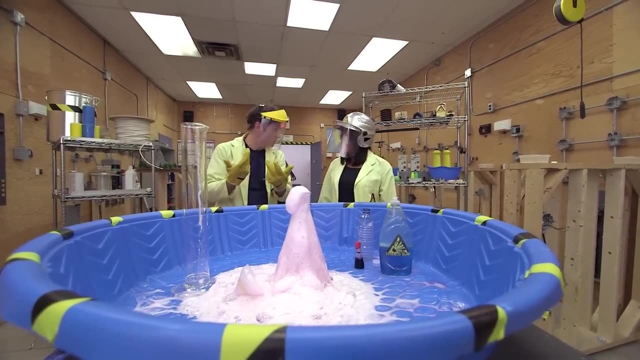 using a different chemical reaction. Ooh okay, Like what The decomposition of hydrogen peroxide produces: oxygen gas, and so that one's pretty vigorous if you use a catalyst. So we want something that makes a lot of gas, so that it makes. 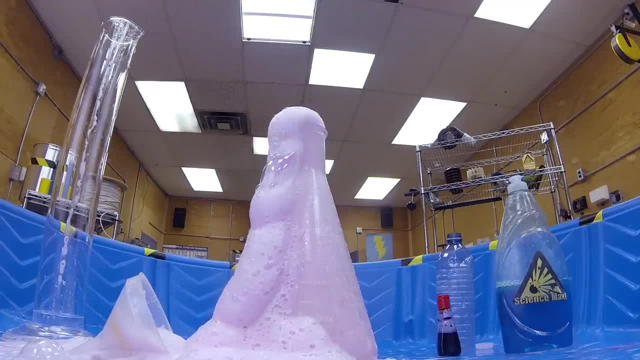 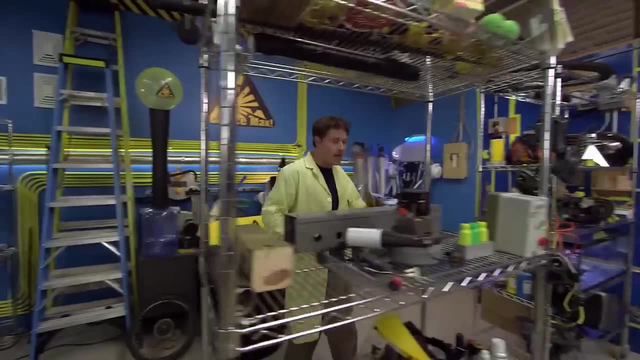 a lot of bubbles when you put the soap in it. Yep, Great, Let's do it. Let's do it. Today we're combining two different chemicals to create a reaction. Sometimes, chemicals can combine in a way that makes them very different from how they started out. 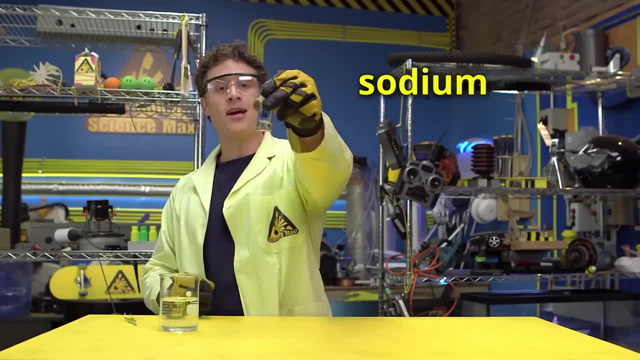 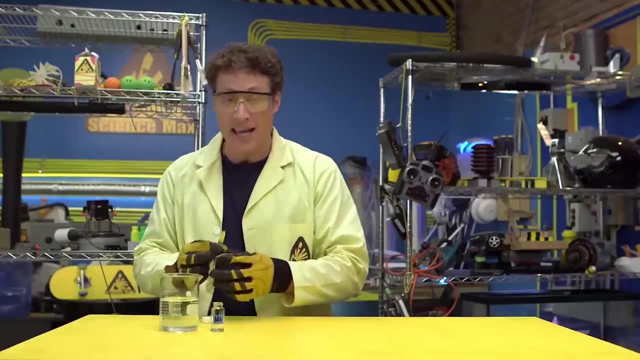 For example, this is sodium or Na on the periodic table Now the sodium tablets are in mineral oil because sodium reacts very strongly with water, even the water in the air, or especially the water in my skin. Watch what happens when I drop. 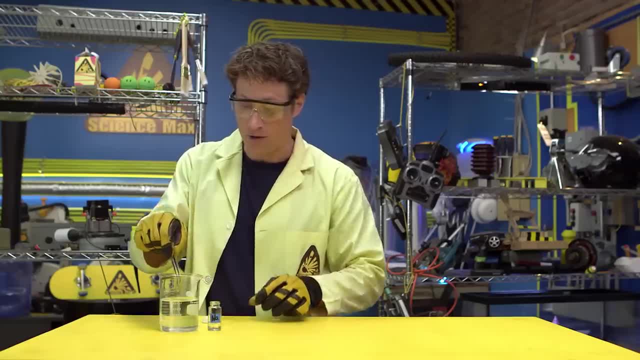 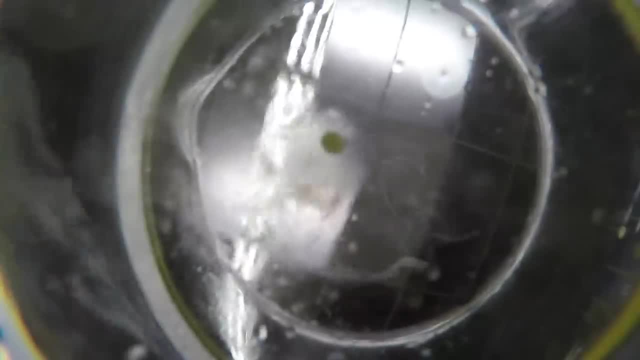 a sodium tablet into this beaker of water. Very cool And very dangerous. And this is chlorine or Cl on the periodic table. Chlorine gas is very poisonous, So So what happens if we combine these two chemicals in a way? 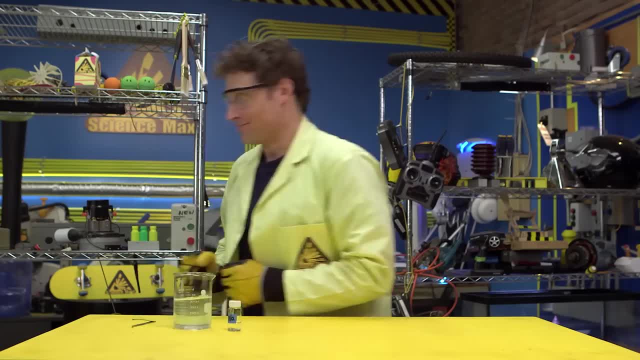 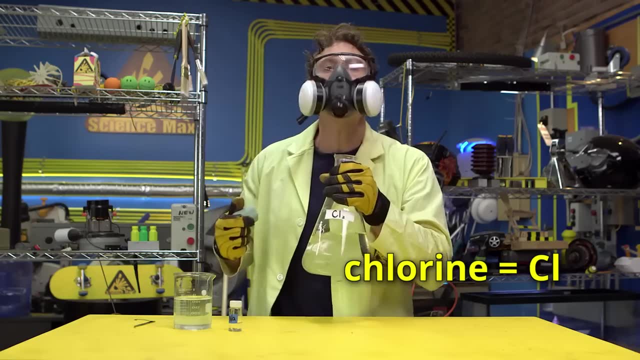 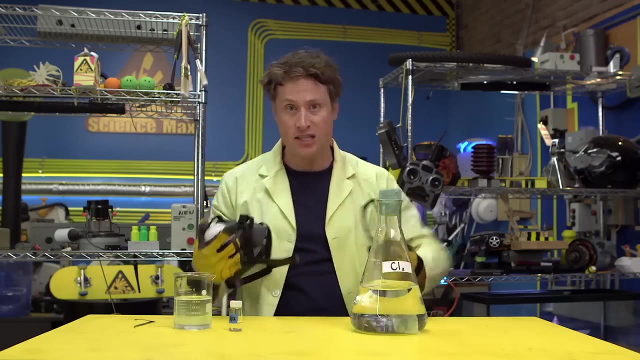 that makes a lot of difference. Well, the first thing we're going to do is take the chlorine and the Na. Now we're going to take the chlorine and the Na. Now we're going to take the chlorine and the Na. 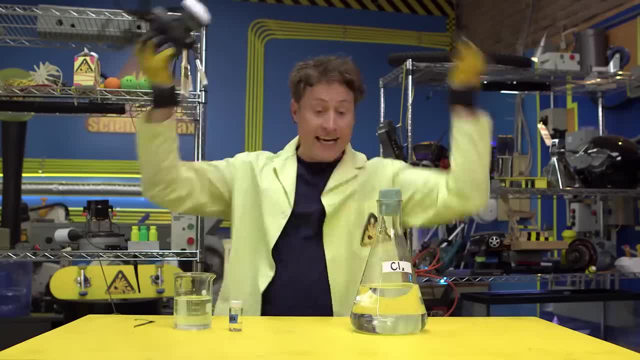 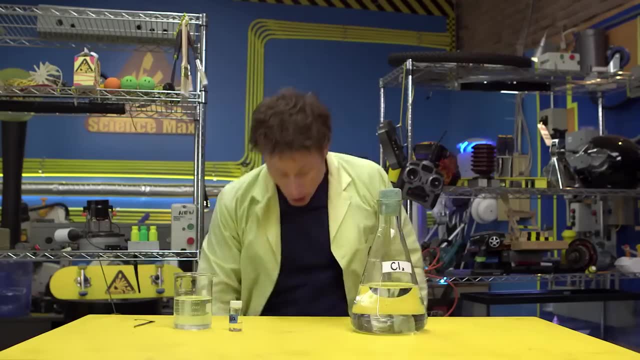 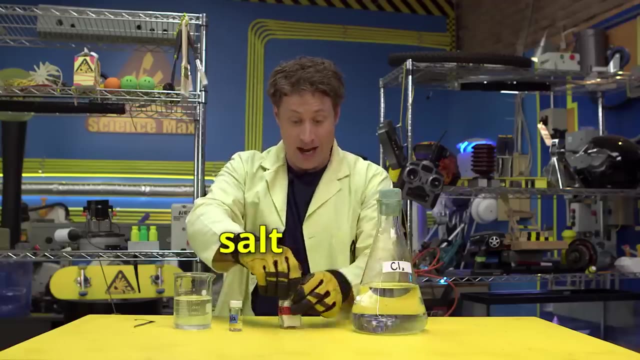 Now, what happens if we combine these two deadly substances? Do we create some sort of super poison, Something more deadly than anything else known to science that causes fear and chaos in chemistry labs all over the land? No, We create salt Good old. 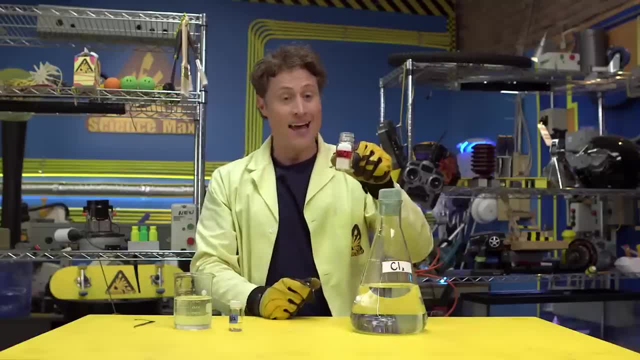 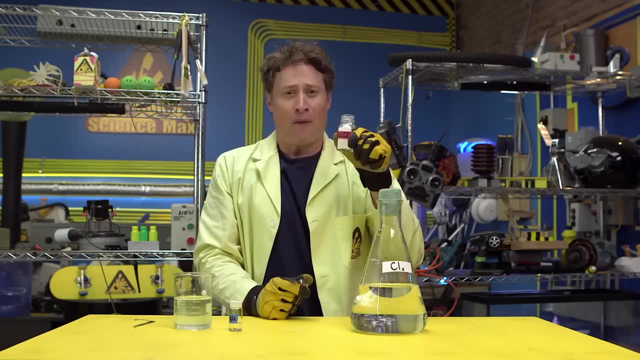 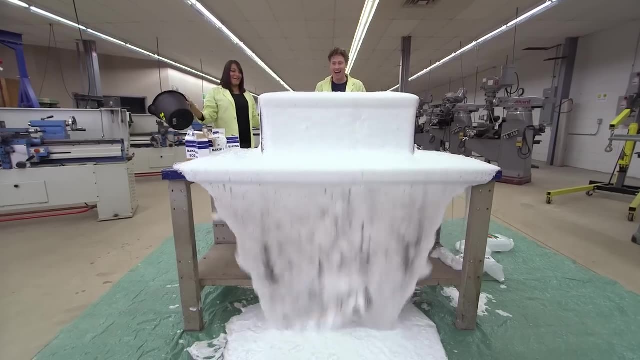 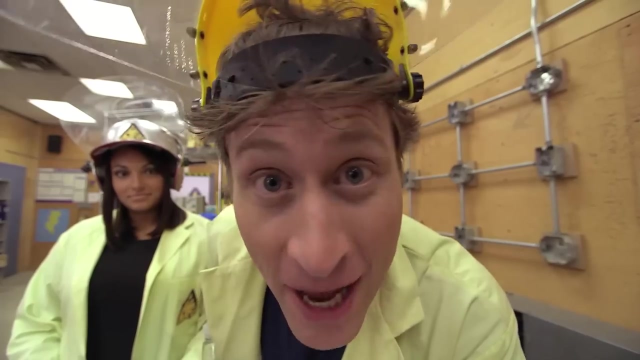 normal table salt. These two substances combine to make NaCl salt Great. We've gone from vinegar and baking soda to 100% acetic acid in baking soda and now we're doing the vinegar and baking soda volcano version three No longer. 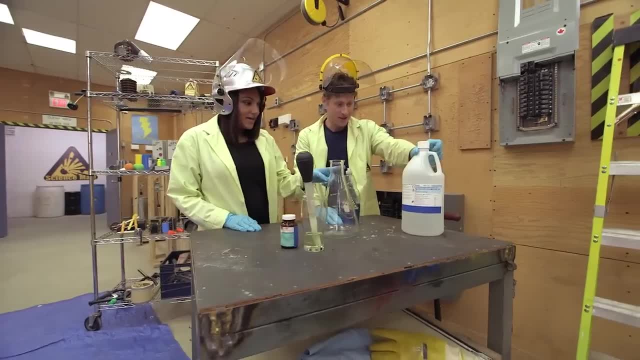 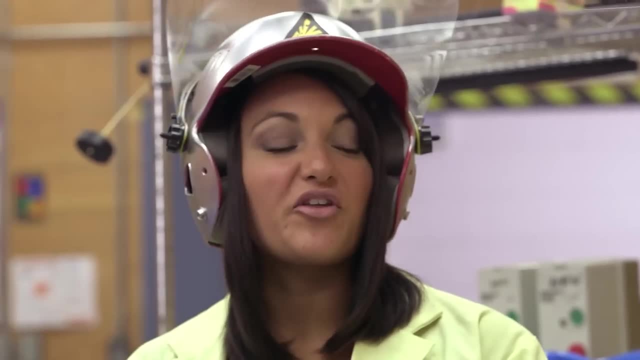 vinegar and baking soda. Nope, What are we using this time? So here we have some hydrogen peroxide. Oh, that's good, Yeah, but the stuff at home is only 3%. This one's 30. So much, much stronger. 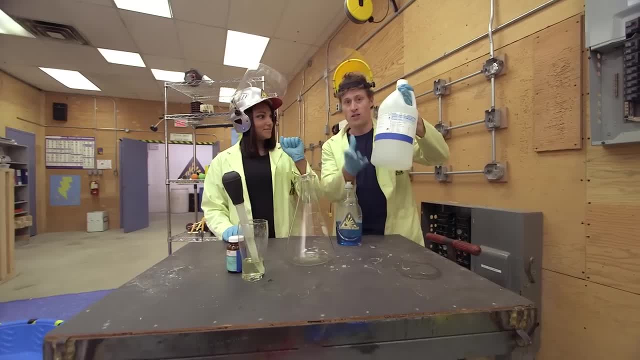 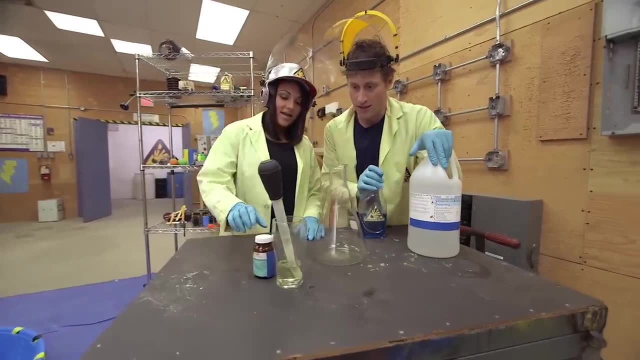 Ten times stronger? Yes, And is this more dangerous? It's definitely corrosive, so wear your gloves. Corrosive means it could eat your skin. It can burn your skin a little bit, Which is why we're wearing gloves and blast shields. 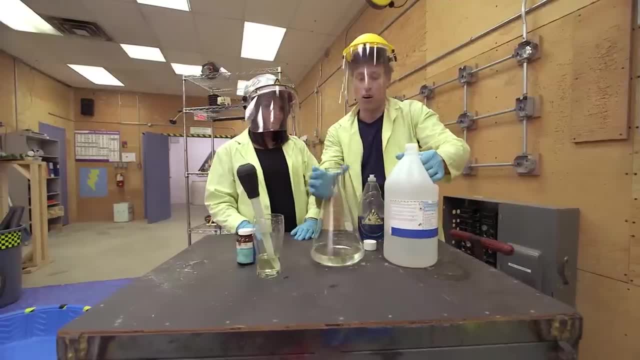 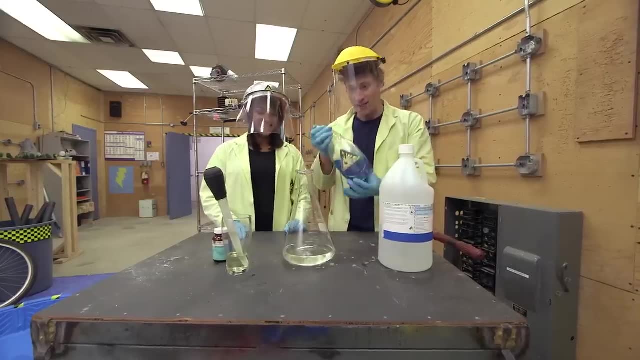 What's going to mix with this? So here we have some potassium iodide, which is a salt, and it's mixed in with some water. The most important part of this reaction is when you put in dish soap, right, Yep, So one big squirt. 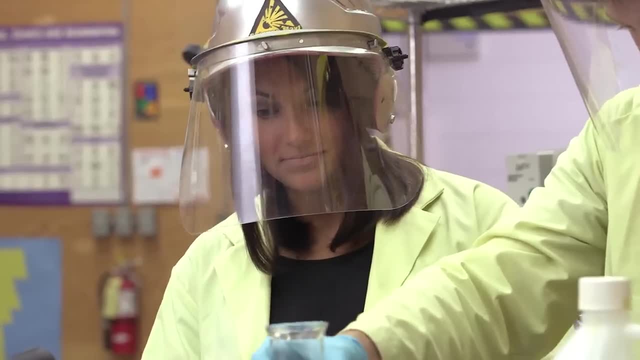 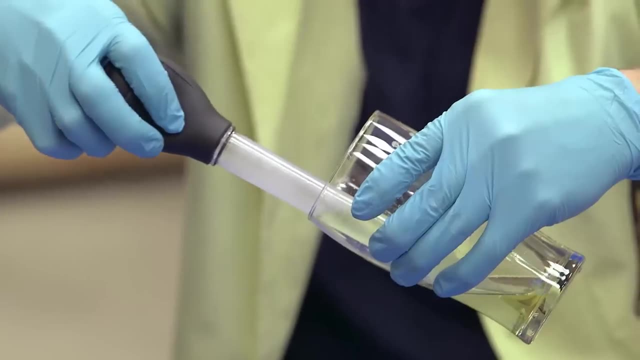 of dish soap like that, Mix it up. Now we go over to the blast zone. That's plugged in. All right. Now that's a reaction. It looks like there's steam coming on here. Oh yeah, Oh yeah. 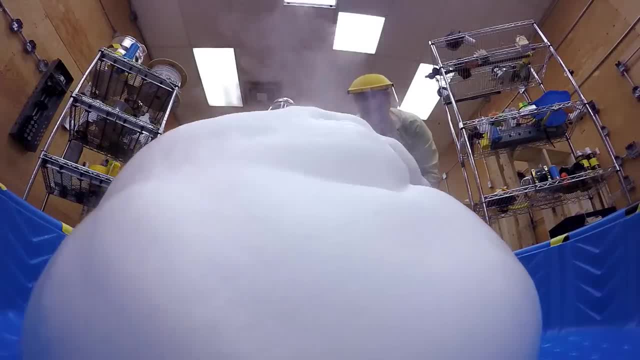 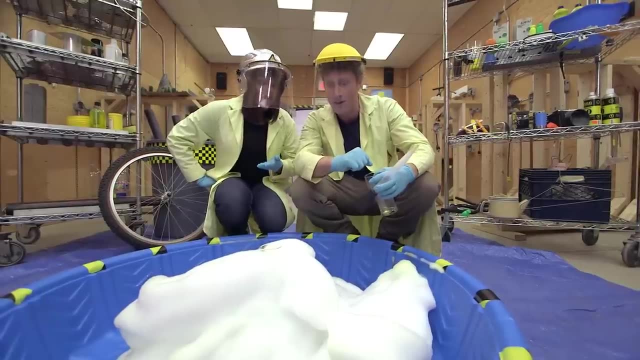 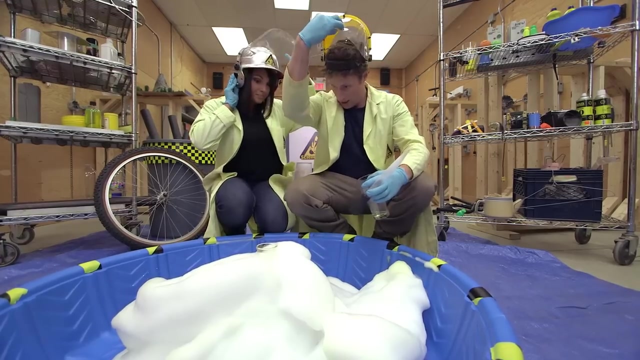 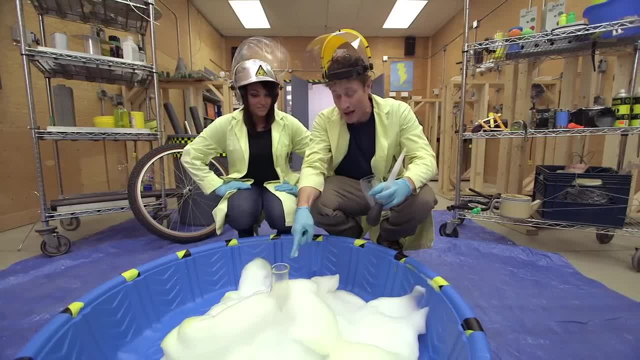 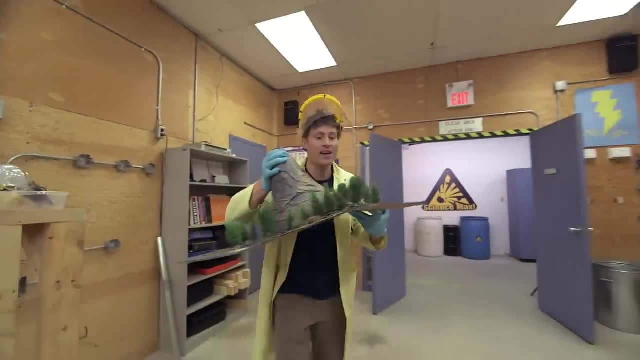 to turn this off, So it's gonna be really hot, Right? So we're going to do the same thing, but we're going to do a new reaction, So we're going to do this reaction here. So it's Sounds like a good idea. 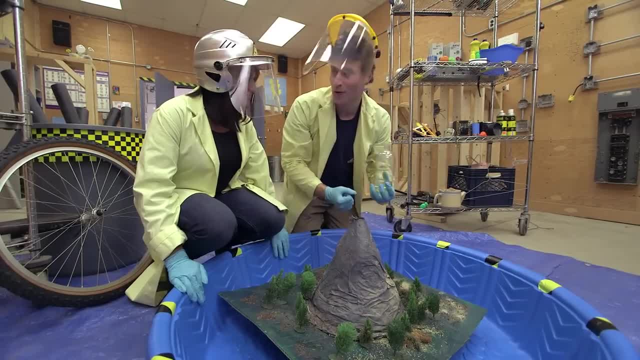 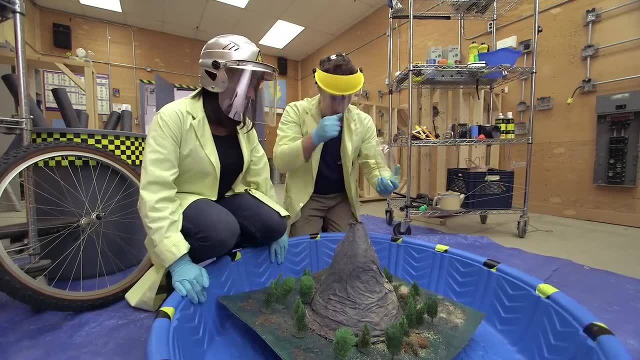 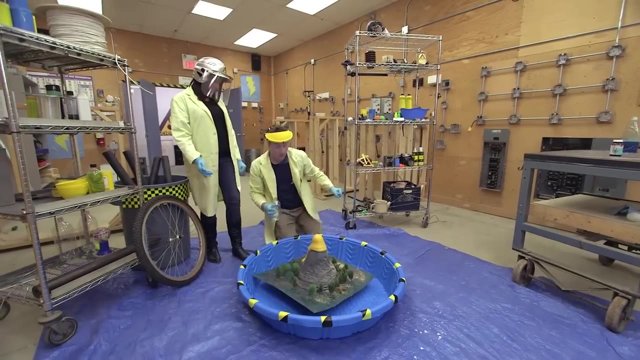 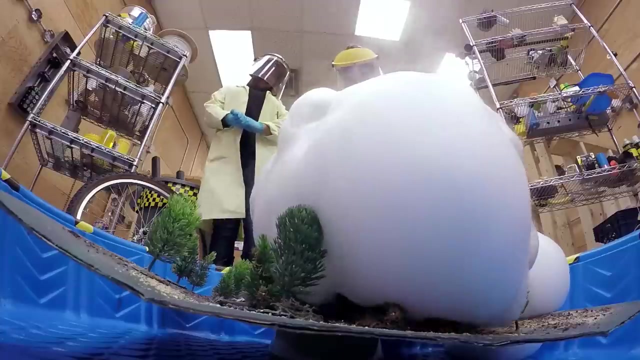 Okay, so if we put it over here, All right. Volcano version 3.5.. Hydrogen peroxide, potassium iodide- Right here we go. Oh, Looks like lava. Whoa, Look at that. That. now that is a big volcano eruption. 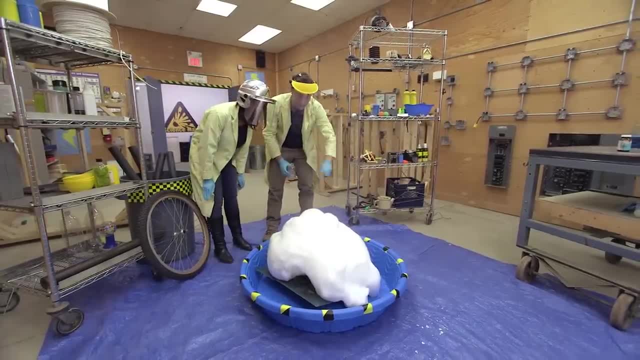 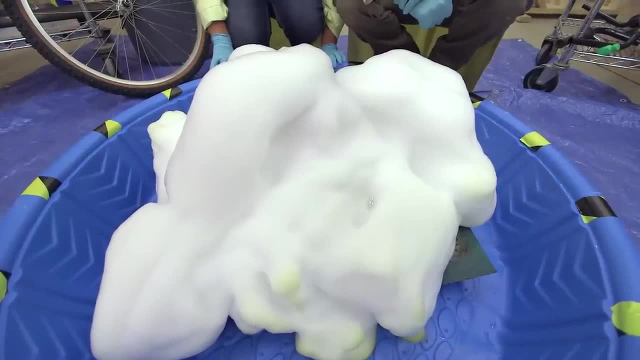 Just covered the town. That is completely Yes. that town is gonna be very clean because it's all soap bubbles. It's the cleanest volcano this side of Science, Maxaville. So I still think we can do this bigger, though, right. 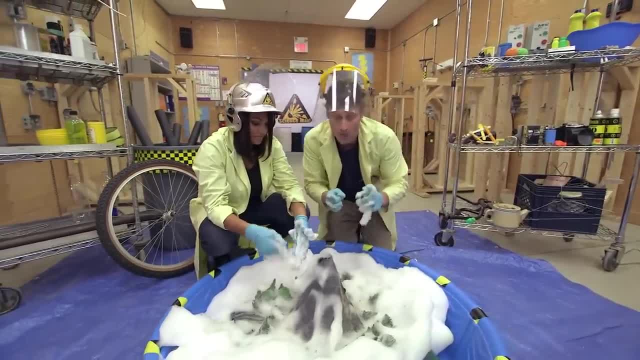 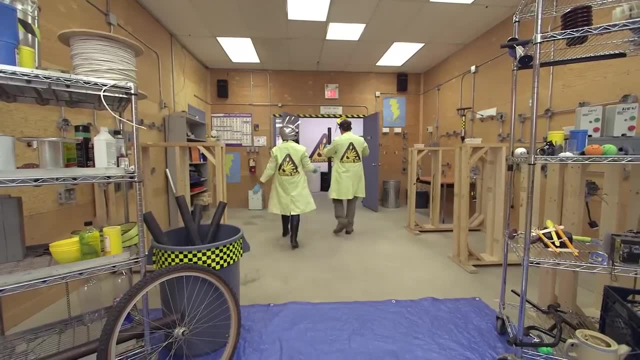 I agree. Um ooh. I know What, if we use some sort of a tube, like maybe one of these right, And then we attach it to like an air compressor, I think you'd get some height. Yeah, and we could get some height. 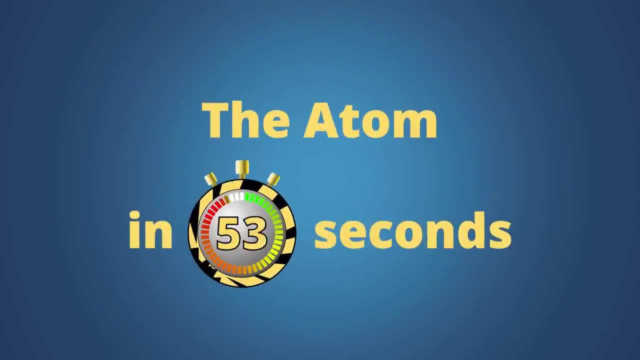 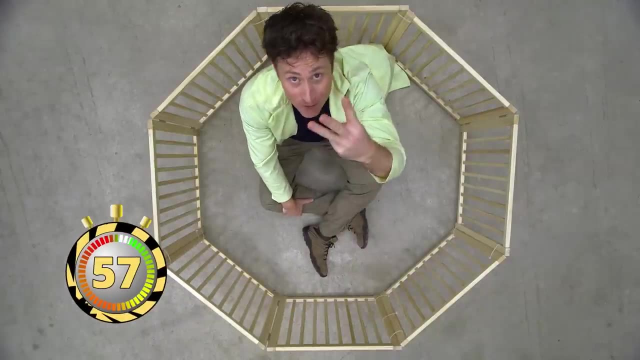 Let's see if we can go aside The atom in 60 seconds. The atom is the smallest unit in a chemical element. Atoms are made of three parts. Part number one are these guys, protons. They have a positive charge. 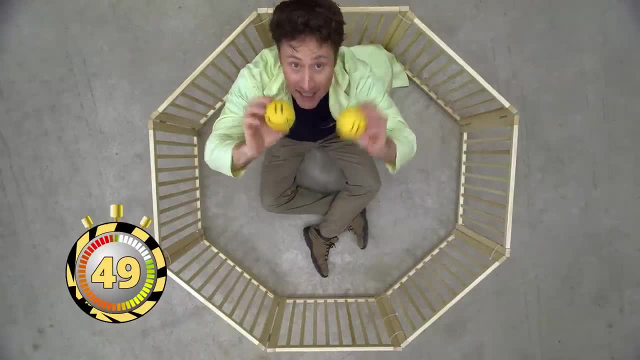 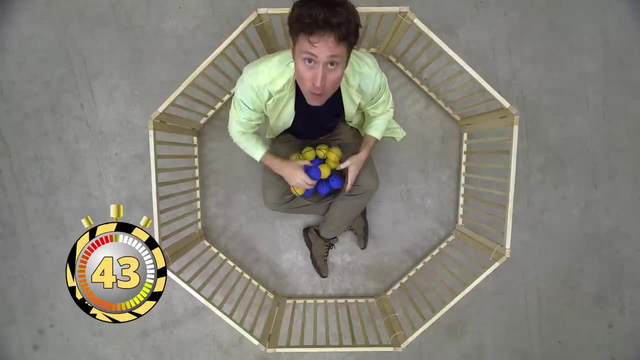 The number of protons determines the element. One is hydrogen, two is helium, three is lithium, and so on. The protons sit in the middle here, which is called the nucleus. They sit in here with part number two. these guys. 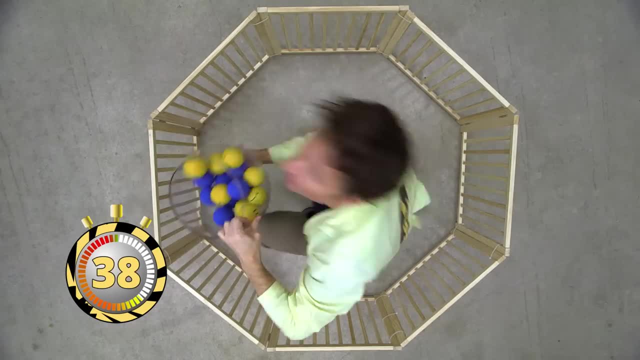 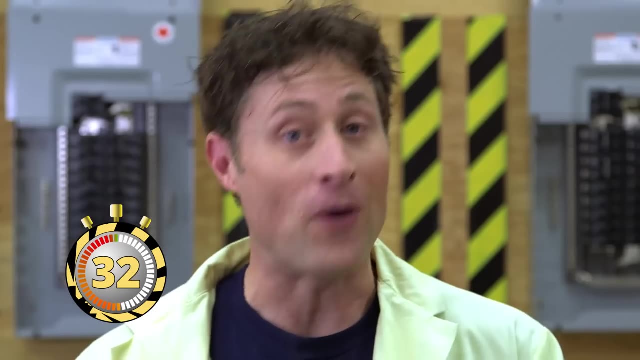 They're neutrons and they have a neutron. They have a neutral charge. Now I've got eight protons and eight neutrons in this nucleus, making this an atom of oxygen. Orbiting around the nucleus are these tiny guys? They're electrons and they have a negative charge. 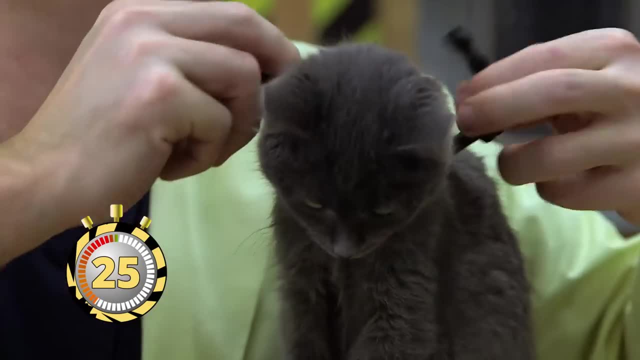 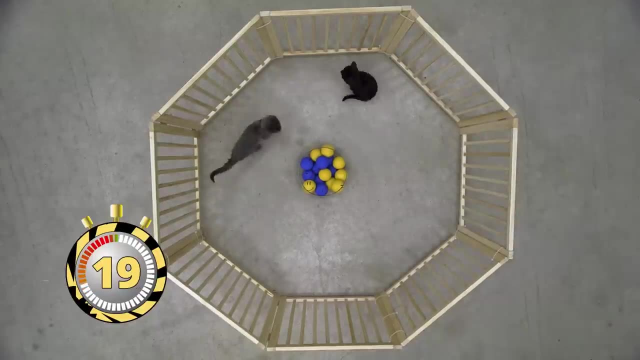 I will demonstrate using kittens. Kittens are perfect because, just like electrons, kittens are really small And just like electrons, kittens move around randomly. You never know where they're going to be. An oxygen atom should have eight kittens or electrons somewhere inside. 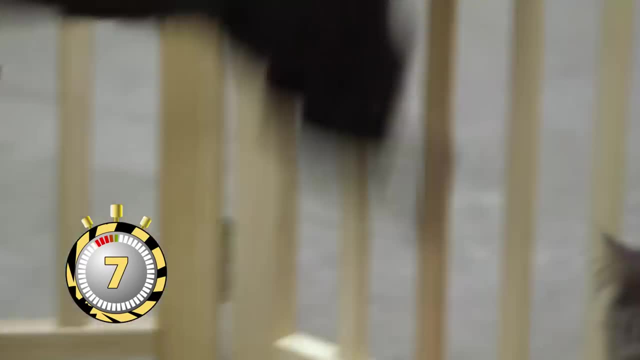 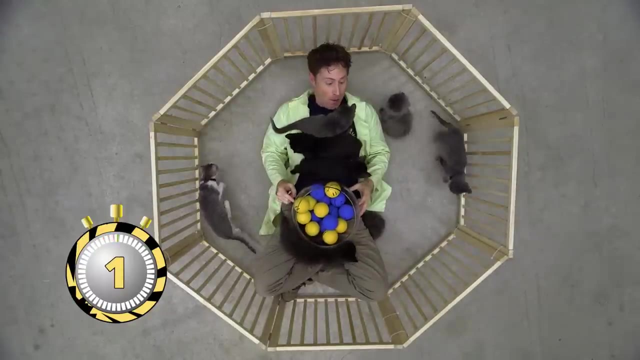 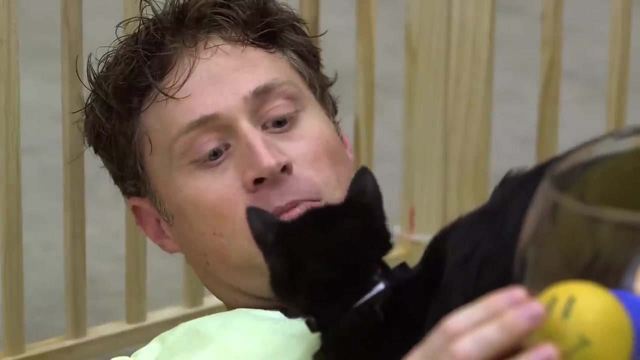 These kittens are constantly escaping, But guess what That happens with electrons too. There you go The atom: a nucleus of protons and neutrons surrounded by randomly moving electrons. Cutest science ever. How do you guys feel? Did you learn something? 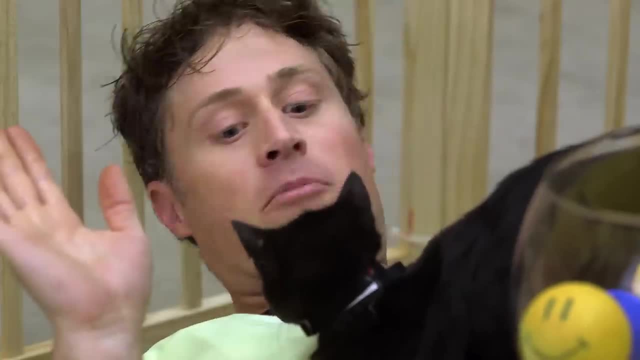 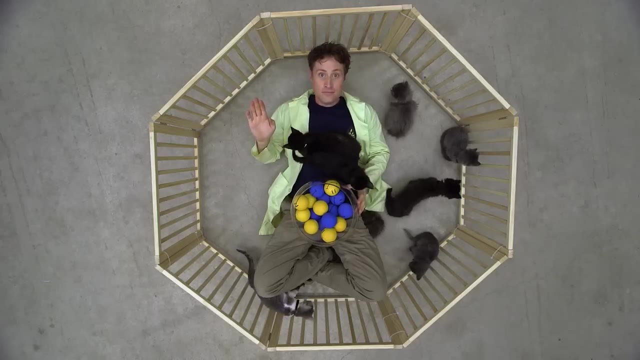 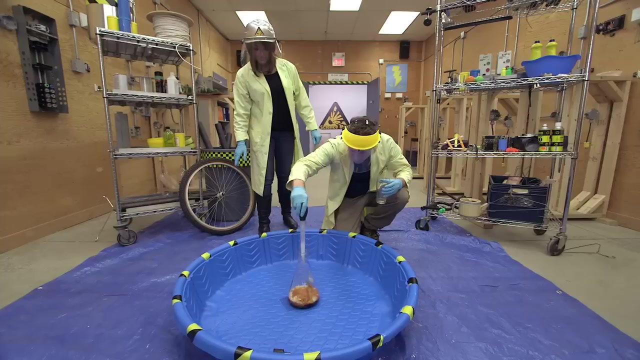 Huh, Pause up. Who learned something? Hm, Do you know what? Solve the question, please. Tellina and I have made a bunch of chemical reactions, But in our quest to max things out, we've got a new plan. 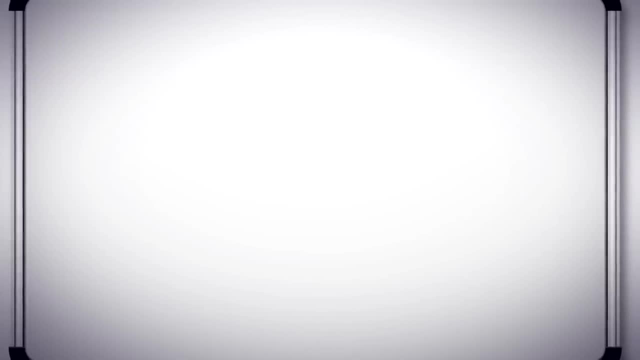 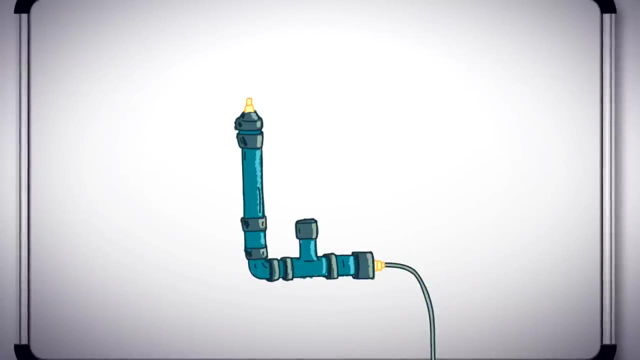 Woah, Hydrogen peroxide and potassium iodide create gas. One way to max out the reaction is to contain the gas in something like a tube. We're gonna put the hydrogen peroxide in the tube first, Then we're gonna put in. 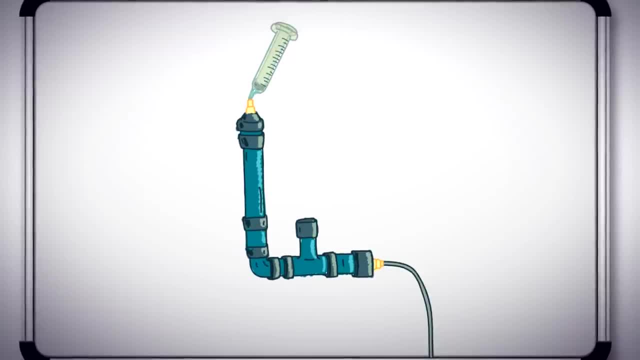 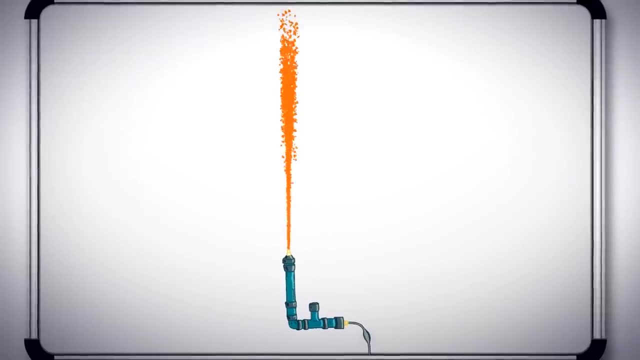 the potassium iodide in the top through a one-way valve. Then we're going to pressurize the container. When it finally reacts, it will shoot up through the valve and we'll see how high we can get our stream of bubbles to go. 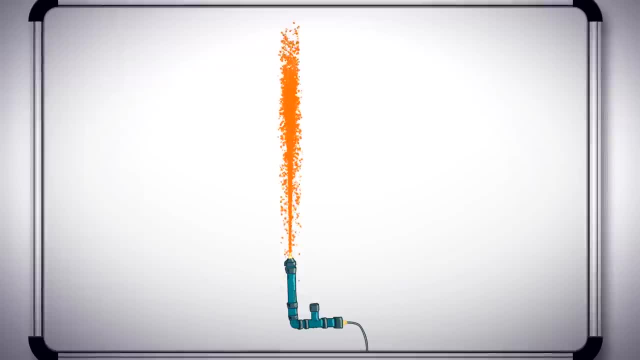 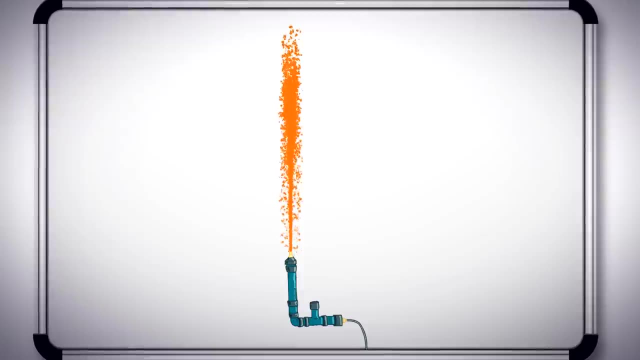 But be warned: capping anything and not letting it escape is never a good idea. So we've got a release valve to make sure things work out. This is one of those experiments that's definitely on the list of don't try this at home. 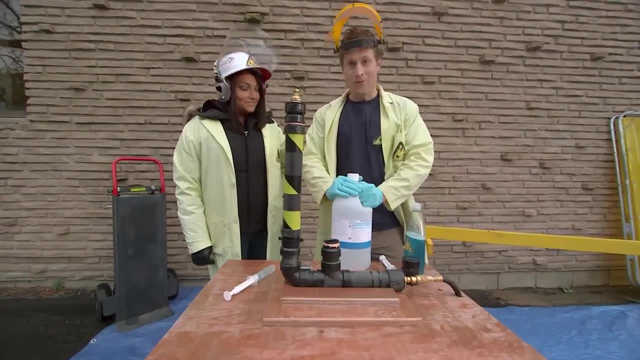 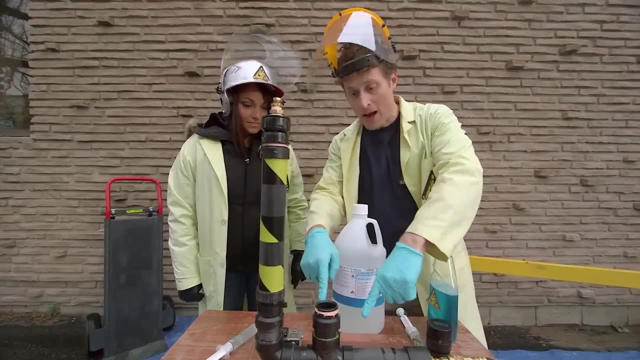 Vinegar baking soda, volcano version four, hydrogen peroxide, potassium iodide, And what we're going to do this time is we're going to put it in this tube. Hydrogen peroxide goes in here And we've got. Talena, do you have the potassium? 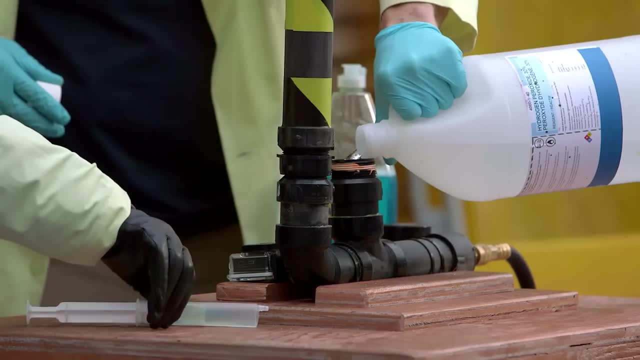 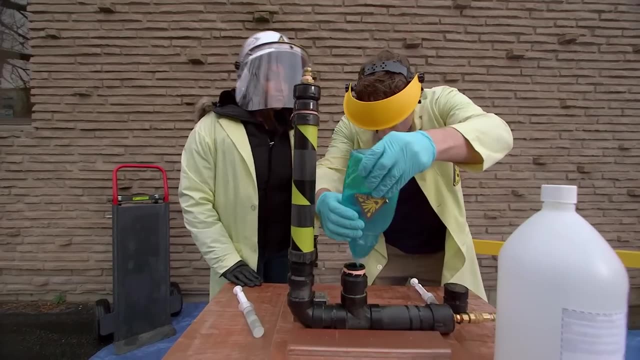 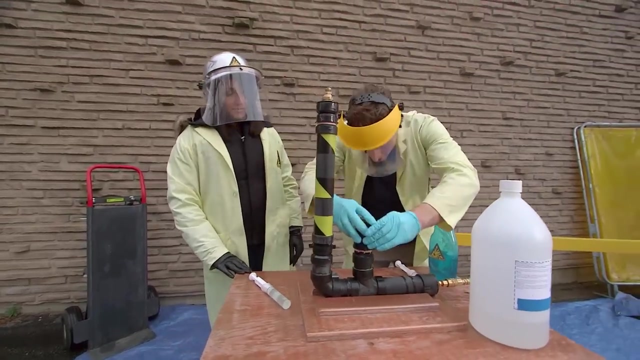 iodide in syringes- Yeah, two syringes full. Two syringes full About. there is good And then soap, Good amount of soap in there, And so what we're going to do is we're going to close this off. 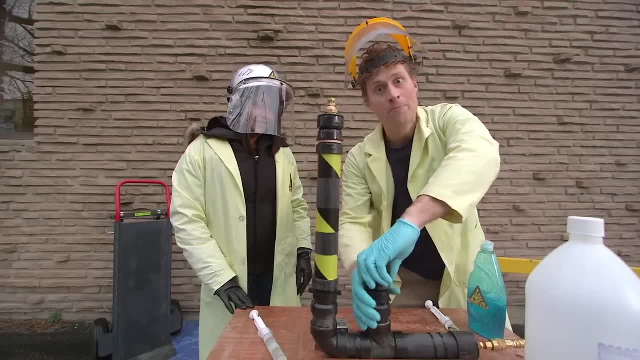 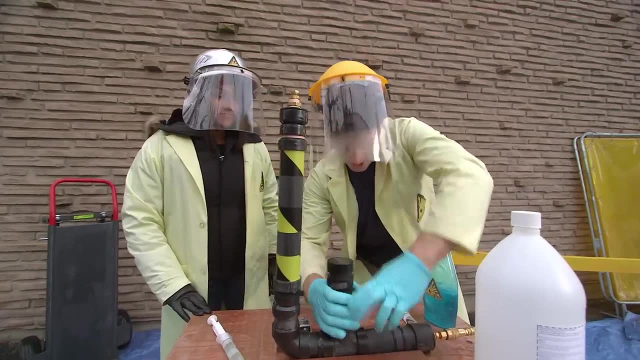 and tighten it up, And then we're going to pressurize the whole system, And then we're going to add the potassium iodide And it's going to be spectacular, we hope. OK, that's on tight, This is all good. 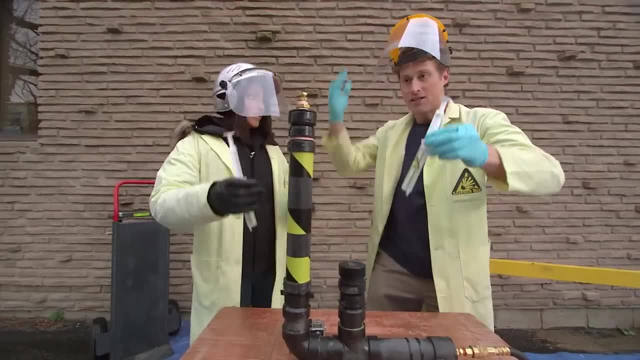 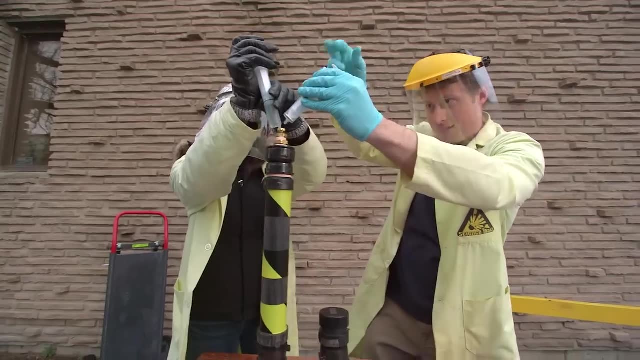 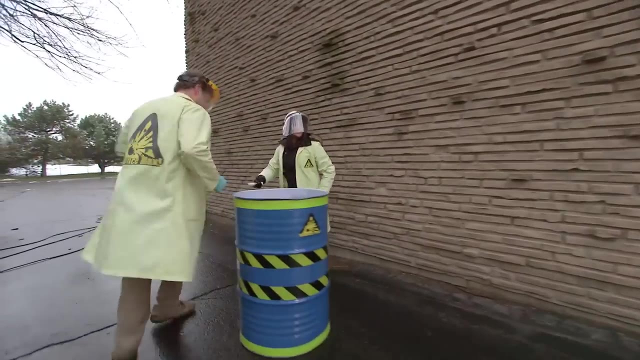 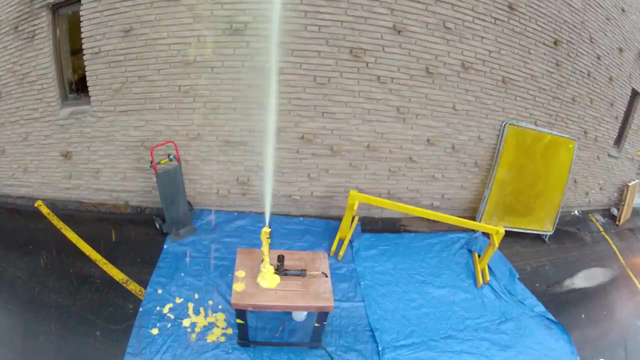 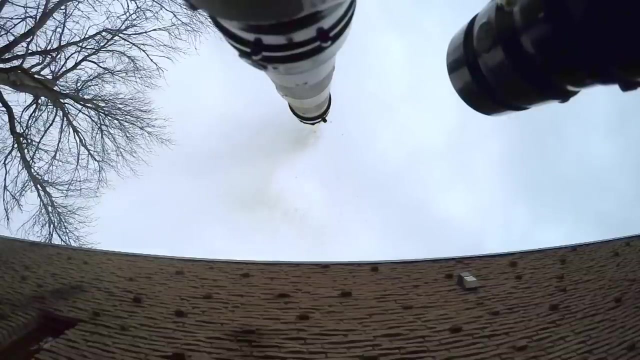 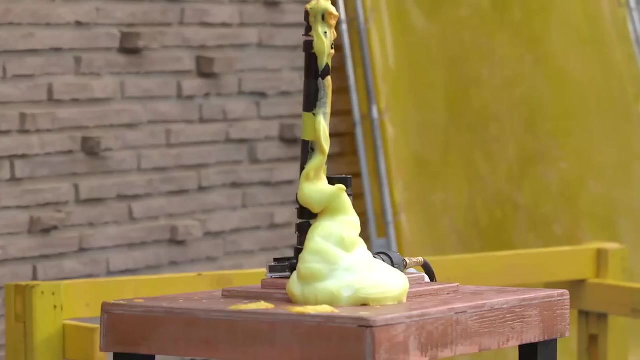 Putting this down here And potassium iodide goes in here, puts down Ready One, two, three go And we back away slowly. Whoa, Whoa. Yeah, that's what I'm talking about. OK, let's check it out. 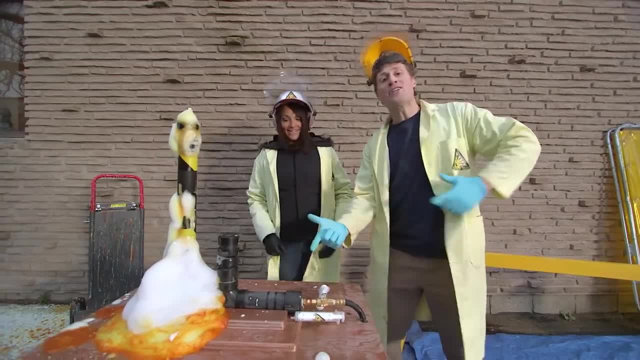 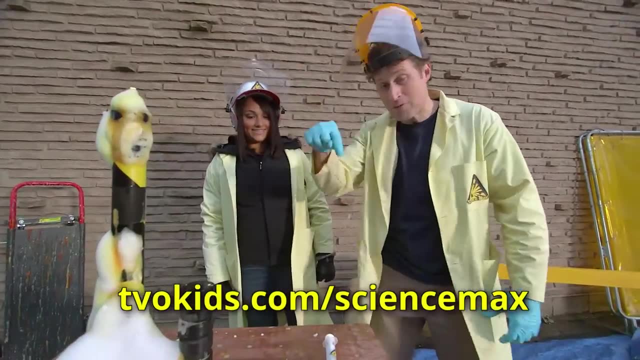 Whoo. All right, there you go. Vinegar and baking soda: volcano maxed out. Thank you, Talena, That was great. If you guys want any instructions for the stuff that we've done today, they're all on the website. 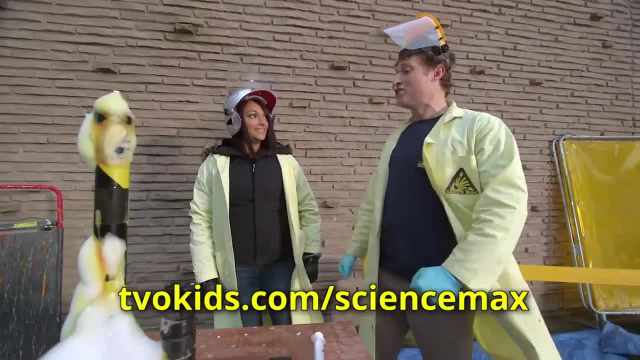 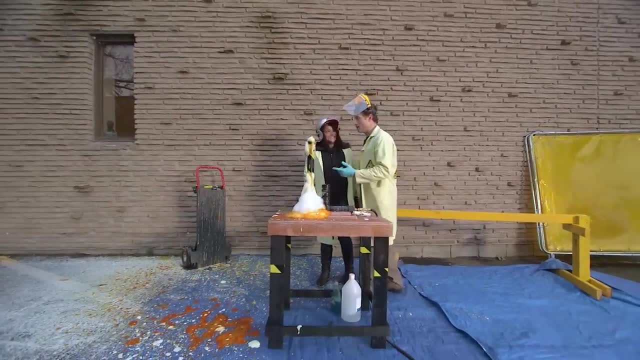 And thank you very much for watching Science Max Experiments at Large. We kind of need to clean up a lot, don't we? We have out here, we have the other room, So tell you what you get: a mop, I will get the hose, and a wheelbarrow for the sun. 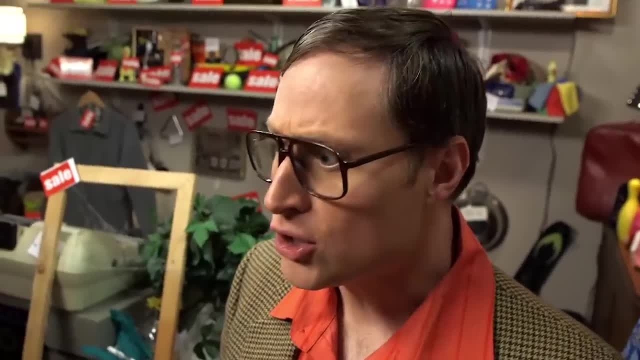 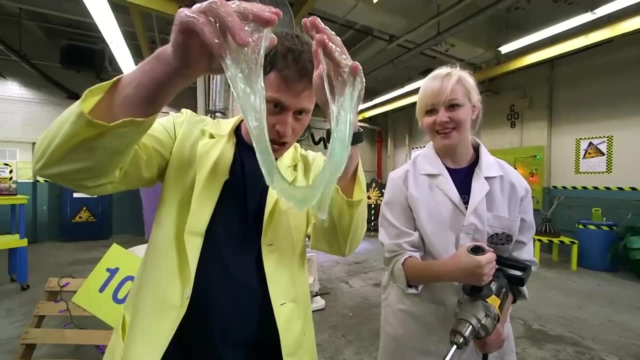 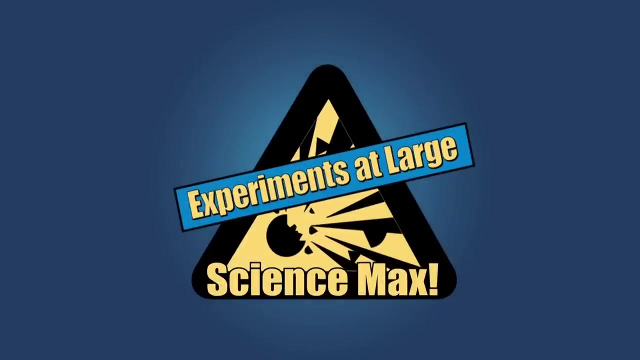 Today we're looking at polymers, Polymers, Polymers, Polymers- Word has lost all meaning: Plastics, latex, rubber and our favorite polymer slime. Oh yeah, All on this episode of Science: Max Experiments at Large. 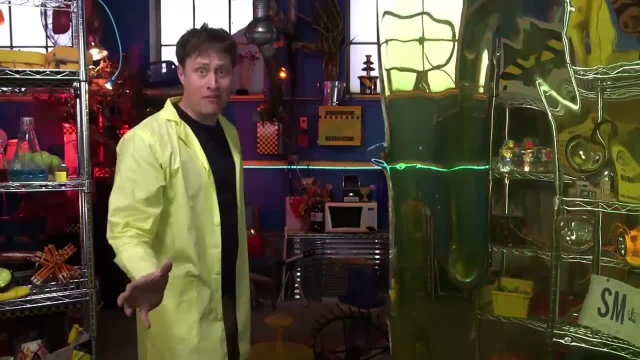 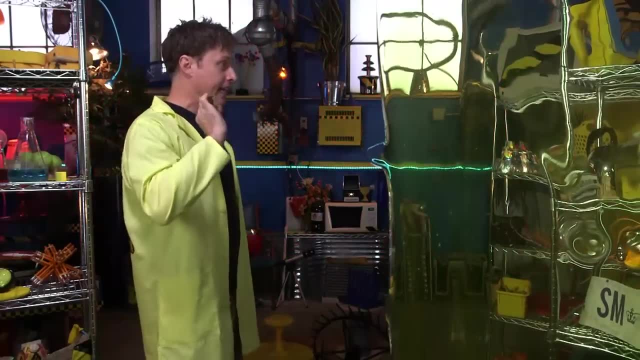 Oh, greetings, Science Maximites. My name is Phil and I think I might have overdone it with the science. I mean, what's a better use of science than creating a whole bunch of slime? Well, I did, and you know what? 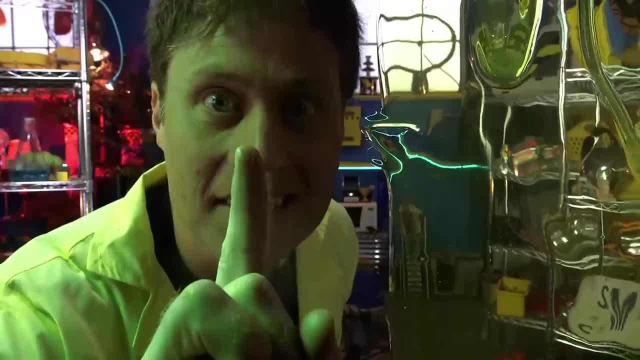 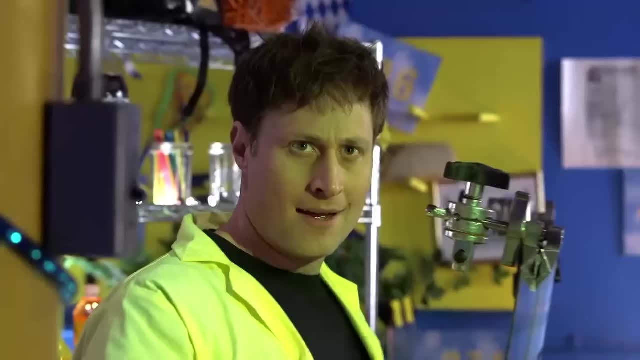 It's really cool. It's really cool, It's really cool. It's slime. I love slime. It always makes me feel like a mad scientist, But I need a good mad scientist. laugh: Mah-ha-ha-ha, Ho-ha-ha. 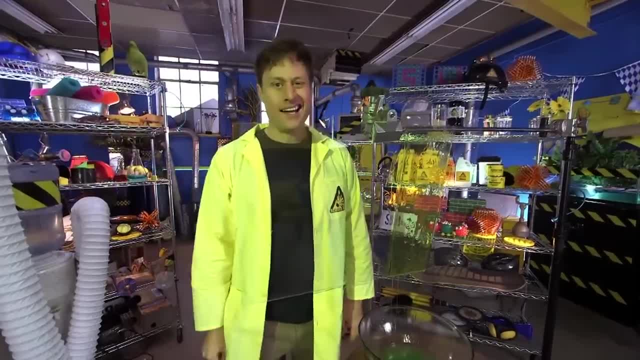 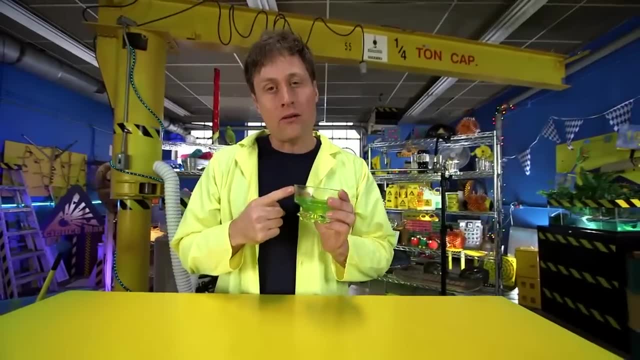 Ho-ha-ha-ha Ha. Yeah, it needs work. Anyway, today we are talking about polymers. Polymers like slime, But you see, polymers aren't really a substance, They're more how something is constructed. 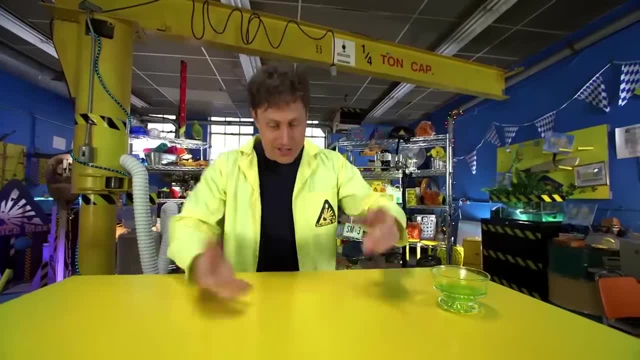 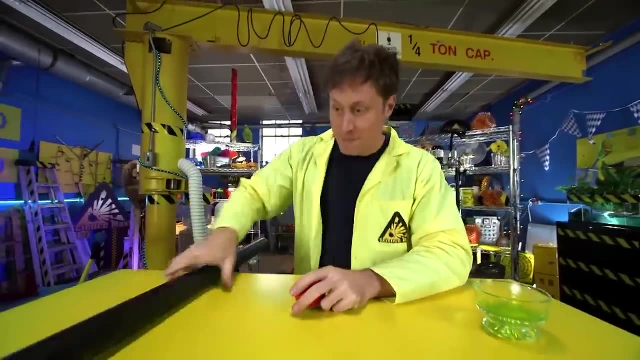 And there's all kinds of different polymers. There's slime, obviously, and rubber polymer like well, like rubber, And there's also hard polymers like plastic. Now, polymers are all kind of constructed the same way. 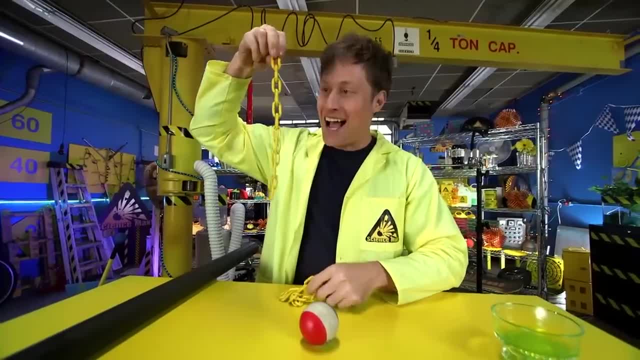 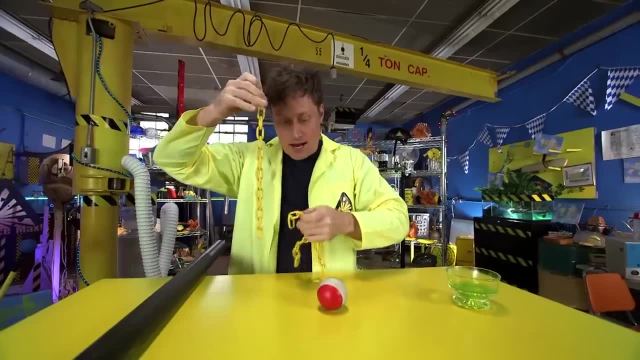 like this: This is a chain. Yeah, so imagine this is a chain of molecules and all the molecules are the same and they just repeat in a long line. Now, when you get a polymer like slime, all the chains are not connected or very loosely connected. 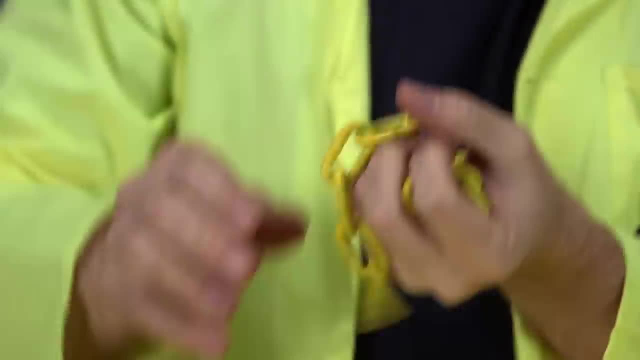 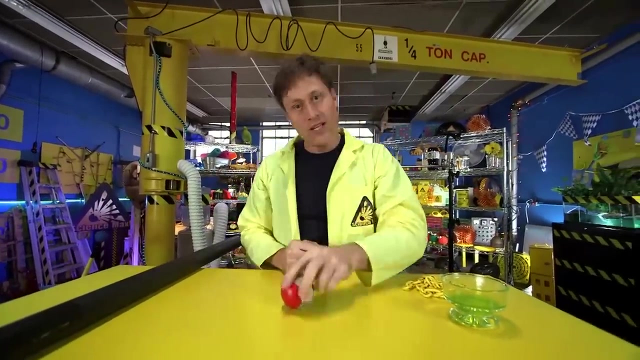 which means that they can flow over each other like a slime or sort of like a liquid and they behave like that. So that is slime. But when you get to a rubber polymer you start to get little bonds in between the chains of polymers that work like this. 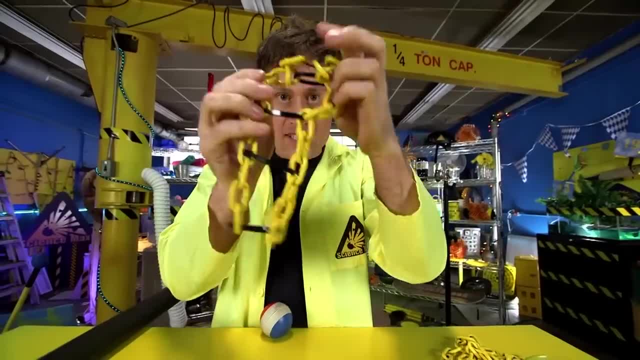 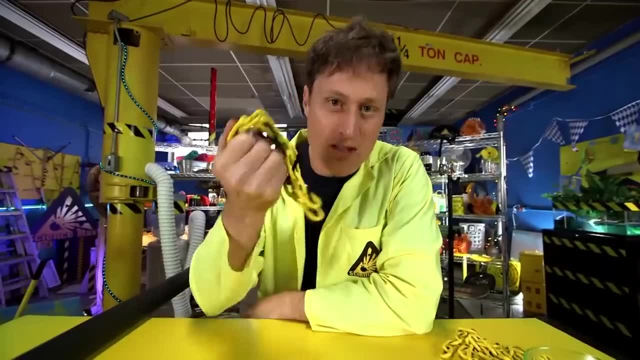 You see, they still move around a little bit, but they can spread apart and they become flexible and bouncy. Yeah, I know, a chain doesn't really bounce, but rubber polymers do. Huh, Now, when it gets to a slime? 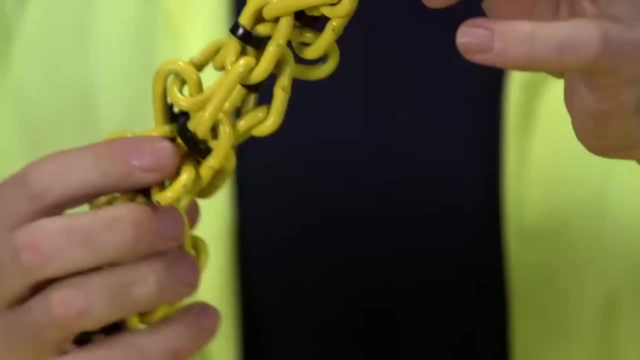 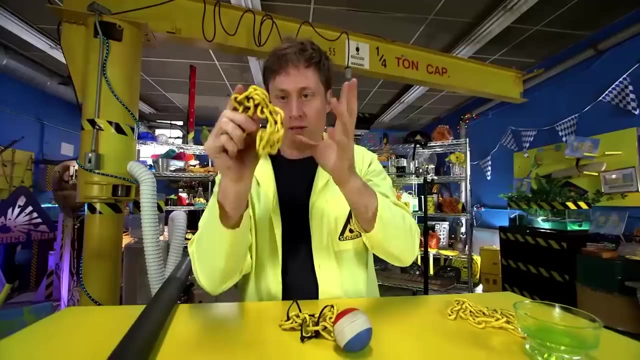 when it gets to a solid polymer like plastic, there's a lot more links and it's all kind of interconnected and it doesn't move at all. It doesn't move- Okay, again, harder to tell with a chain, but plastic is very hard and rigid. 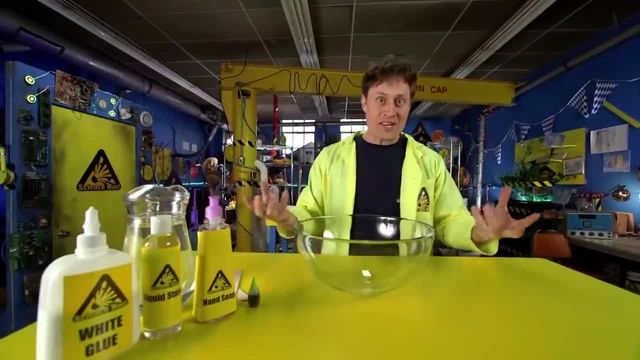 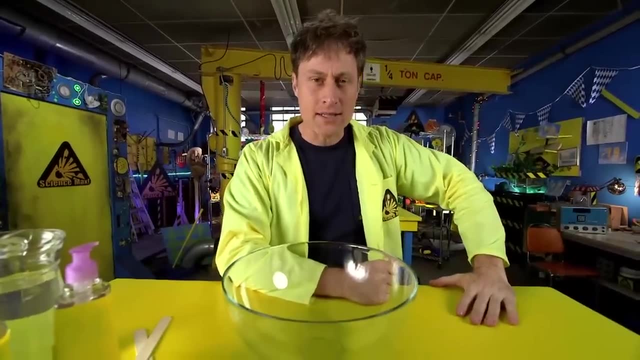 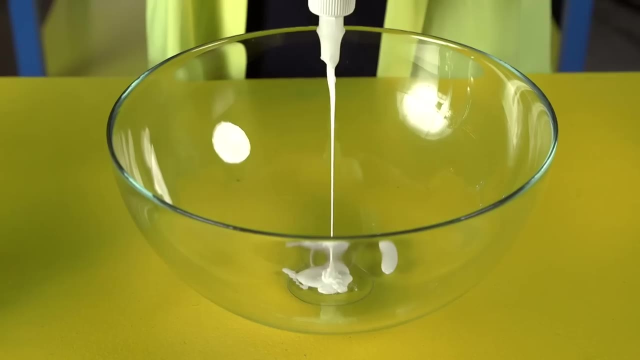 So let's dive into the world of polymers and make some slime. Yeah too mad. not enough scientist. I'll keep working on it. Anyway, to make slime, take your white glue and pour in, uh, an amount. 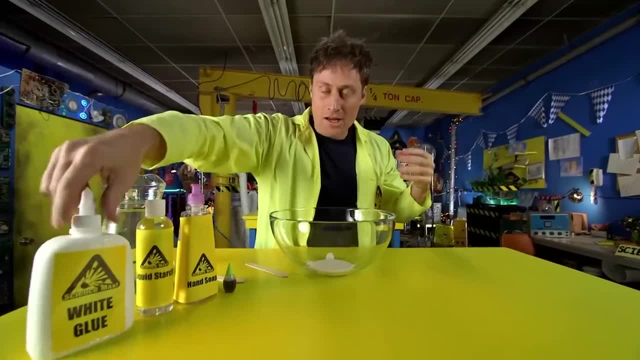 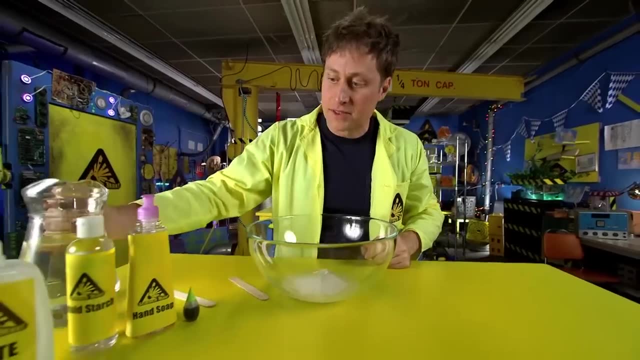 It really kind of depends on how much slime you want to make. Now you want to add about twice as much water as that. Uh, yeah, somewhere around there. great, Now we want to put in just a little bit of soap. 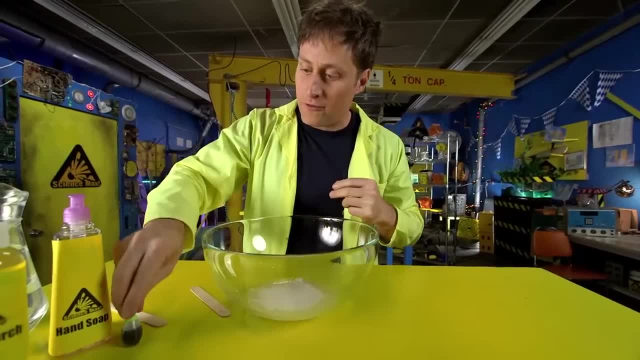 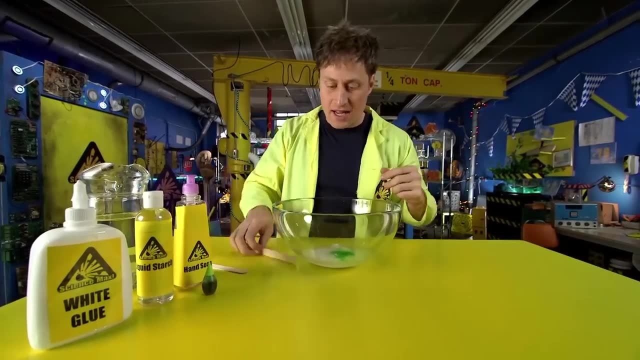 Mm-hmm, maybe there that's good And you want to put in your food coloring. I like green. Green seems like the right slime color to me. It's the right, appropriate mad scientist kind of slime. And then you want to start mixing that up. 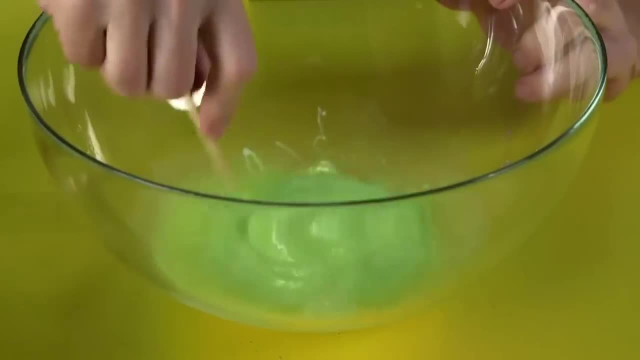 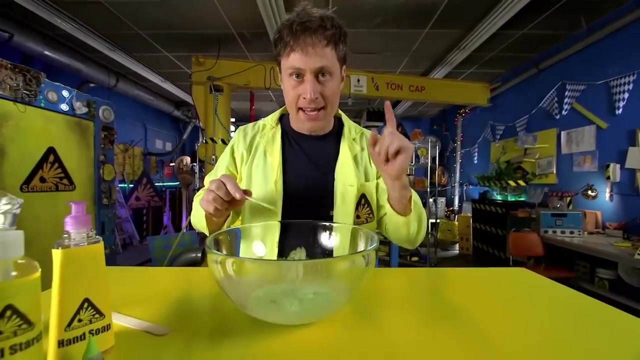 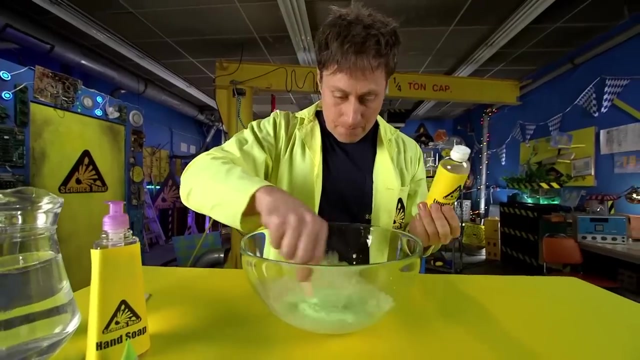 till you get the right kind of consistency. That means make sure the glue and the water are equally mixed up. Good, And now we're ready to make it an actual slime by bonding the polymers together by adding liquid starch Mm-hmm. very good. 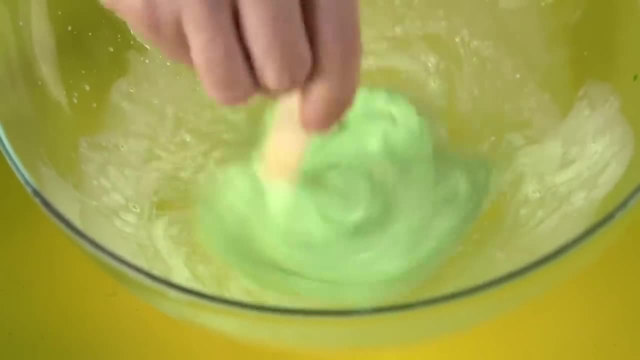 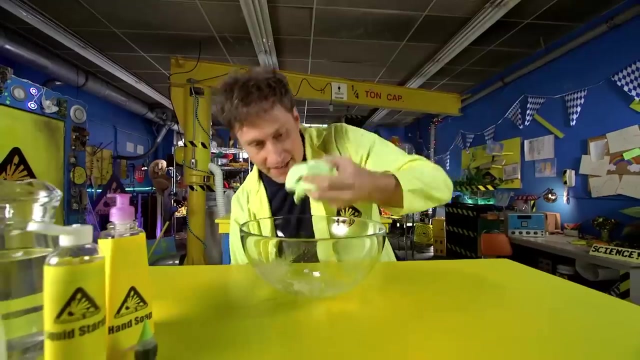 And you want to mix it up. When you add the liquid starch, it starts to bond the chains of molecules together, changing it from a liquid to a slime. It's coming along And there you go- slime. Now, if you want clear slime and not opaque slime, 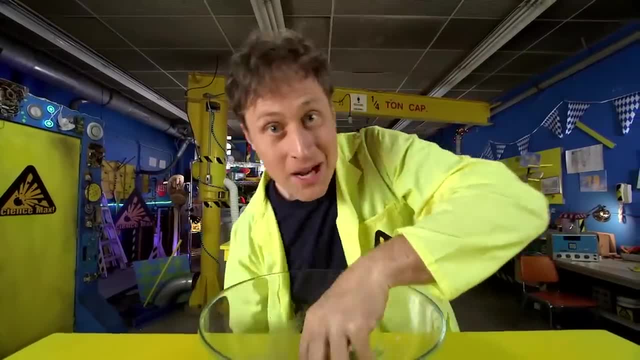 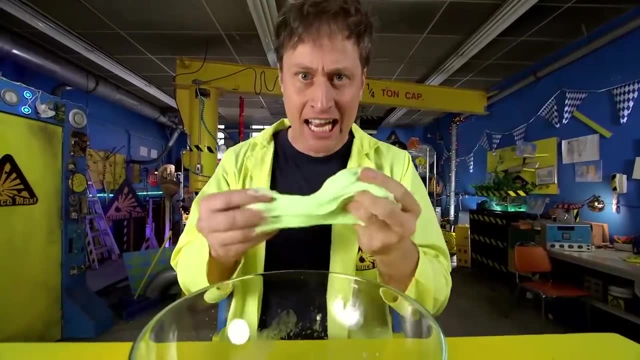 you want to use clear glue and not white glue, But that's basically the recipe. So there you go. slime, Mwahaha, Mwahaha, Too supervillain, Yeah, OK, well, anyway, we got it all right. 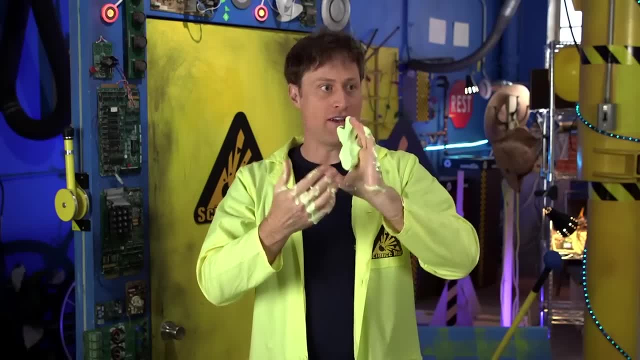 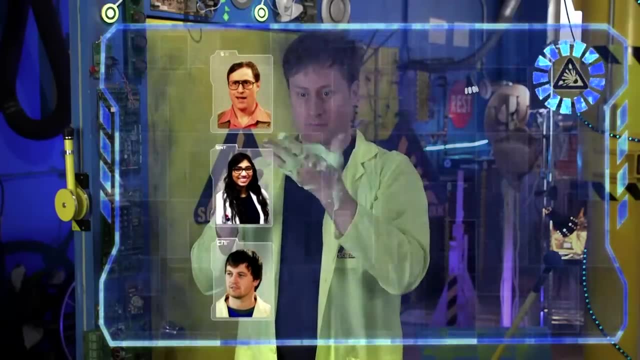 Now all you need is an expert to help me max it out. Of course, my interface is command-gesture based, so I don't know if the slime. Oh hey, there we go. Great, so you got to Uh-huh. 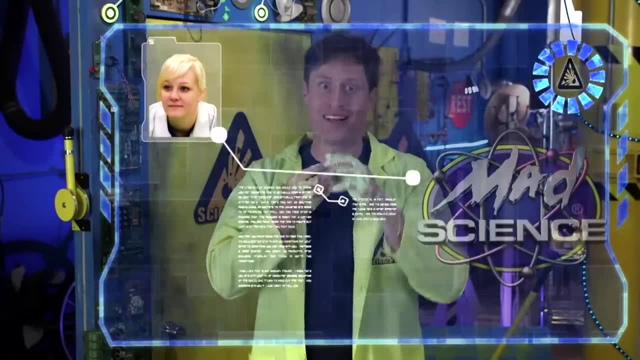 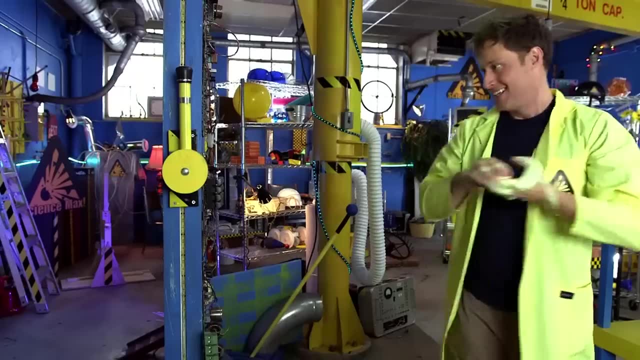 Oh, of course, Sarah from Mad Science. Mad Science, they really know their slime. This is great. OK, I got to close, close, close, close. Ah, there we go. All right, Ugh, I'm not sure bringing it through the portal. 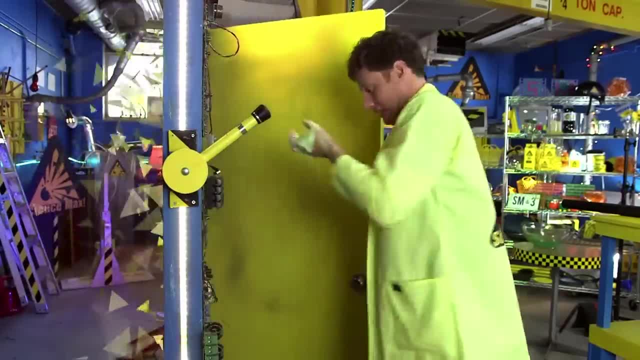 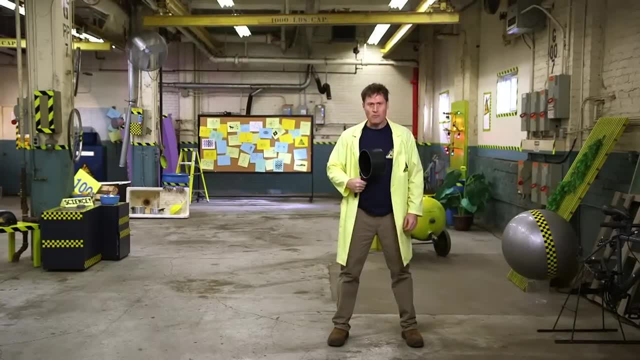 is such a good idea, but at least I'll have it on the other side. Ugh, I have a pot. Why do I have a pot? I didn't have a pot when I went through the portal. Is someone somewhere missing a pot? 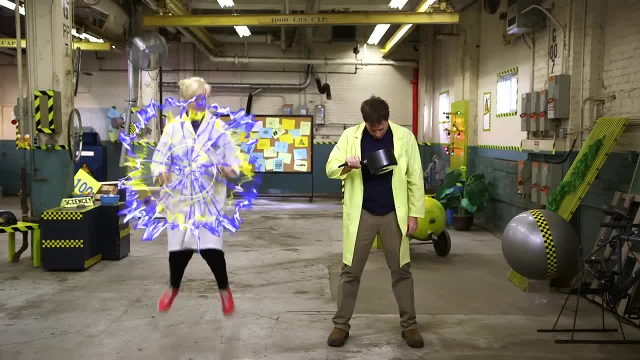 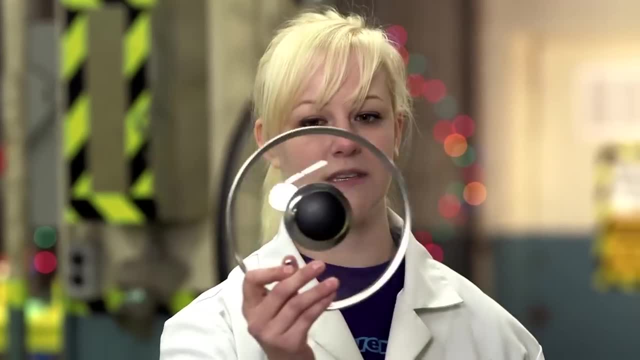 Or did it just create this pot out of nothing? Huh, Hey Sarah, Hey hi, How are you doing? Good Sarah from Mad Science, you're going to help me make some slime. Yes, I actually brought some. 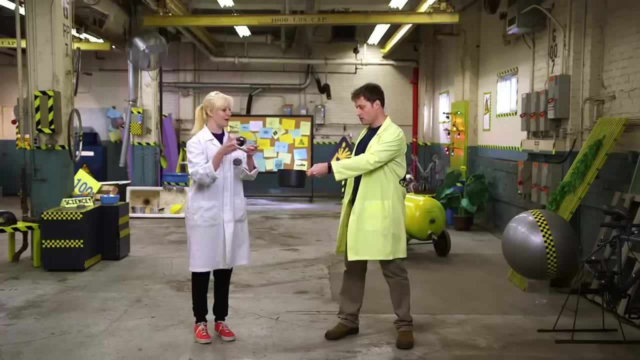 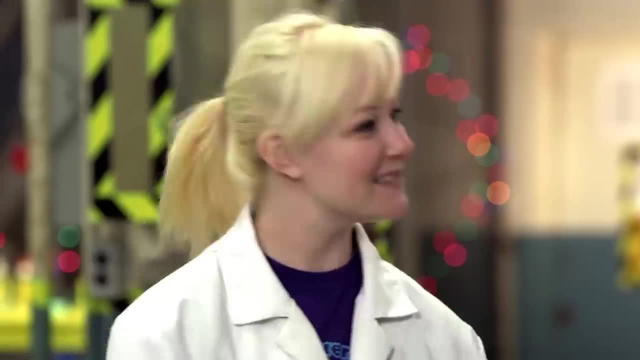 Oh, this isn't slime, This is a pot lid, Hey, Oh Well, at least we have a set. Doesn't answer any questions, though, And I guess we're going to have to make some slime. Definitely, What kind of slime do you want to make? 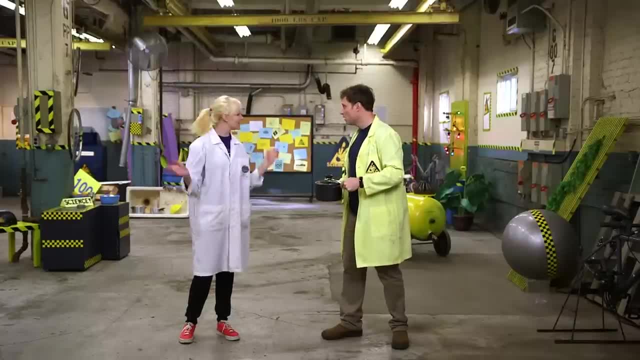 Uh, what do you mean? what kind? Is there more than one kind? Oh yeah, There are tons of different kinds of slime with lots of different ingredients and recipes. Oh, I only know the one. Can you show me all the others? 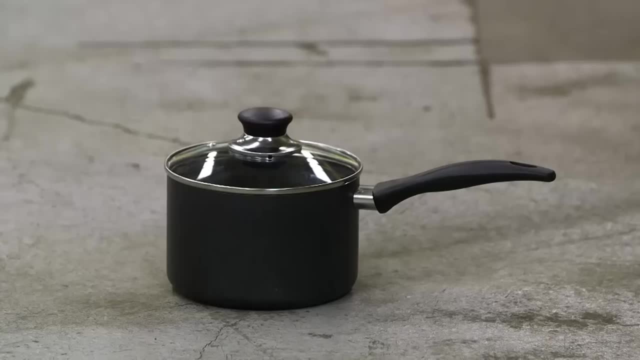 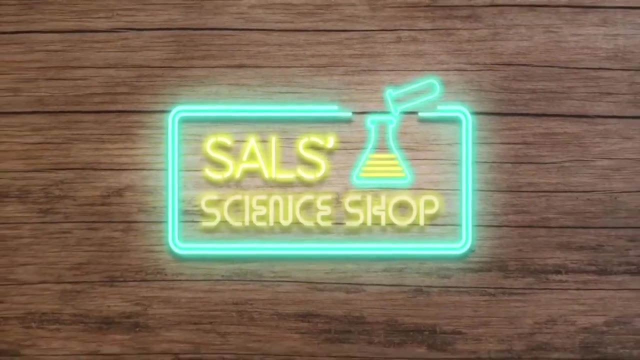 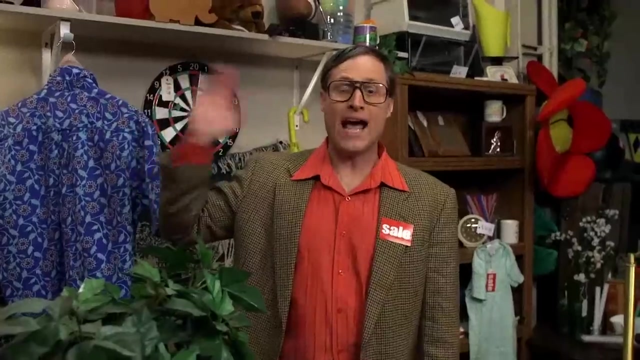 Of course Let's go make some right now. OK, great, Awesome. Come on down to Sal's Science Shop and see me, Sal, while you shop for science. This week, only Sal's one of a kind, once a year polymer sale. 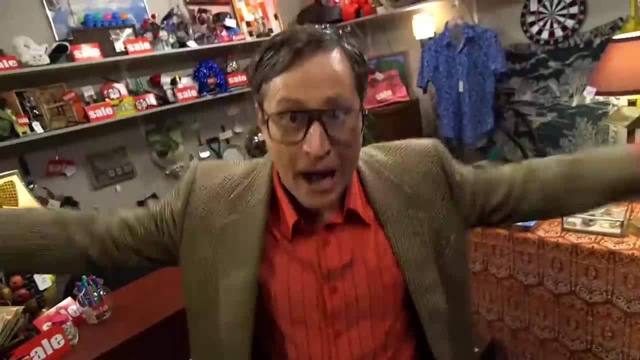 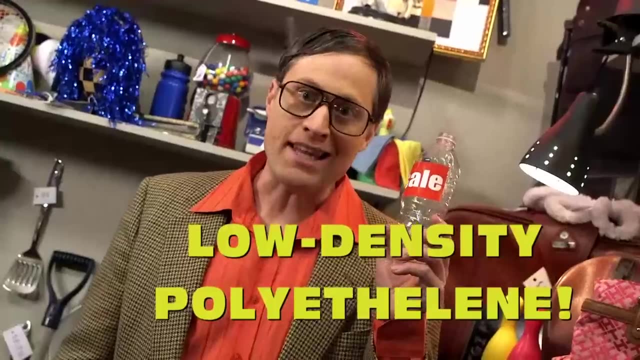 50 to 70%. 25% off anything made of polymers. Rubber That's a polymer Polystyrene. When you're eating your next meal, I recommend some polypropylene. Low density polyethylene. High density polyethylene. 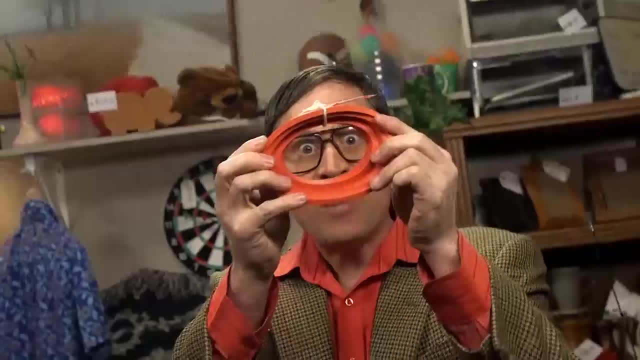 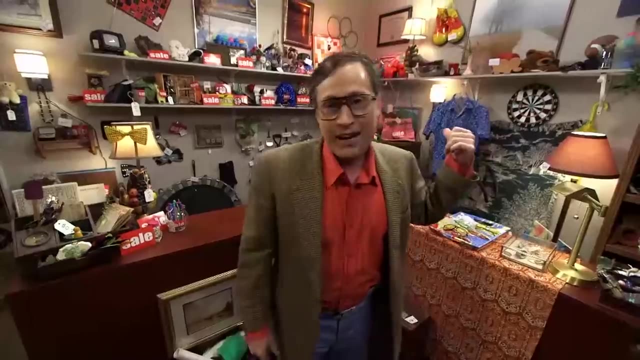 You want some polytetrafluoroethylene. We got it. We've even got polychlorotrifluoroethylene. Do they even know how good a deal this is? Because you're not going to find that kind of deal just like every day. 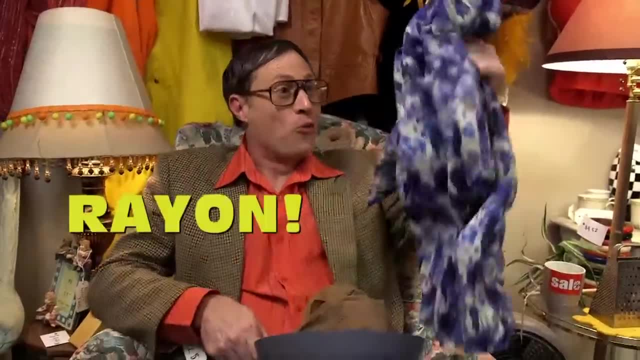 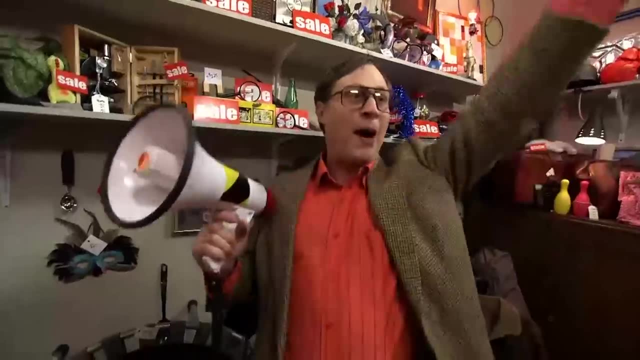 But hold the phone. Polymers aren't just plastics. Rayon, Nylon, Teflon, You name the lawn, we got it on Sale. What do we want Polymers? When do we want them? Any time, during normal business hours. 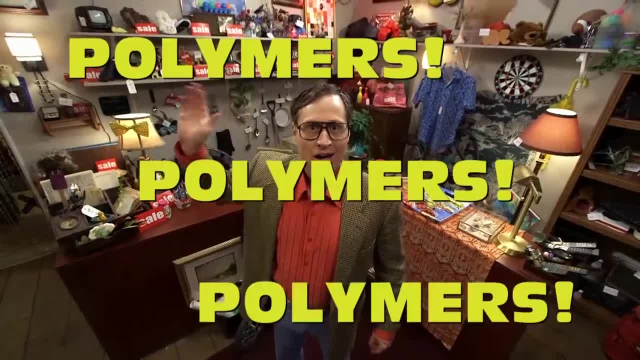 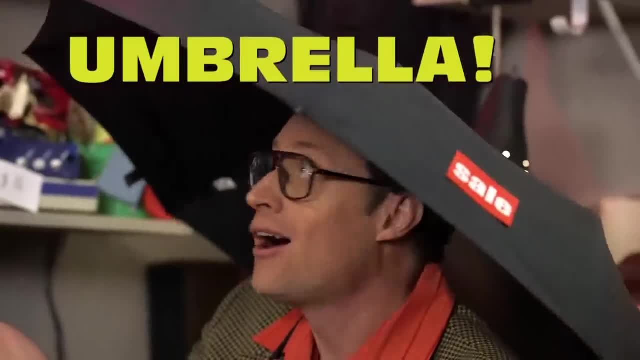 Wool, Silk, Even cotton, Polymers, Polymers, Polymers, Polymers, Polymers, Polymers. Word has lost all meaning. Glue, Paint, Umbrella, fabric- Oh yeah, Cop it. 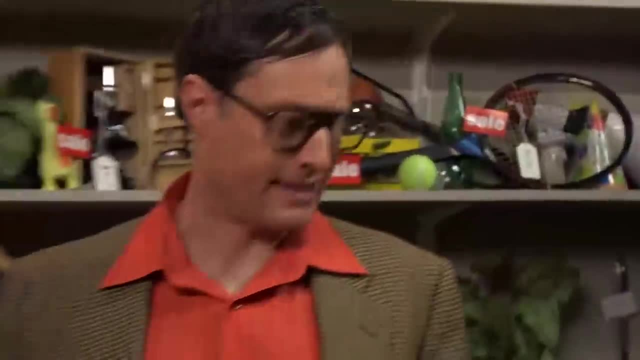 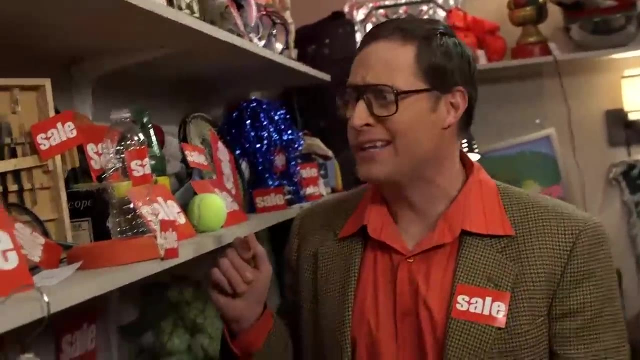 You bet that's on sale, Roberta. I'm running out of sale signs. Buy it and I'll put it in a plastic bag, also made of polymers. Seriously, Roberta, we can't have a sale on everything. Oh, hey, hey, even you, even me. the proteins in our bodies. 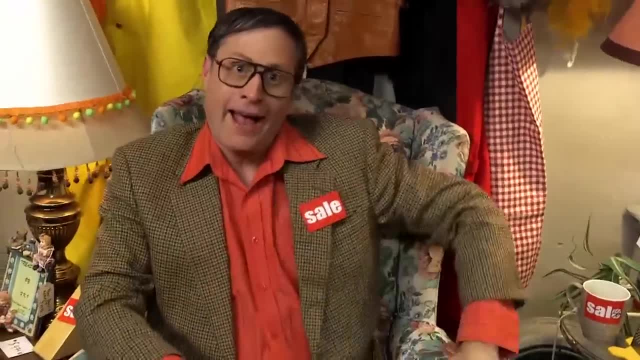 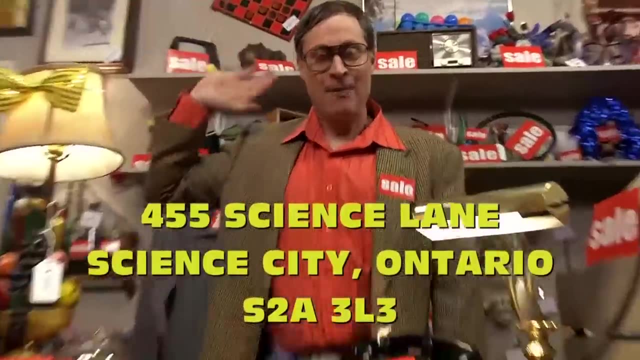 even our DNA, all polymers. So come on down to Sal's Science Shop and get a great deal on your polymers for a limited time. I mean it'd have to be a limited time, right, Roberta? Because I mean I can't discount everything. 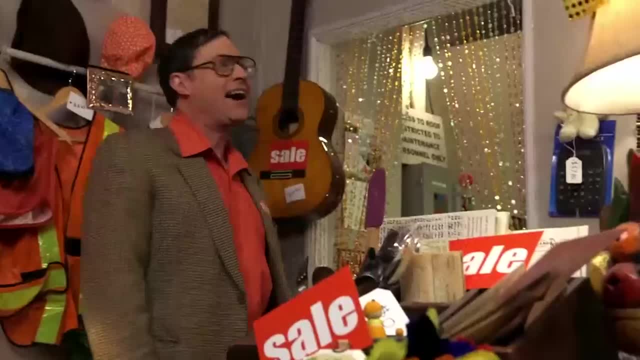 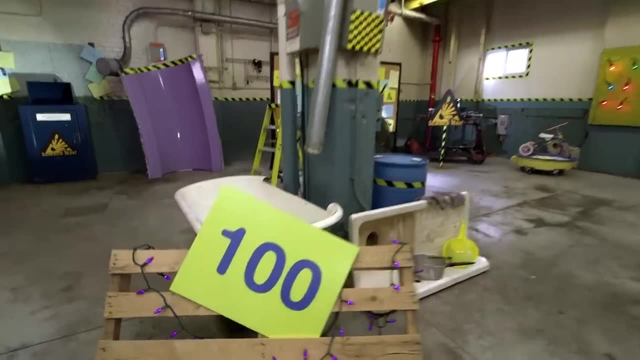 in the store at 75% off. How am I going to make any money? I mean, Are we still rolling 100 different kinds of slime? Yes, it's going to be so much fun, but we're not going to make 100 today. 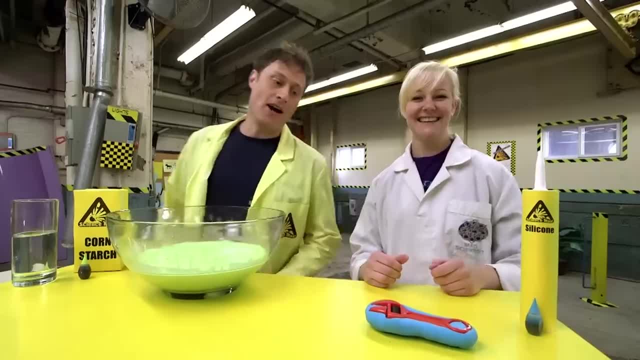 Yeah, I know We're just going to do our top favorites. Yeah, it's going to be super great. All right, what are we starting with? So our first slime we're starting with today is some really cool molding slime. Now, this slime actually, if you leave it out overnight. 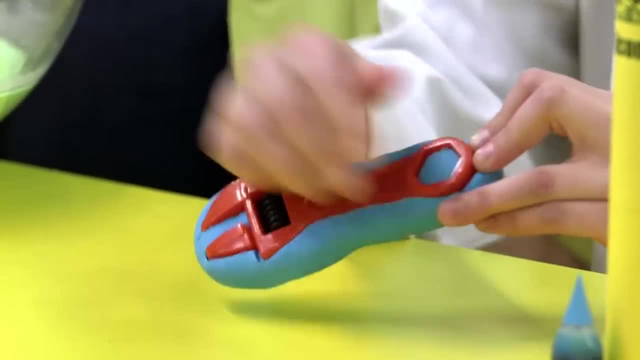 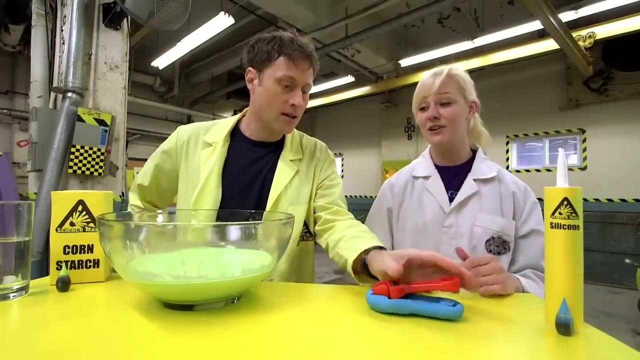 it'll harden and you can make an imprint of whatever you like. So here we made an imprint of our little tool there. So we're going to look at it a little bit. So we're going to make a little bit more liquidy slime. 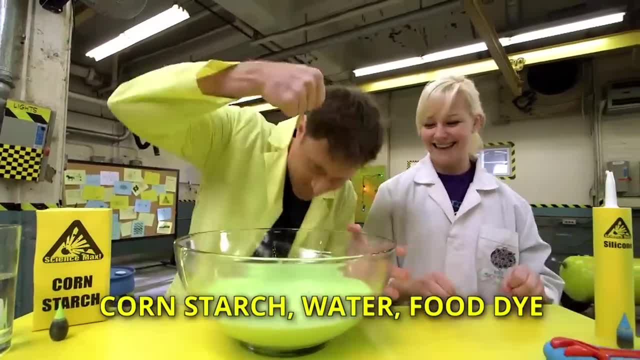 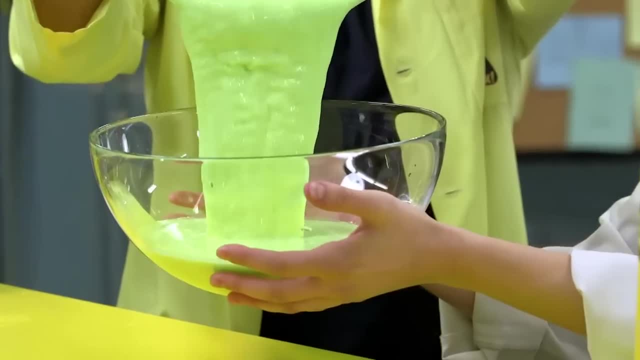 starting with this one over here, which I believe you already know about. This is cornstarch mud, Exactly. You hold this Sounds good, I'm going to hold this and we're going to try pouring it. Whoa, Oh, so see, it's like a liquid. but then, if you do it fast, 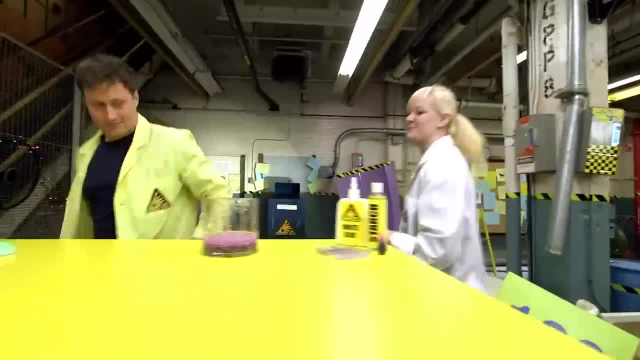 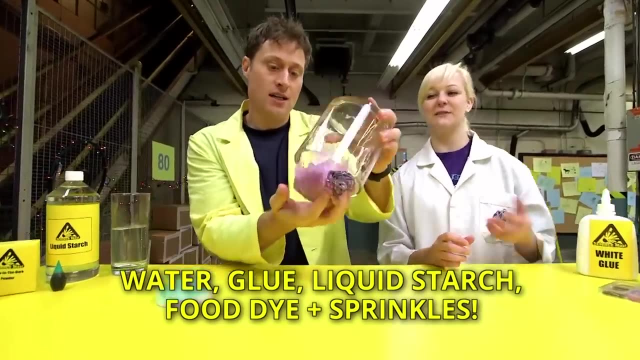 it's like a solid. All right, what's next? Over here we have some other really awesome types of slime. So right over here we have some crunchy slime. Crunchy slime, Exactly. Why is it crunchy? Now, it's crunchy because we've actually added a few beads. 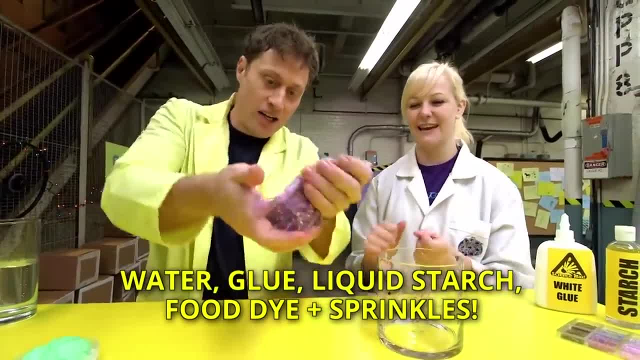 inside of it to make it crunchy. So this is some really cool, awesome slime Here. you take half And you can feel the beads as you stretch it out. It's so cool. This is why this one is a little harder to clean. 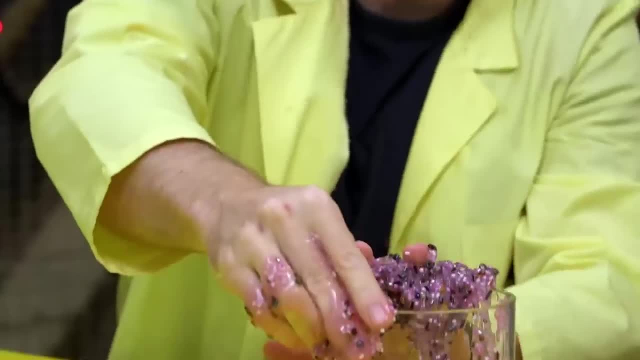 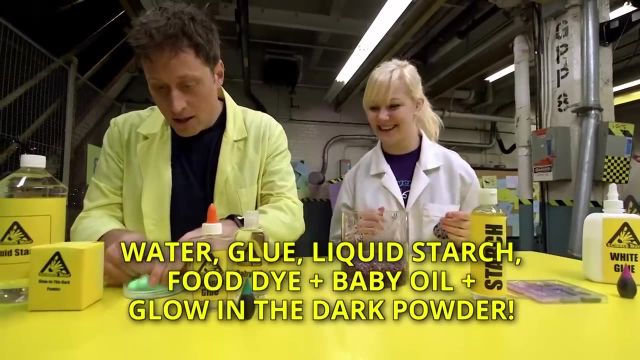 Exactly. I'll just do that, All right. so what's next? So next we have some really cool glow-in-the-dark slime. Glow-in-the-dark slime- Yeah, it's so awesome. Ooh, Look at how much it glows. 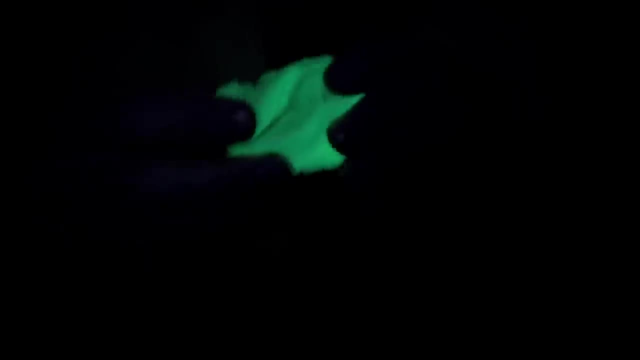 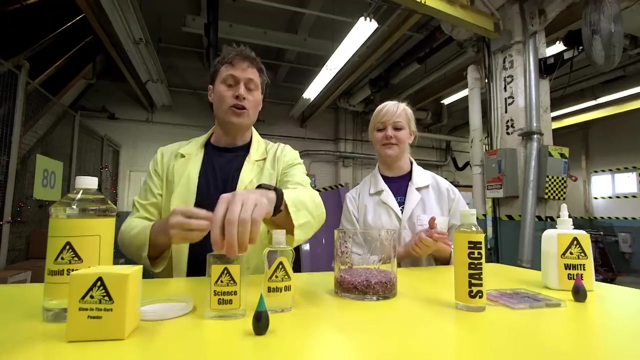 That glows a lot, That's super glowy slime. So to do the different kinds of slime, we need the polymer, Yes, And then the thing that sticks the polymers together, Exactly So: the glue is the polymer, Glue is the polymer. 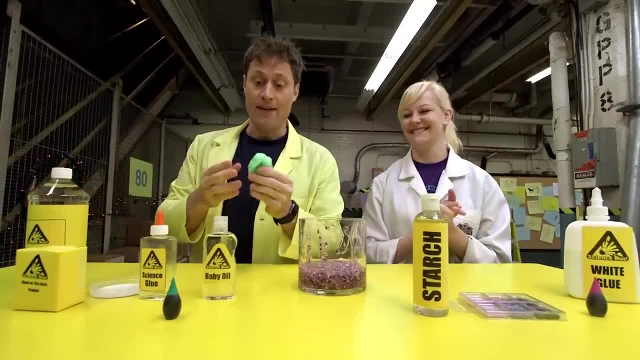 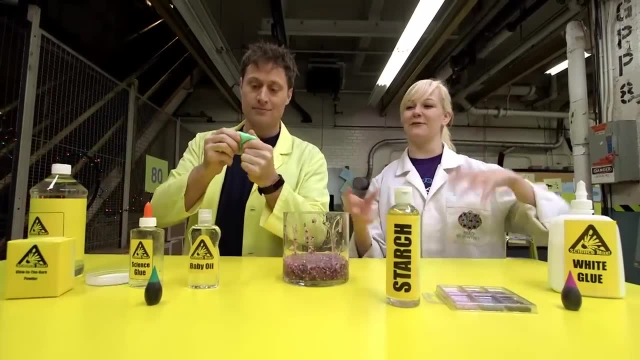 And the starch is the thing that bonds it. Yes, Uh-huh, Very cool. And then you put the thing in that makes it the kind of slime. Yes, right before you add the bonding component, because if we keep adding stuff after it's already made, 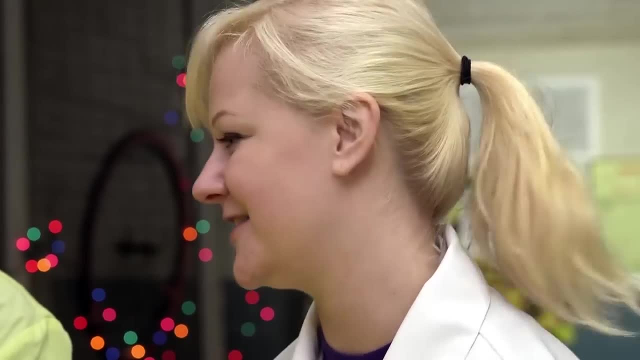 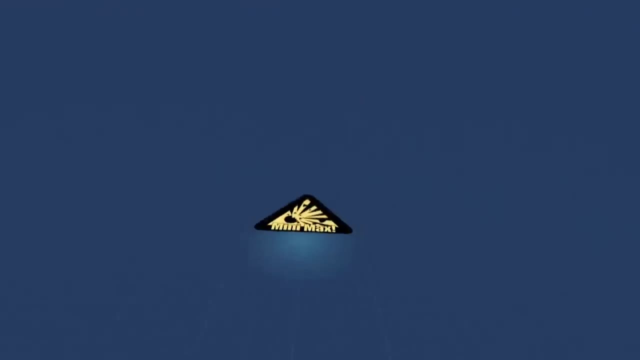 it unfortunately won't be able to take it, So we add our powder before we add our starch. in this situation, Should we go on to the next thing? Yeah, let's move on to the next. slime, More slime. Little Max, Whoa. 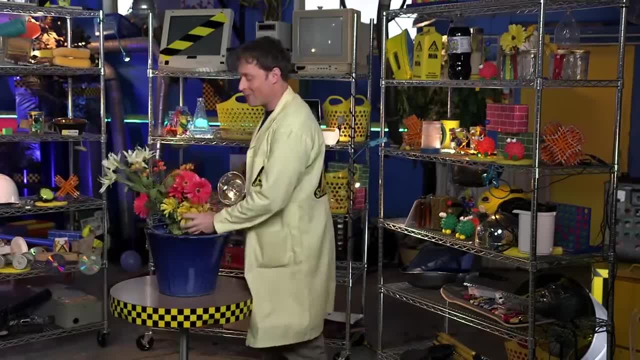 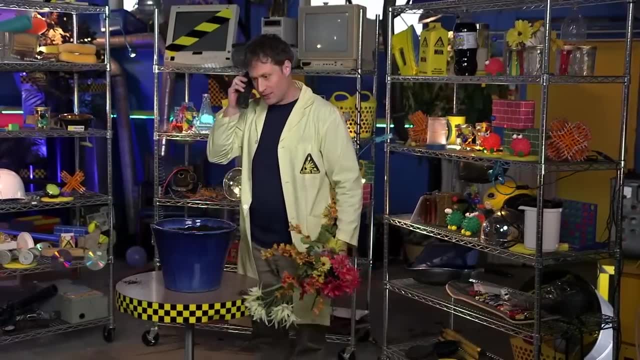 Plastic is great and plastic is everywhere. But the problem with plastic is it isn't very biodegradable. It doesn't break down in the environment. I'm still on hold. Oh well, There you go Back for another couple of years, I guess. 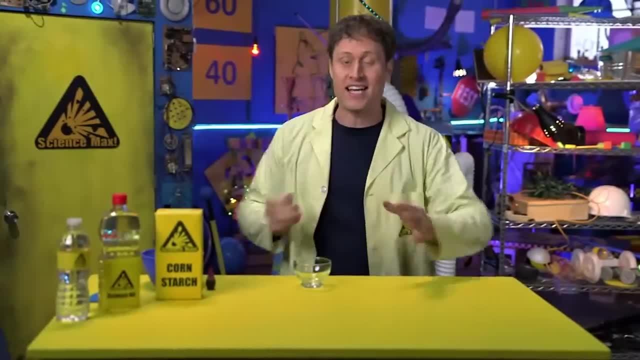 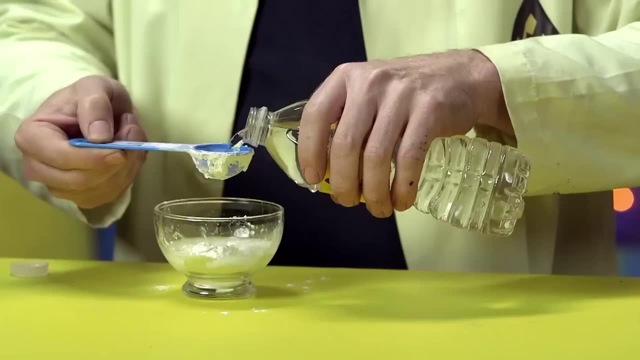 But here's a way that you can make bioplastic. It's fully biodegradable because it's made of natural materials. The recipe is easy: Two parts cornstarch, three parts water, a few drops of cooking oil And some food coloring to make it whatever color you want. 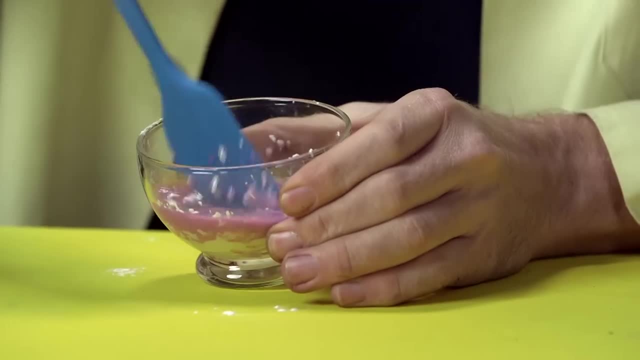 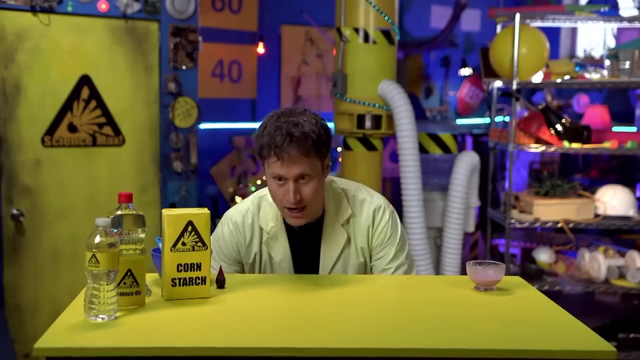 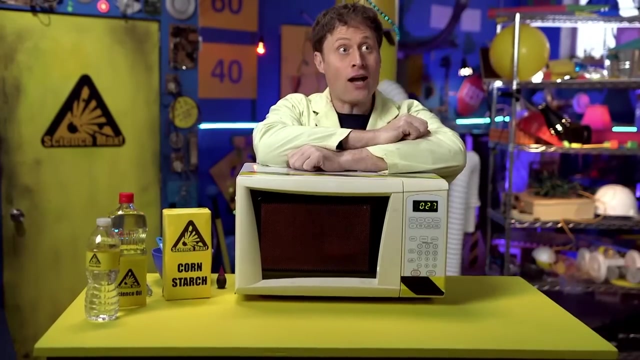 Purple science, purple. Mix it up and it turns into a paste. Now what you'll need are two things: One an adult And two a microwave. Put it in for 30 seconds. Clock wipe. There we go. 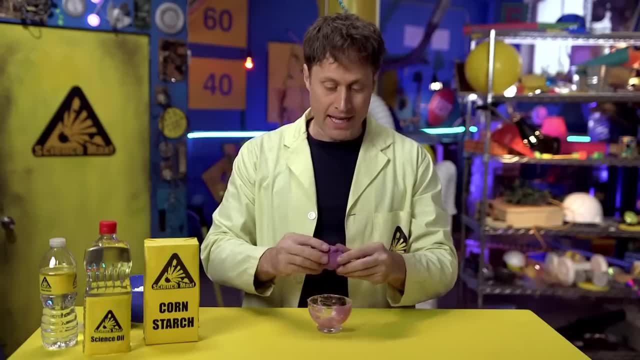 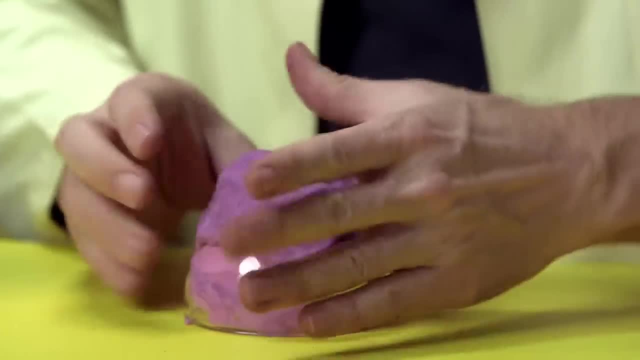 Then take it out and mix it some more until it cools down. Then you can pull it out and use your hands to sculpt it into a shape, The shape of something else. Once you put it all the way around, you can turn it into a little flower pot. 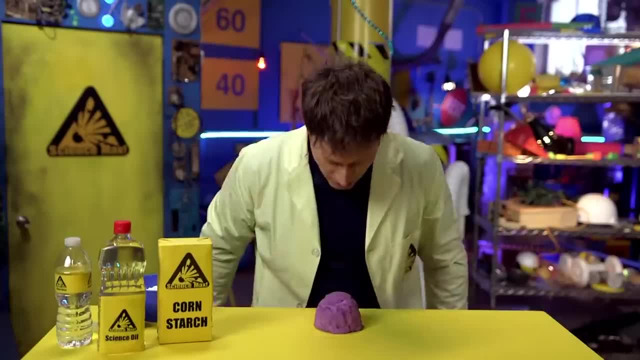 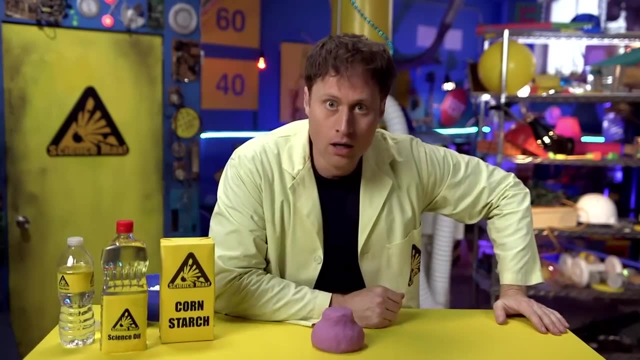 Once you've sculpted it, you need to wait for it to dry, which will take about a day. Clock wipe After waiting a day. what It's been a day? Oh, You have something made out of bioplastic. 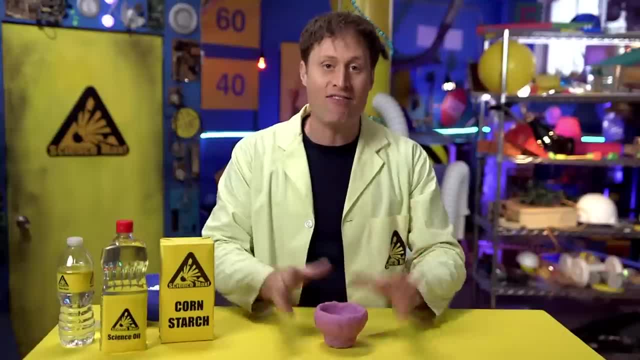 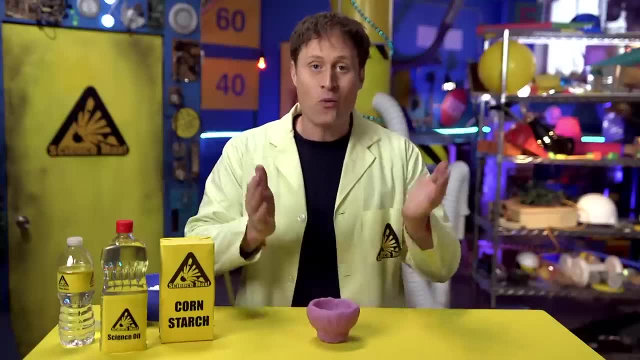 like this little flower pot you can use to grow a small plant And then, when it grows big enough, you can take this biodegradable flower pot and plant it right outside. You put this side in the dirt and this pot will biodegrade. 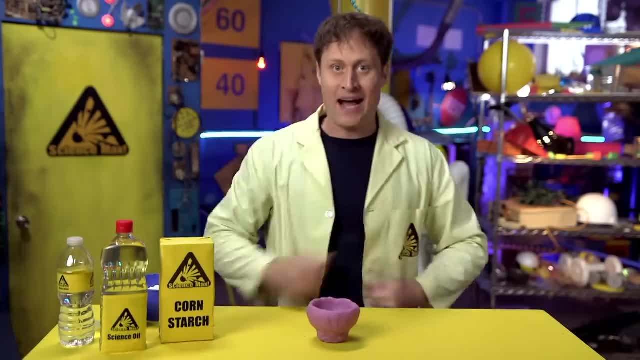 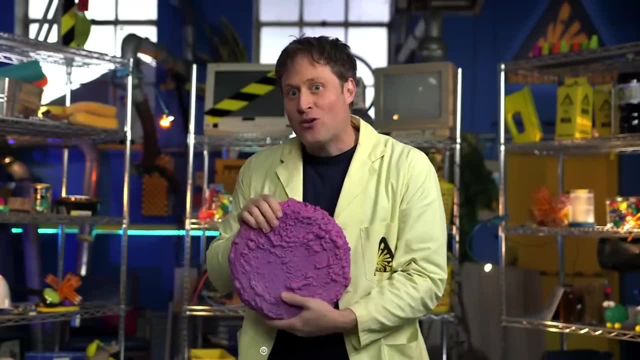 and turn back into dirt. Pretty cool, right? Well, let's max it out. Biodegradable frisbee. Check it out. It's a frisbee, but it's biodegradable. So you throw it around in the park. but if you lose it? 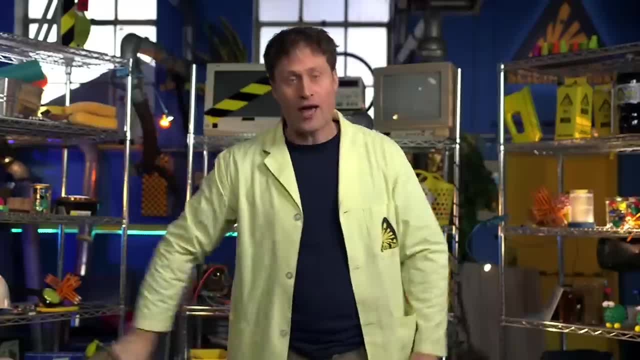 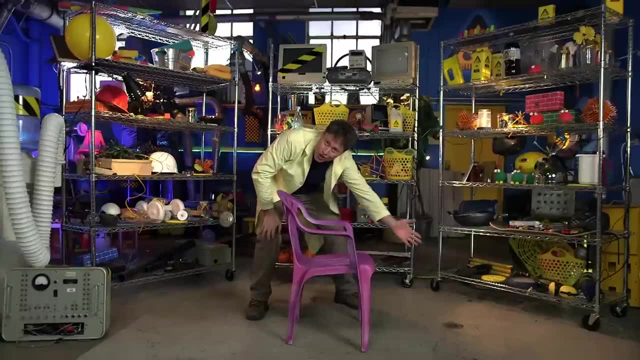 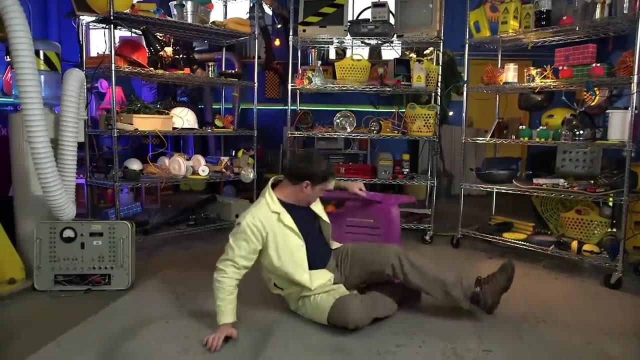 it turns back into dirt. Ha ha, What, not enough. OK, Clock wipe Biodegradable lawn chair, Use it for one season and then return it afterwards. I think this is one of my best science max. OK, Bioplastic lawn chair not as strong as regular lawn chair. 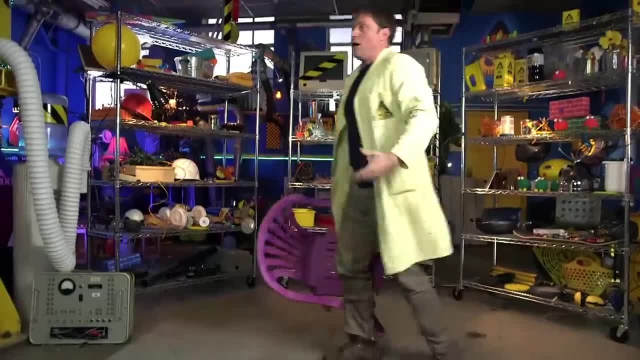 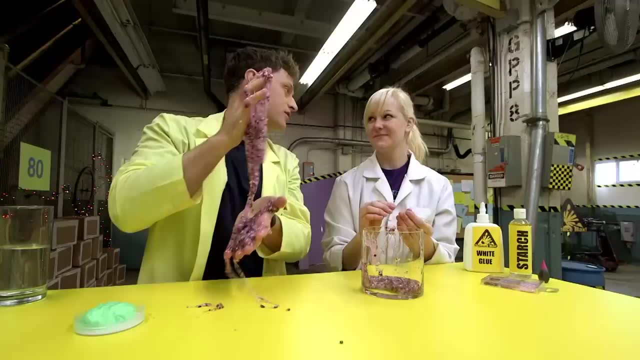 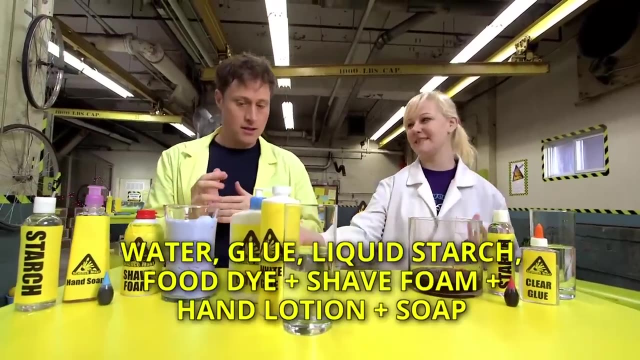 We've learned that lesson now, so that's good to know. I mean, how would I have known if I hadn't tried it? Sarah and I are looking at different recipes for slime. All right, what do we got here? Over here we have some amazing foamy slime which has so, so. 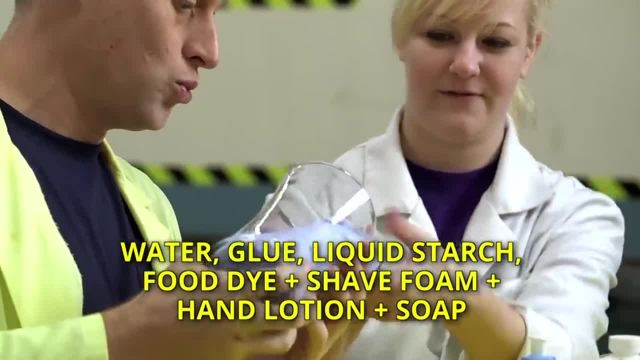 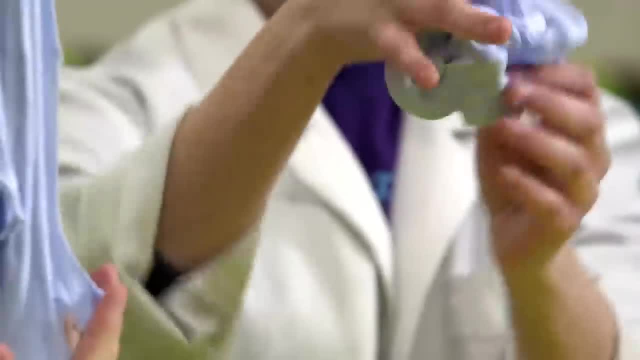 many ingredients in it Here. watch what happens when you start pulling it out: Ooh, Wow. So it's like super stretchy and super fluffy Here. that's great. OK, now you got to hold yours. You got to hold this end. 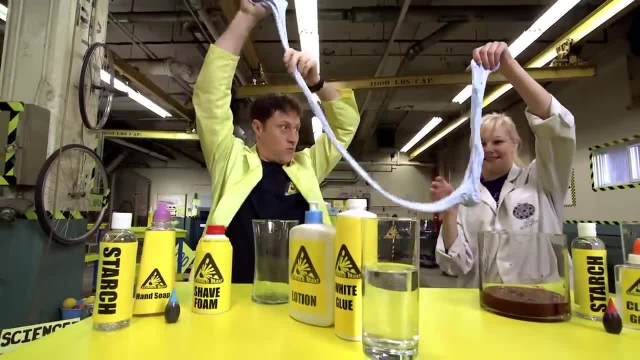 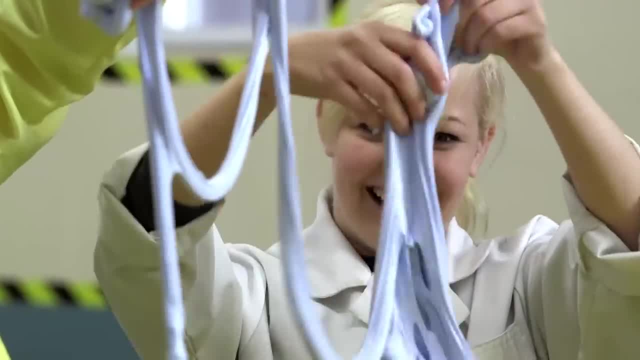 Then you take and then take some more, And then we take that And then, yeah, It gets thinner and thinner and it becomes more and more lines of foamy slime. Yeah, And the last kind of slime we made today is some classic. 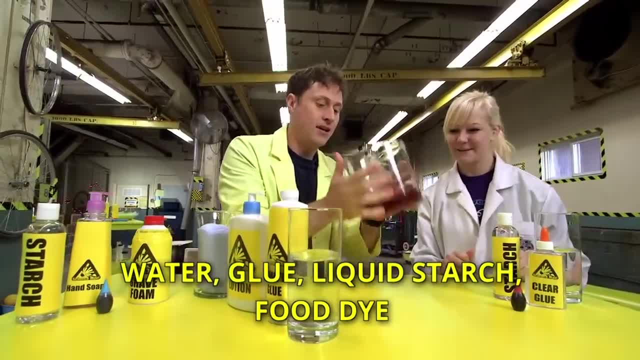 clubber slime. Ooh, It's so much fun. Now, why do you think it's called clubber slime? Because it's? is it really a slime? It is a slime. yeah, It's super fun and it's super stretchy. 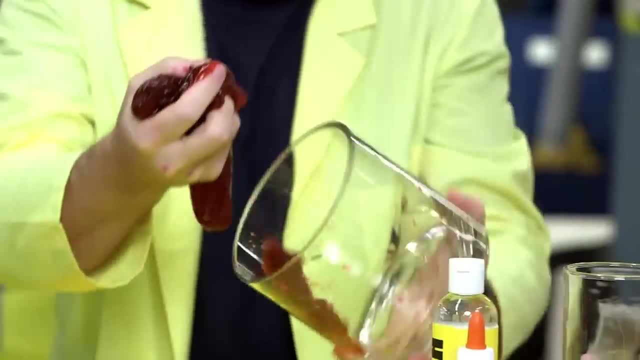 Oh, OK, I get it. Look at that And it's sort of like like a little bit like gelatin. It is almost like gelatin. Here you can have some, There you go. Whoa, Oh, oh. 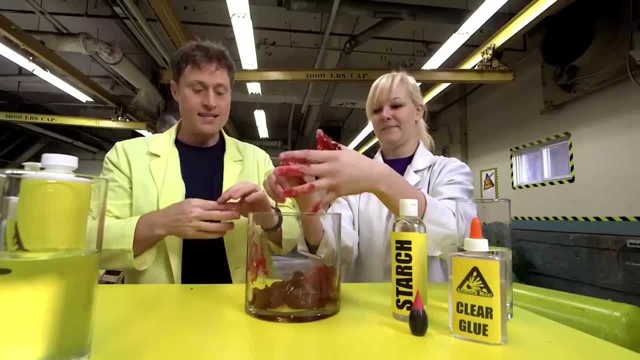 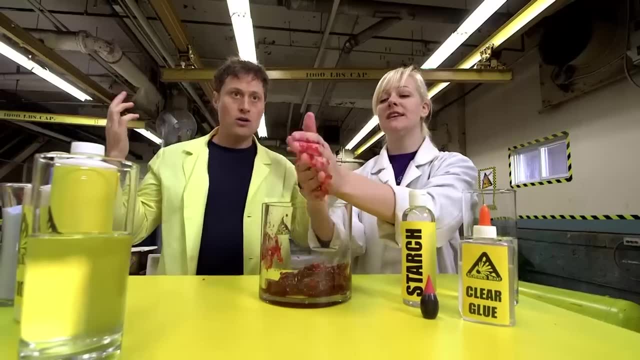 All right. so, Sarah, now what we need to decide is how we're going to max it out Right, Like, should we just get a lot of slime? That sounds like a really good idea, But we are going to need something to put it in, because we can't just 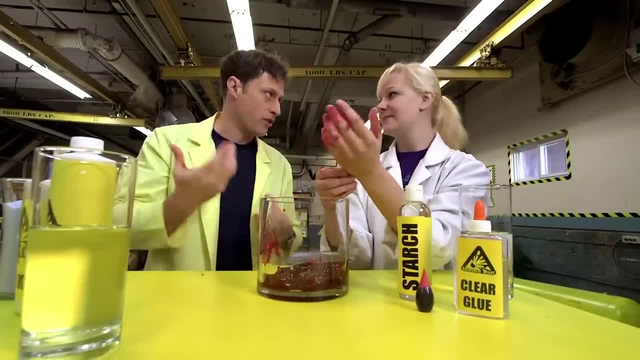 have slime all over the floor. OK, you're right, So we'll get. we'll get some sort of container thing, Yeah, And we'll see how much slime we can make, and then we'll just play with it and see what happens. 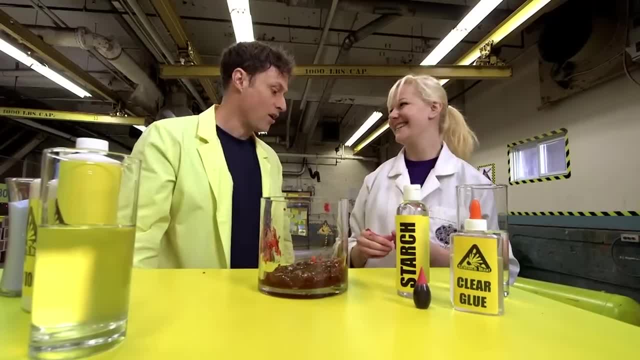 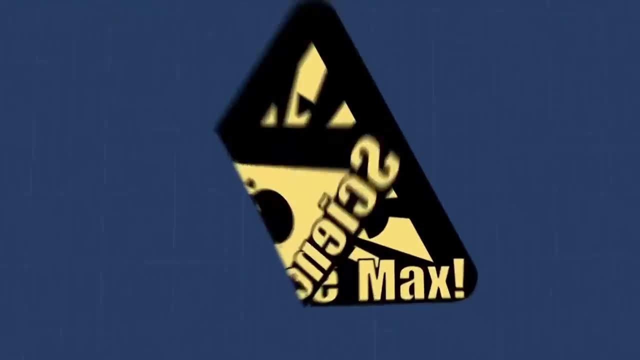 Sounds good And we will experiment, because it's science. Yeah, OK, high, high five, Careful high five, so we don't splatter, OK, good, OK, let's go. This is like Mini Max. 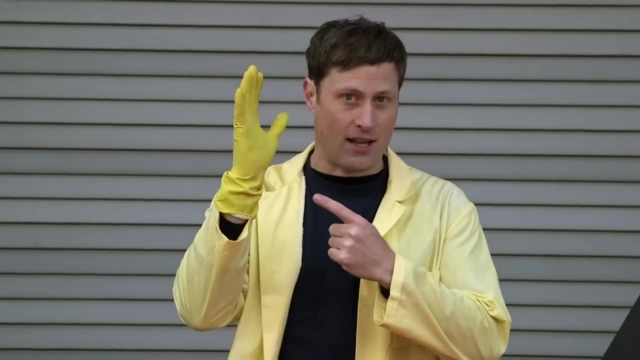 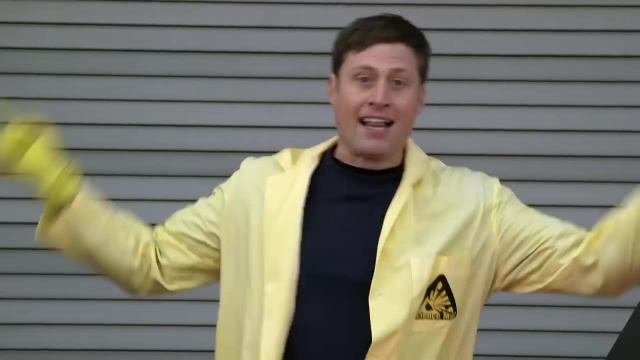 This is a rubber glove. Well, actually it's a latex glove. What's in it? What's the difference? I will get to that in a second, But I'm sure you can agree it's super stretchy. How stretchy. 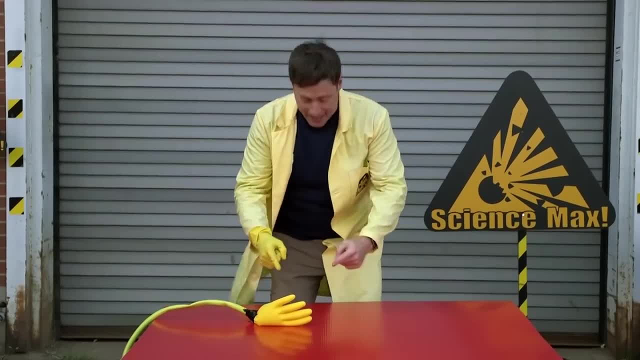 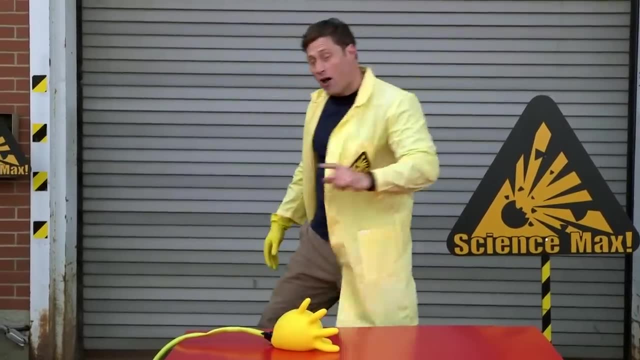 Let's fill a rubber glove with water and see how big it gets. So difference between latex and rubber. Well, it all comes from a rubber tree. Well, actually it's a fake tree. It's just to show you how it works. 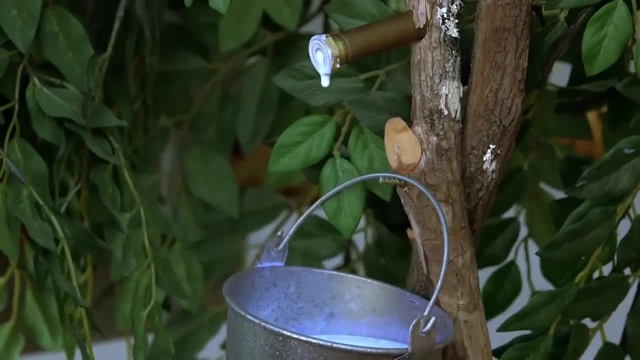 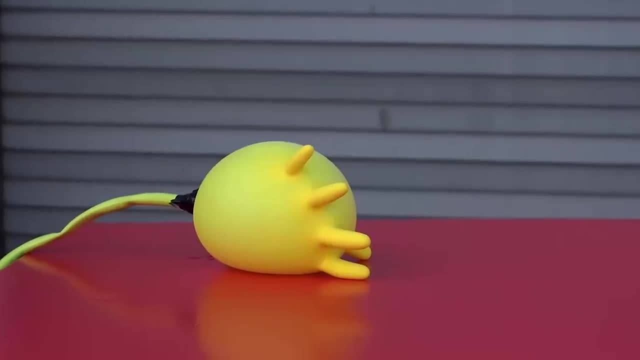 The sap of the rubber tree is collected just like this: There's a spigot and then the sap goes out and it's collected. It's the same way that the sap for, maybe, maple syrup is collected, And this, this is natural latex. 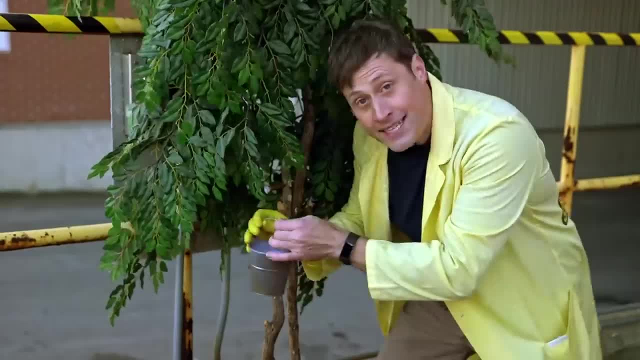 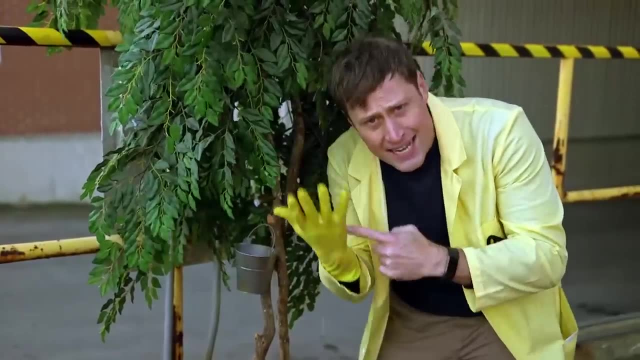 If it's dried out, it becomes natural rubber. Latex generally means the liquid form and rubber means the solid form. But wait then, why is this a latex glove? The glove is not liquid. What's the deal? Well, generally, latex means water-based or liquid. 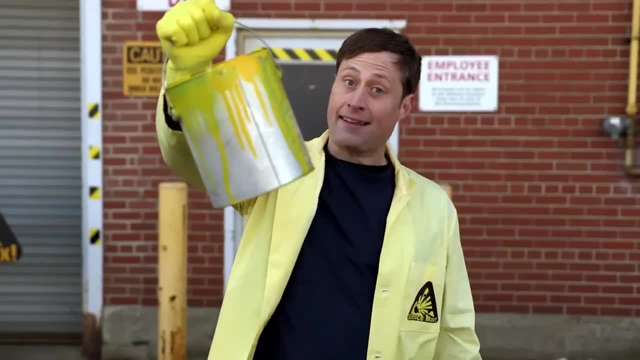 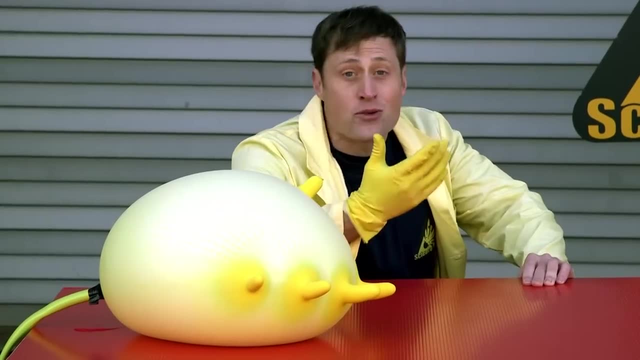 like latex paint, But it could also mean synthetic latex. That's latex, But it's man-made and doesn't come from a rubber tree, So we call rubber gloves rubber gloves because they used to come from rubber trees, But now they're usually made out of man-made latex. 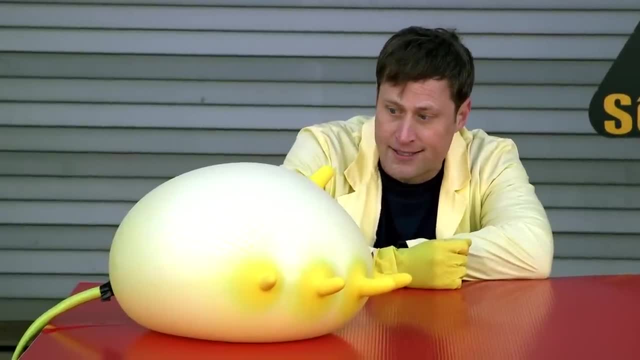 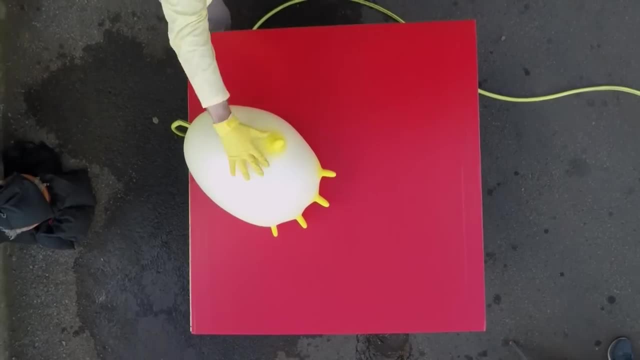 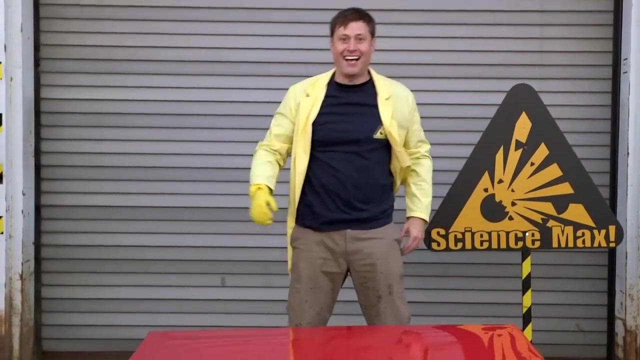 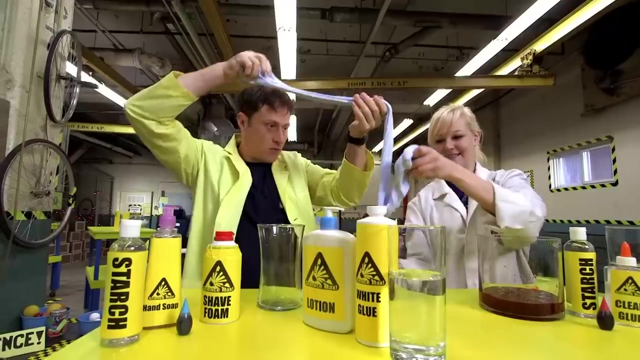 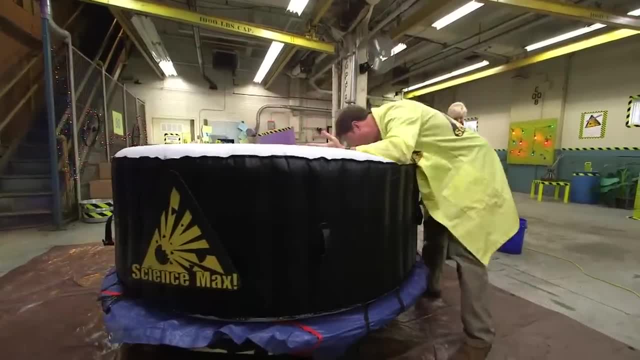 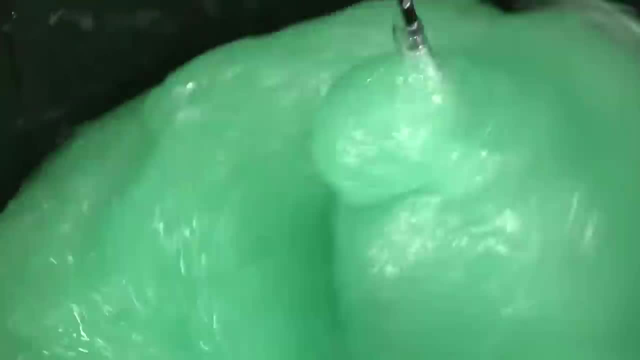 How Maxed out tub of slime, Whoa OK. so how do you feel Is it? are we mixed up enough? First, we mix up a bunch of slime in a garbage bin. So, with the polymer chemistry, the polymer, 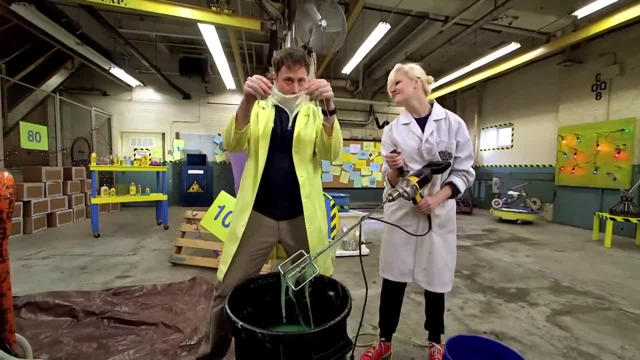 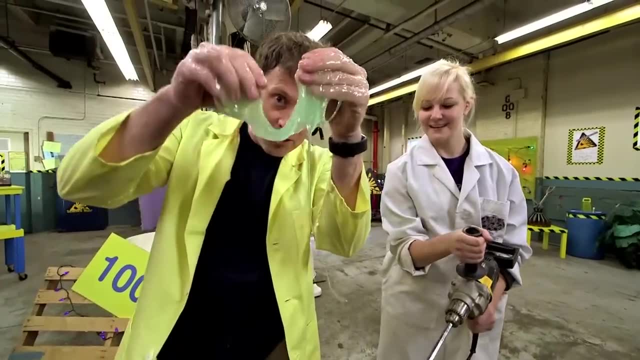 is generally a liquid, right Yep, And the bonding agent makes it stick together. So the more we use, the more of a solid we get, Exactly, yeah. So we want to split it and make it sort of of halfway between a liquid and a solid, and i think we're exactly at the right stage. it looks. 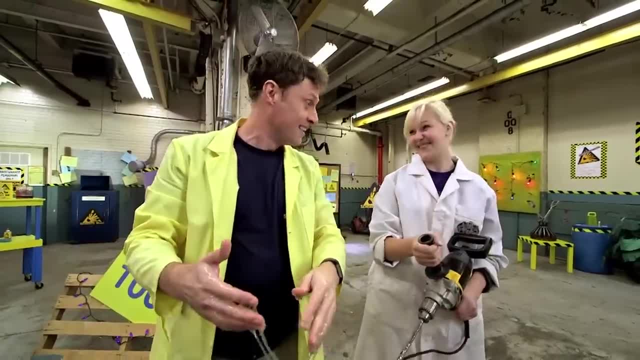 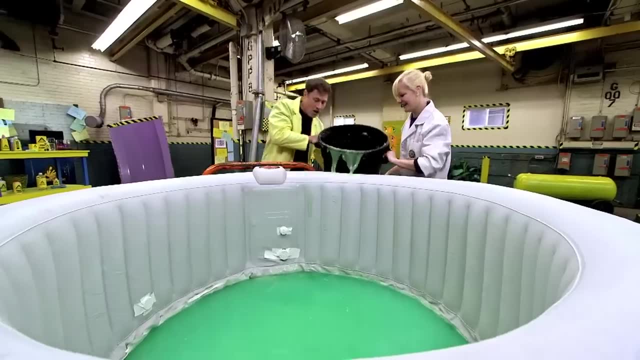 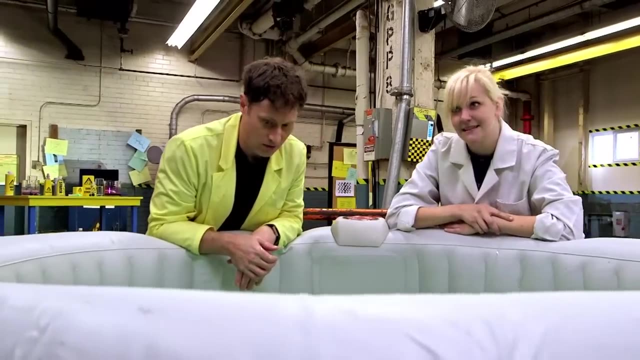 perfect, oh yeah, okay, so let's dump this garbage can in, all right. all right, then we dump it in. it turns out we needed more slime. um, i don't think that's gonna be enough. i think we might need some more slime. yeah, how much more do you think we need? so we added 11 more. 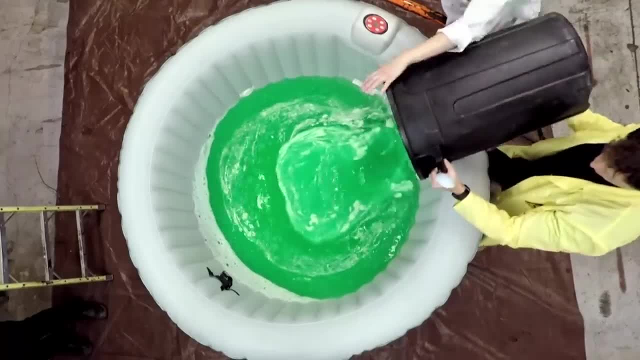 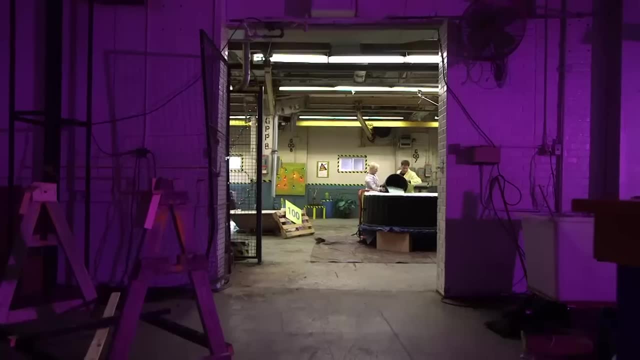 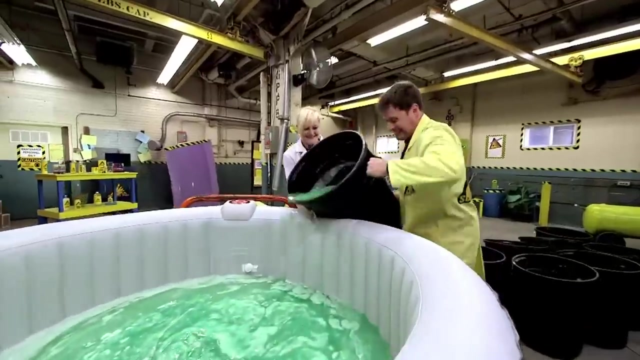 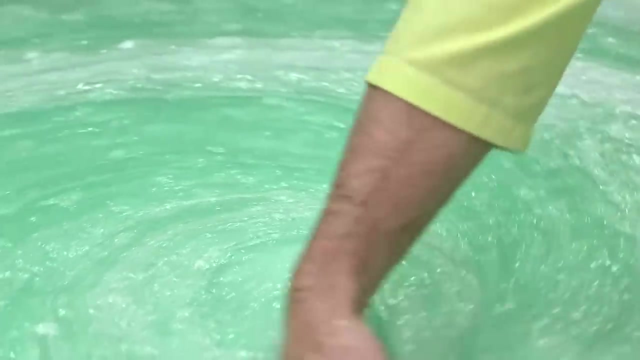 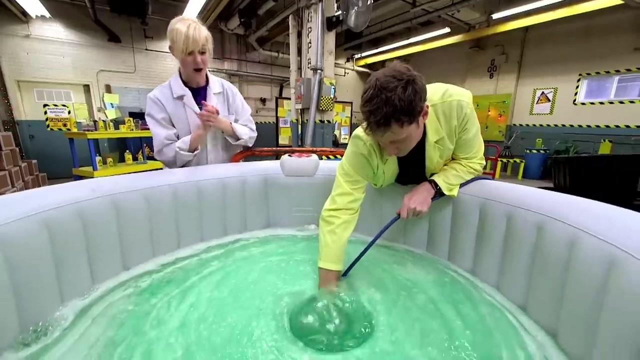 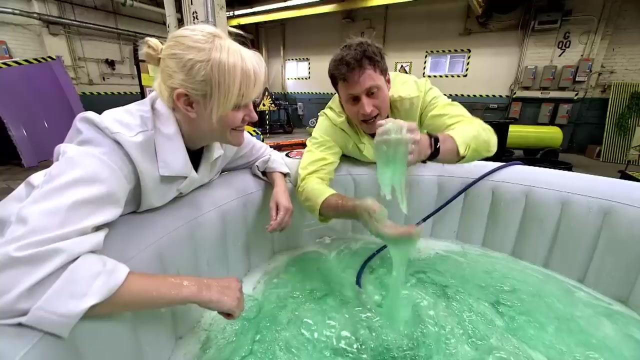 ah, delicious. last one, last one, oh yeah. then we experimented. oh yeah, we have a giant, giant tub of slime. ah, because the slime is stretchy, it created amazing bubbles. so do you think i could blow a bubble with the slime? well, maybe not you, but definitely the air compressor. 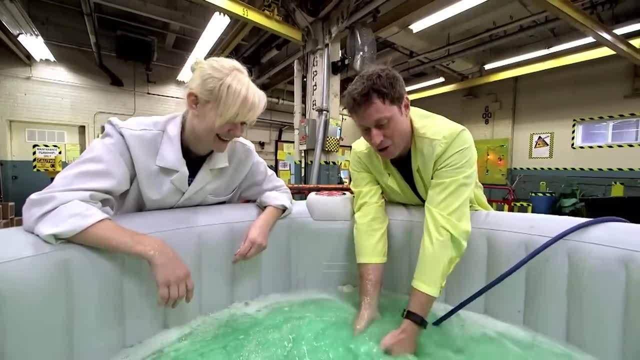 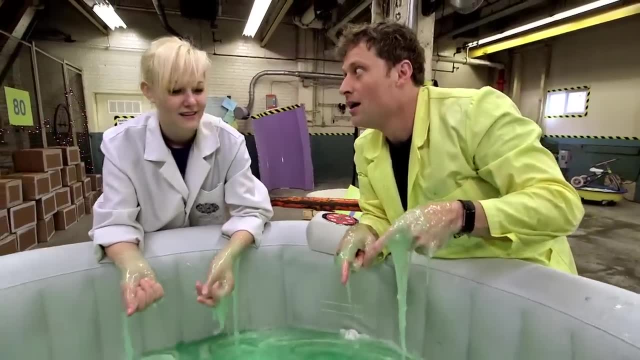 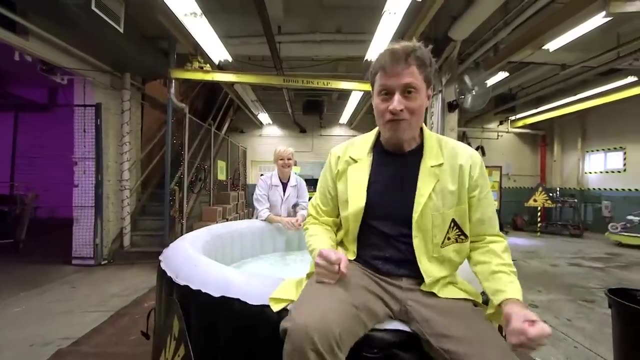 no either. no, i'd have to just put it on my face. i think i've already got it on my face. then there was only one thing left to do: we get in this slime. can we do that? we can totally do that. this is science. maps. that's so exciting. going swimming in slides. who's going first? you are, i am. 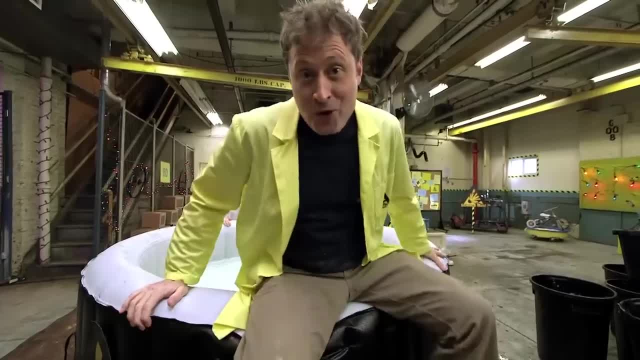 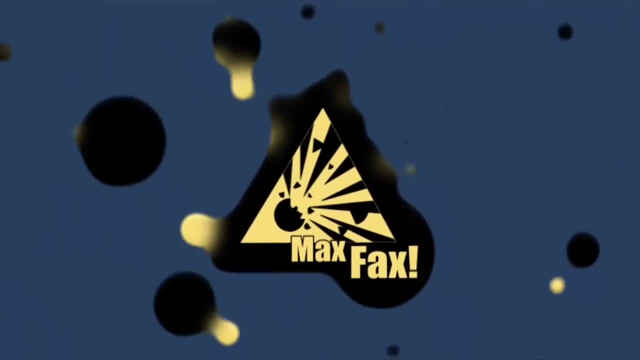 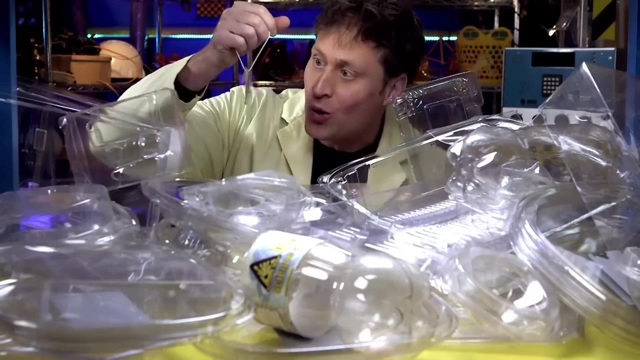 obviously all right. this is how science max does. polymers: three, two, one. plastic is everywhere, but what can we do with it aside from recycle it? well, we can reuse it to make cool plastic charms, but you're gonna need the right kind of plastic and you need polystyrene. 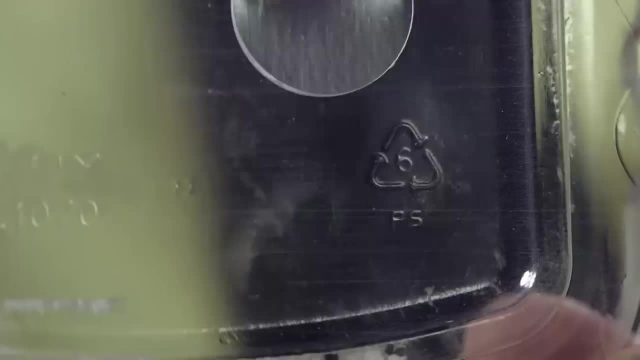 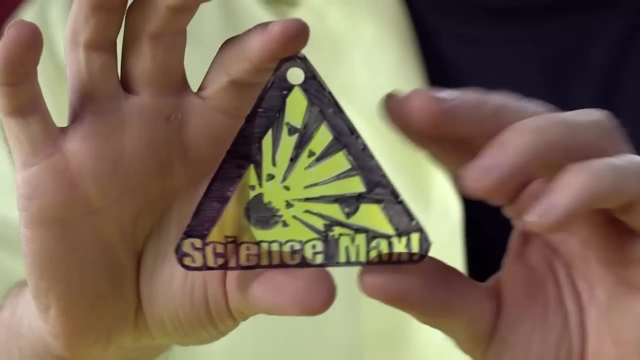 Just look for the little number 6 inside the recycle symbol. Cut out some plastic and decorate it however you want. There we go, Ha-ha. Check it out The Science Max logo Also. I've made a couple other things. 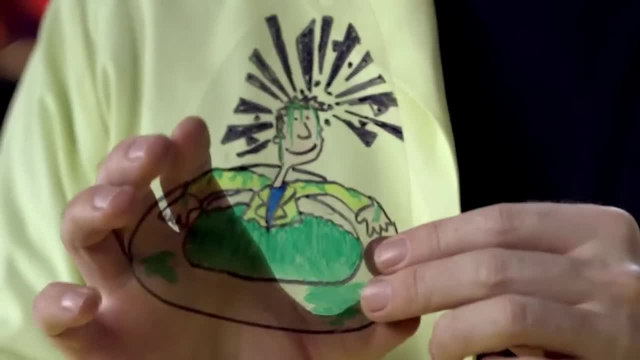 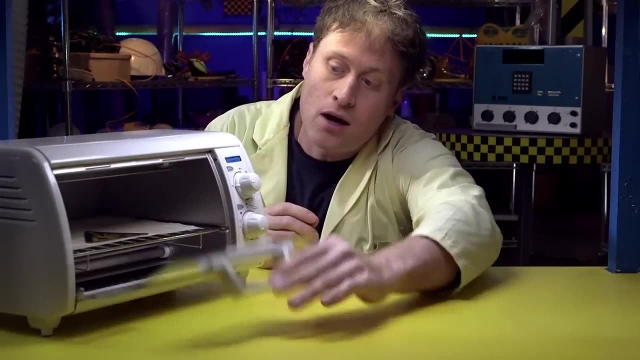 I've got a chemical symbol, an atom, and this is me in some slime. Then get an adult to help you. put it in the oven or Booster oven at 350 degrees. It only takes a few seconds for the plastic to shrink to one-third its size. 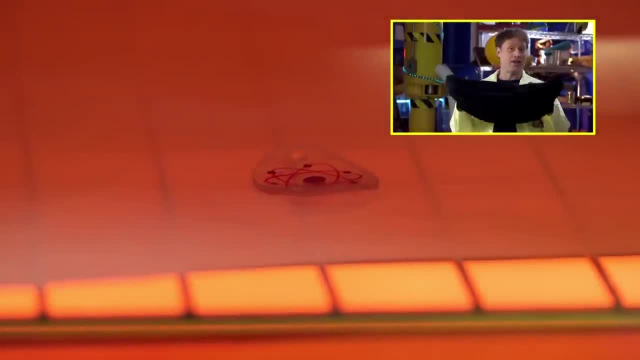 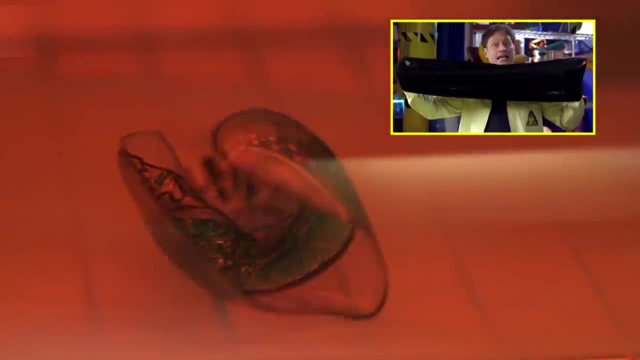 The reason why this happens is when plastic is manufactured it's heated and stretched out and then cooled and it sort of freezes in that stretched-out shape And when you reheat it it shrinks back down to the unstretched shape. Get your adult to take it out and wait for it to cool. 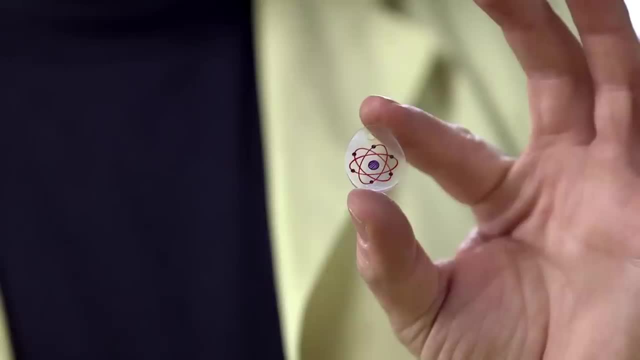 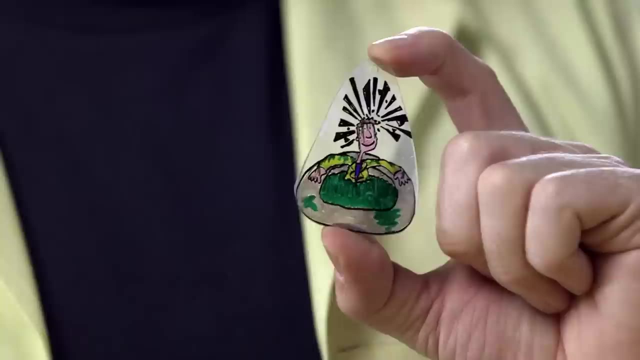 and you'll have yourself some small plastic designs you can use for key chains, bracelets, name tags, bookmarks, whatever you want, all using the power of polymers. Awesome, I'm going to make all of those. What was that? What was that again? 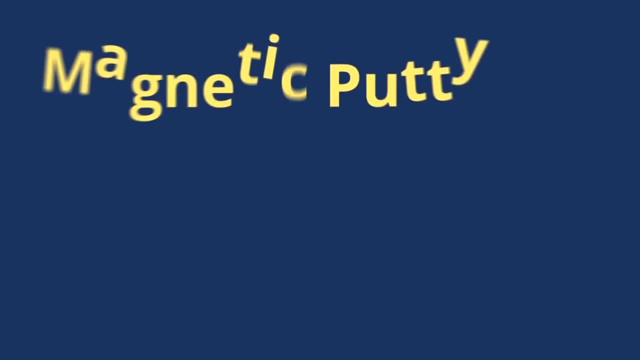 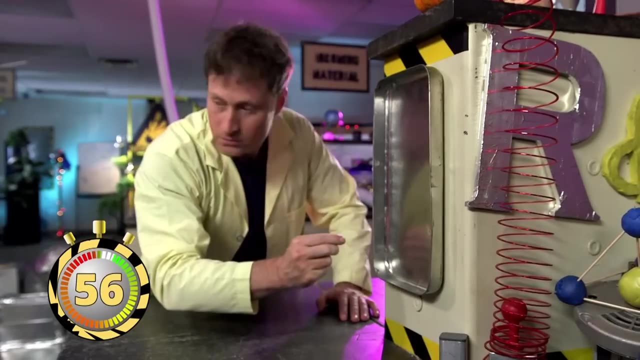 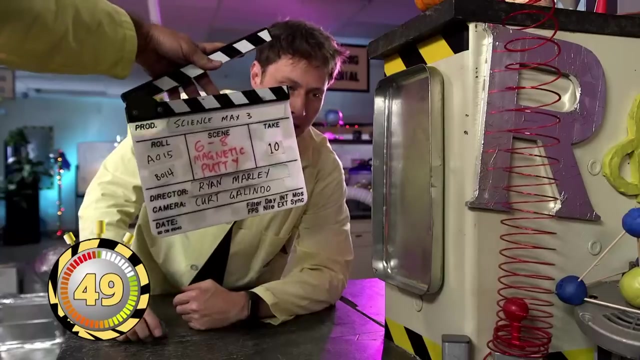 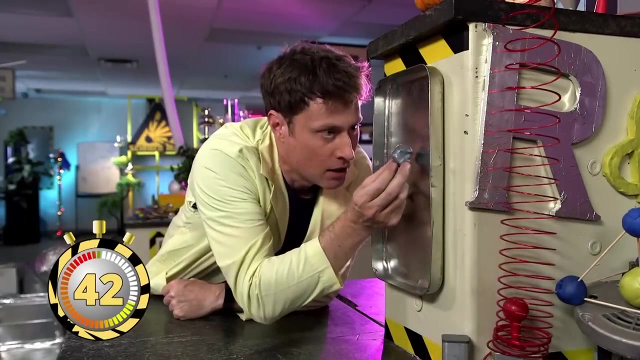 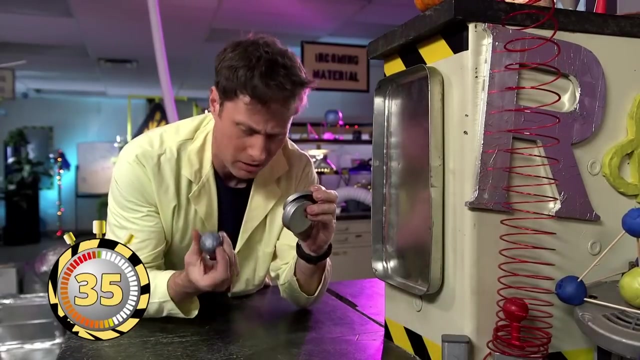 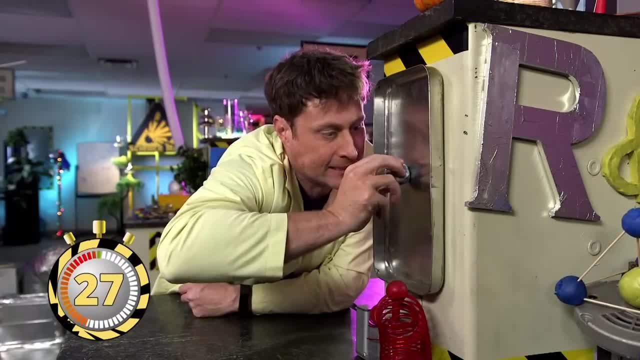 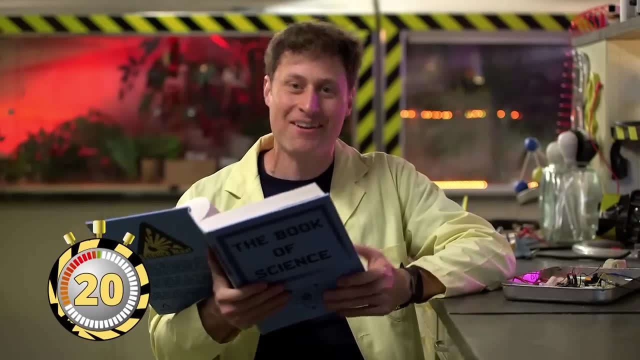 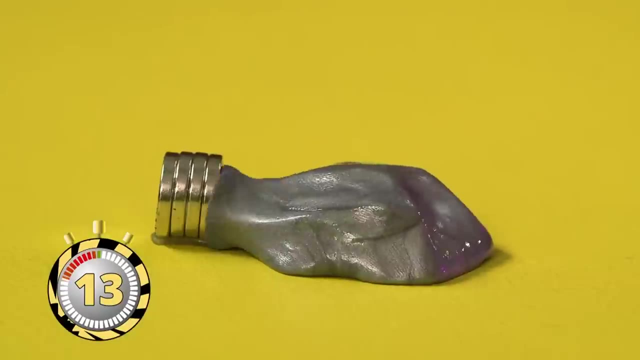 I can't count this high. This is magnetic putty. Ha, Magnetic. Oh, it's not a magnet, It's attracted to magnets. Oh, that makes more sense. This is magnetic putty and this is a magnet. The putty is made of polymers. 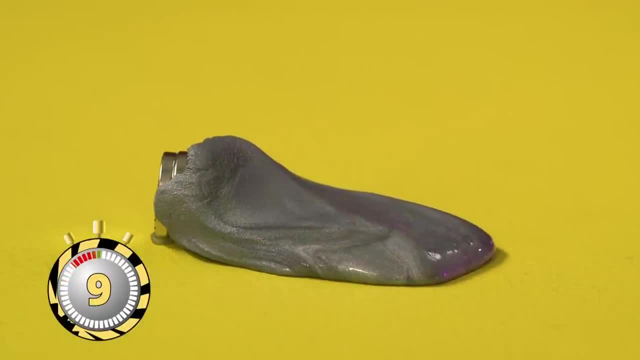 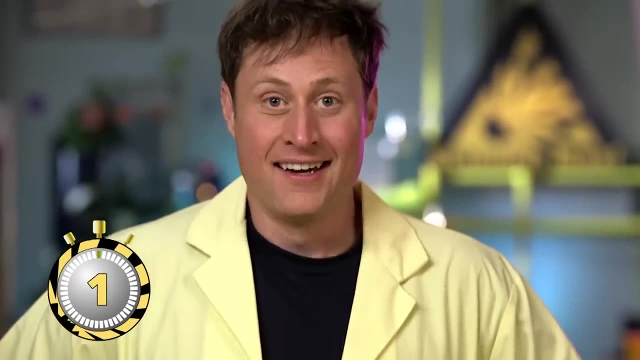 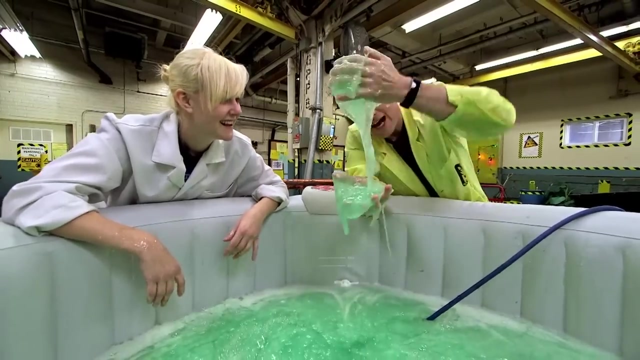 which means it can flow over itself. It also has lots of iron filings in it, which is why it's attracted to magnets. This is what happens over several minutes, And there you go: Magnetic putty. Okay, so where were we? 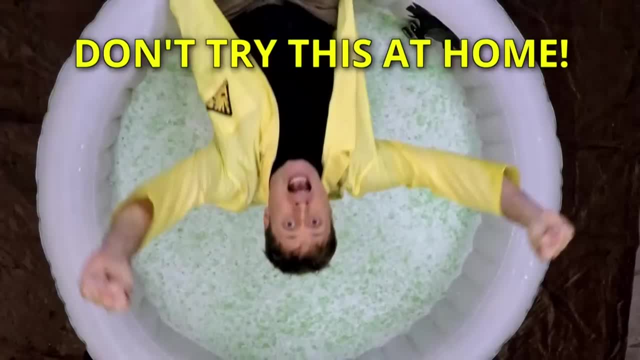 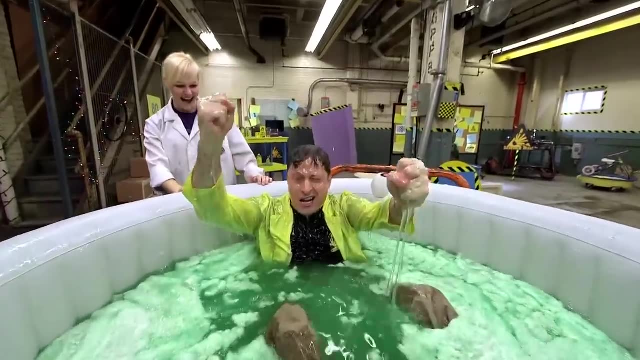 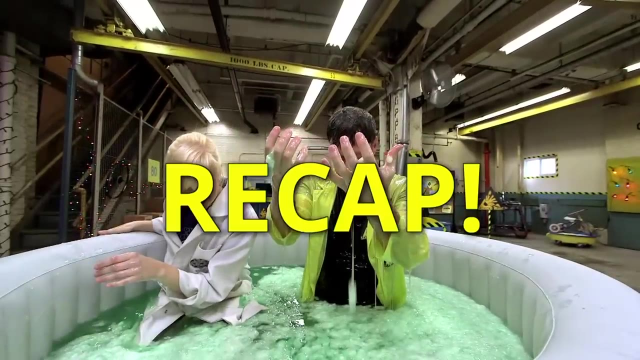 Oh yeah, Three, two, one yeah. And remember, don't try this at home Slime. Sarah and I enjoyed our maxed-out tub of slime. So let's recap. Slime is made of polymers. Polymers come in a lot of different forms. 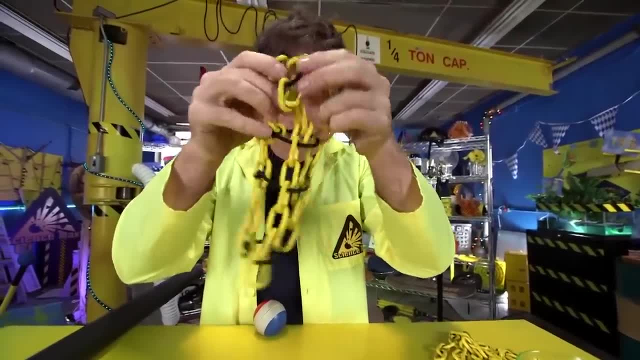 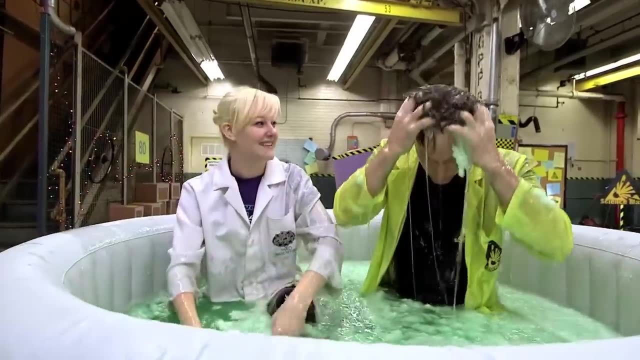 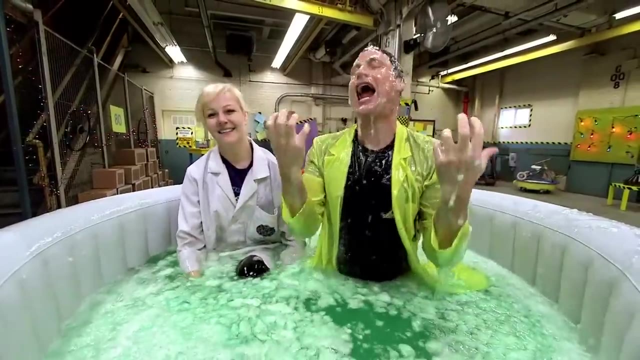 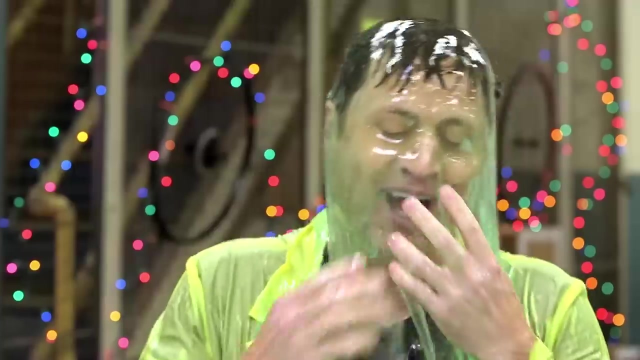 It's all about long chains of molecules, And none are more fun to swim in than slime. Do I have slime here? Ooh, yeah, definitely Slime here. Oh, slime, Ha, ha, ha, Ha, ha ha. 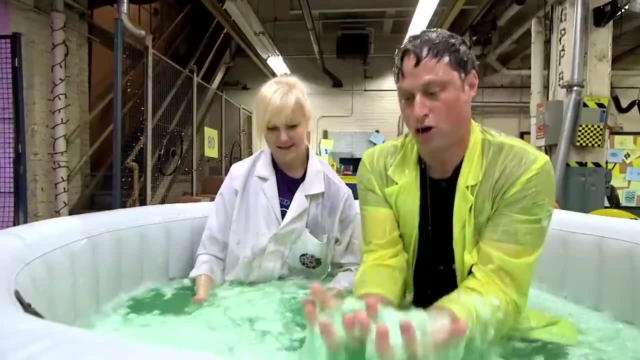 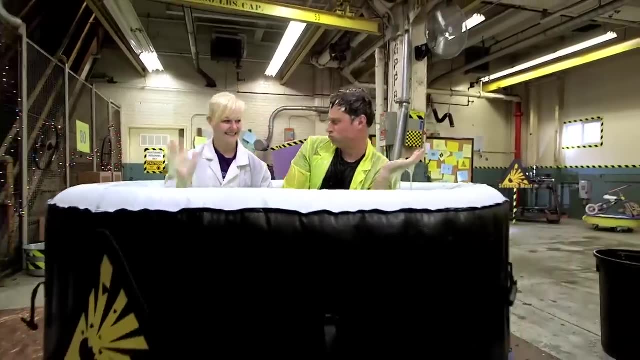 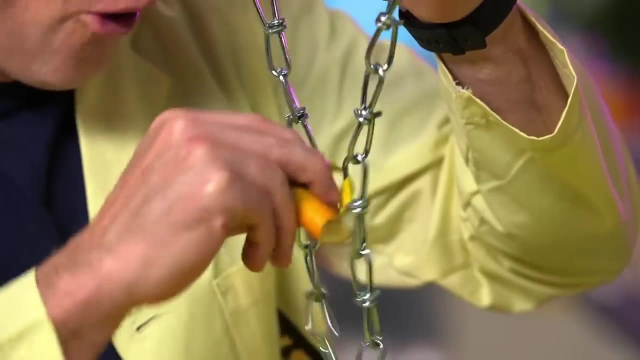 Well, there you go. Science Max, experiments at large Polymers. Slime, Yeah, High-fives Yeah. Slimey, high-five, Yeah. This episode is all about chemical reactions. Om nom, nom, nom, Om nom nom. 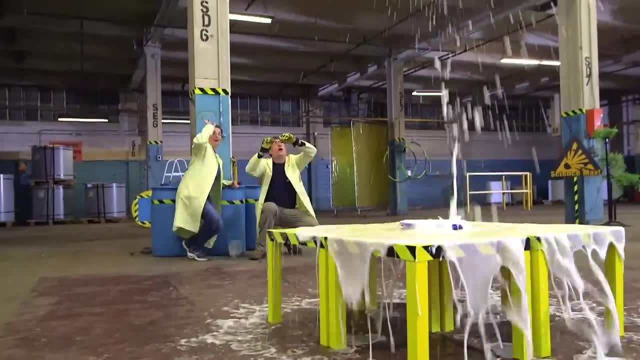 Om nom, nom, nom, Om nom nom. Delicious Reactions to make things fly, to make things glow, to make things pop and to make things fly. Ha ha ha, That worked. Wait, did I mention the flying? 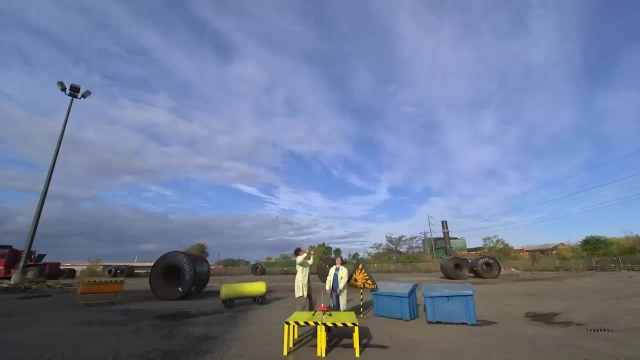 I'm sure I did, But I'm mentioning it again because it's awesome. All on this episode of Science Max Experiments at Large. Okay, Science Maximites prepare to hurtle through the cosmos. I am Captain Phil and today we're going to be building rockets on Science Max. 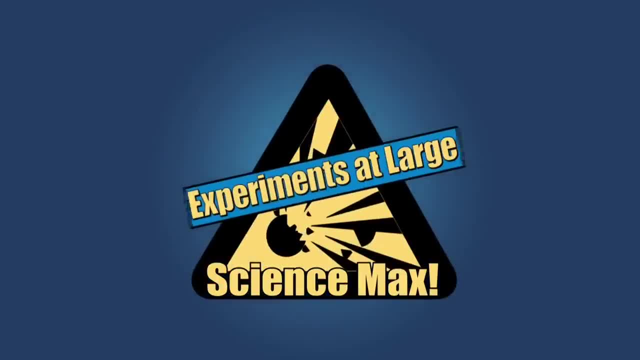 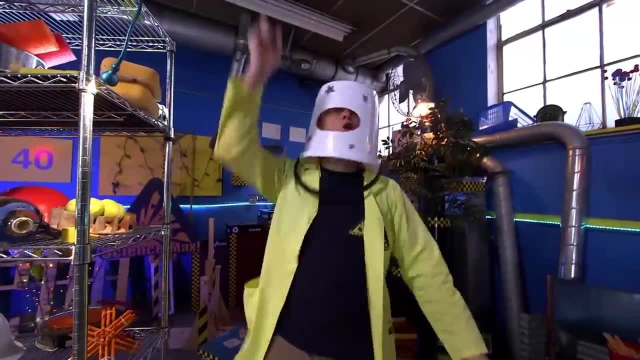 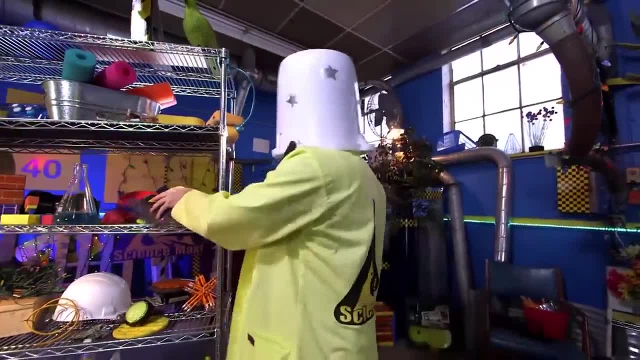 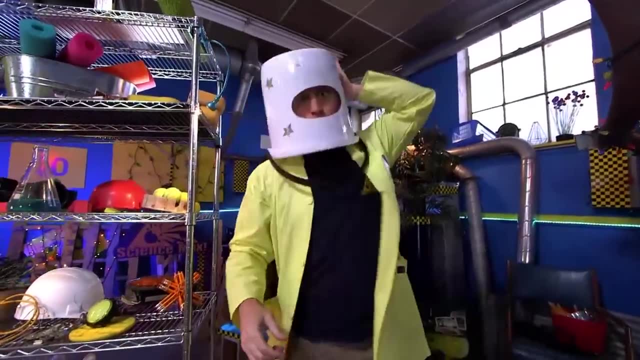 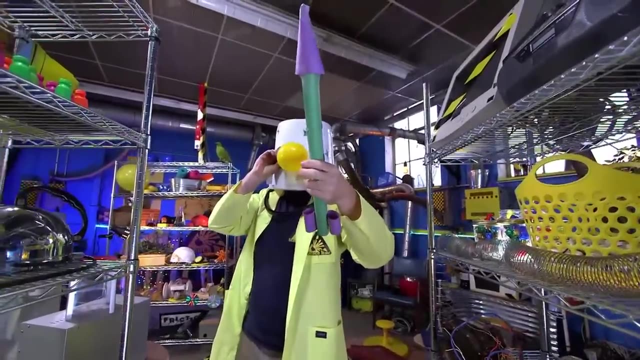 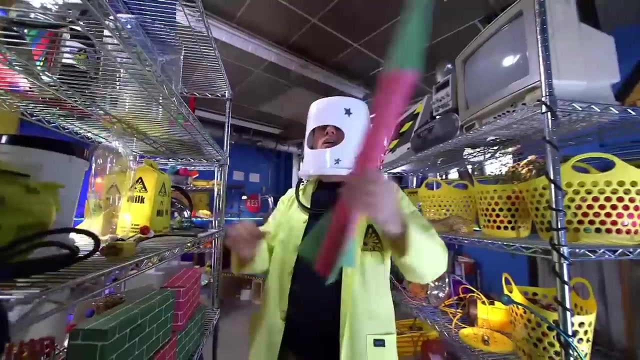 Powered up, Powered up, Powered up. So for this episode, we've built rockets before, like this one powered by air pressure And this one stomp rockets, which were also technically powered by air pressure- air pressure rocket. But today, Science Maximites, we are going to be building rockets powered by chemistry. 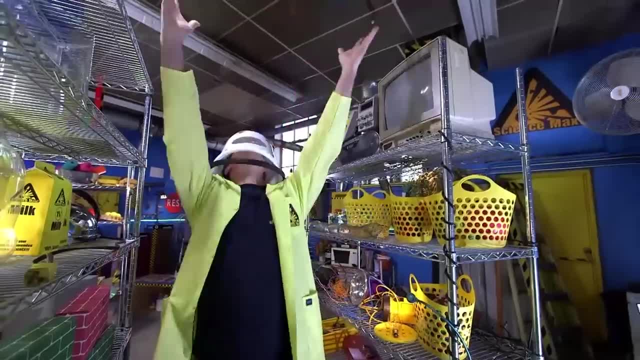 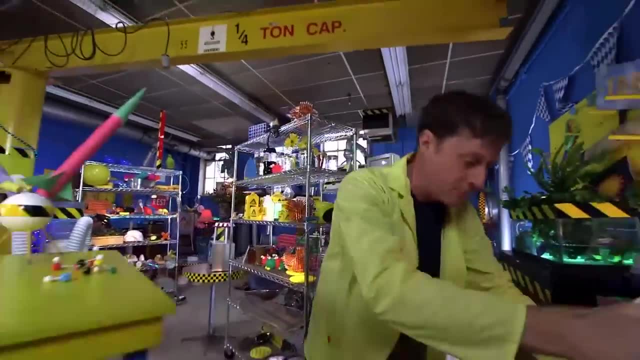 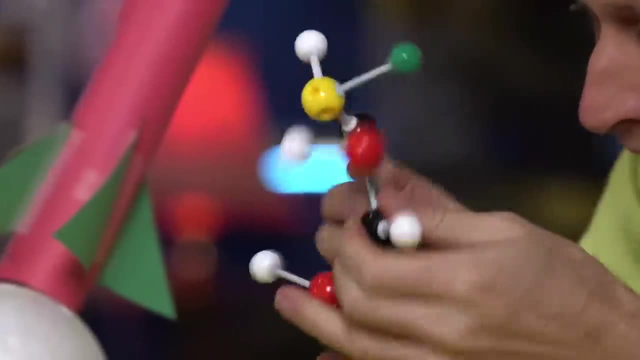 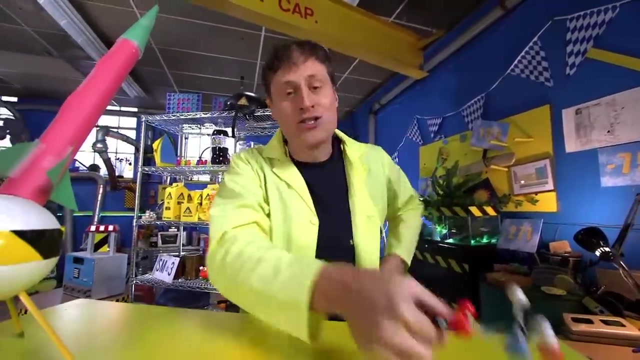 Chemical powered rockets away. Hmm, Okay, I promise it'll be more exciting than that, because today Science Maximizes. we are going to be looking at Chemistry. Chemistry is when two molecules combine to make another molecule Like magic whoo. So let's take a look at what we'll be powering our chemical rocket. 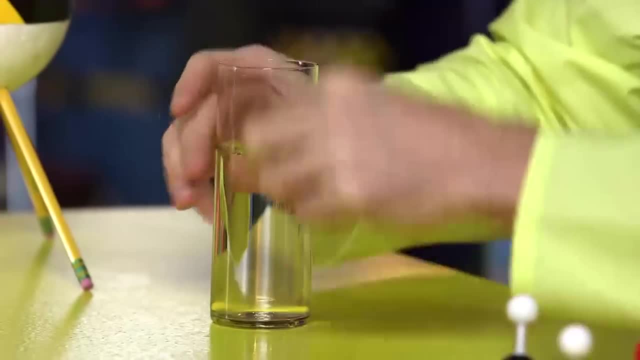 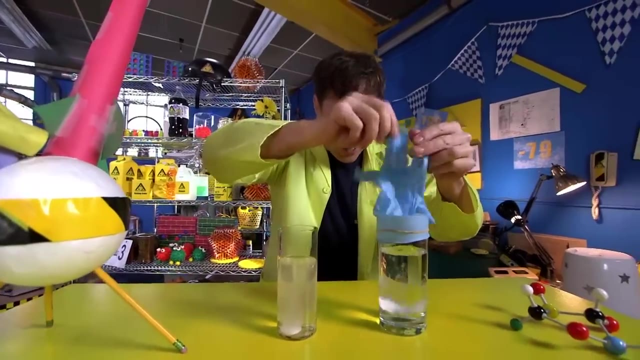 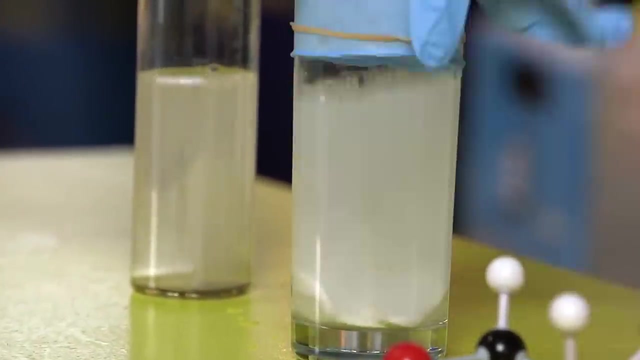 This. it's an ant acid tablet. when you put an ant acid tablet in water, it makes little bubbles of carbon dioxide gas. this happens because of a reaction between two kinds of molecules called Acids and bases like vinegar and baking soda, But all contained in a small package that won't start working until you put it in water. 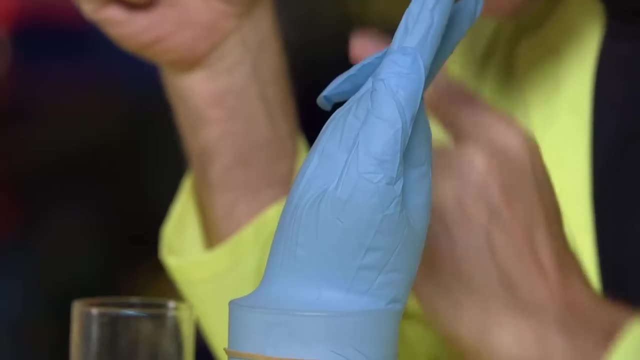 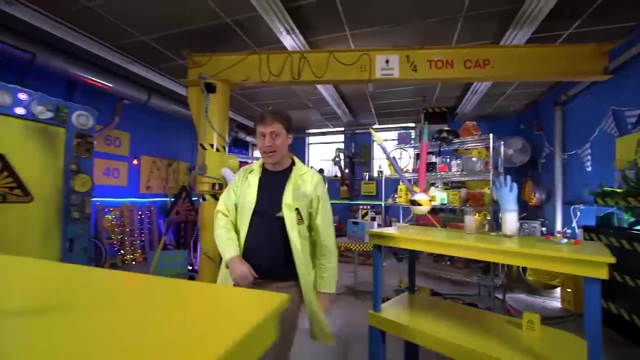 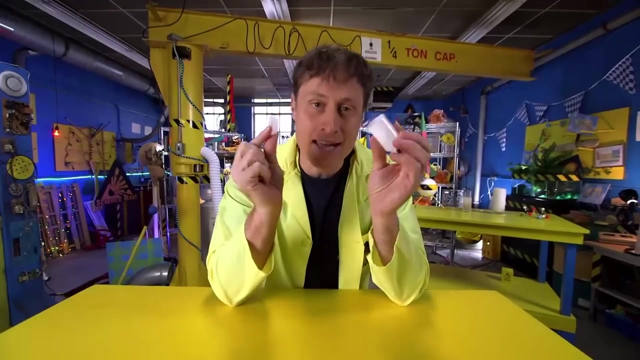 If we contain the reaction, the carbon dioxide gas builds up and creates pressure. High-five for science, All right. so let's look at our chemical powered rocket. What you need is one of these. This is a. This is a film canister. and ask your parents what that actually means, because they're not used for holding film anymore. 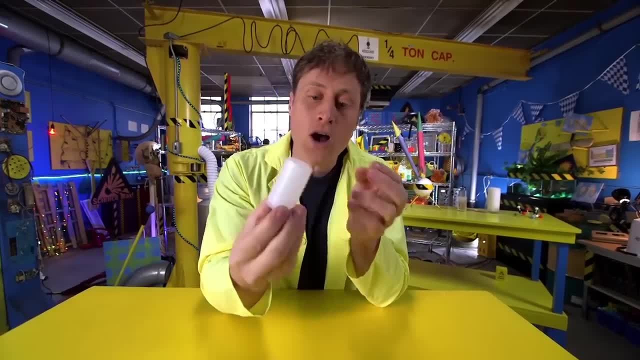 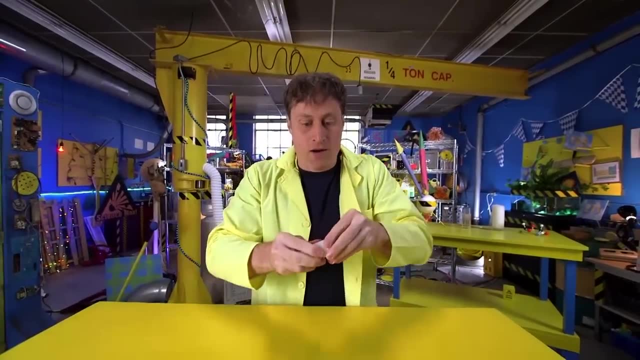 You can get these at craft stores, though, to hold paint or little things, but really all you need is a plastic container with a good lid that snaps on, nice and tight and Keeps the air in, and then, of course, what you need are your ant acid tablets and a little bit of water. 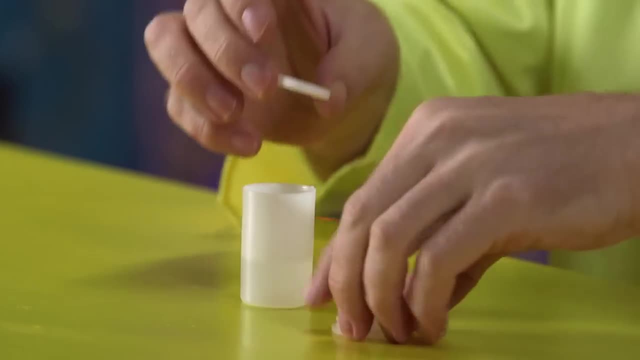 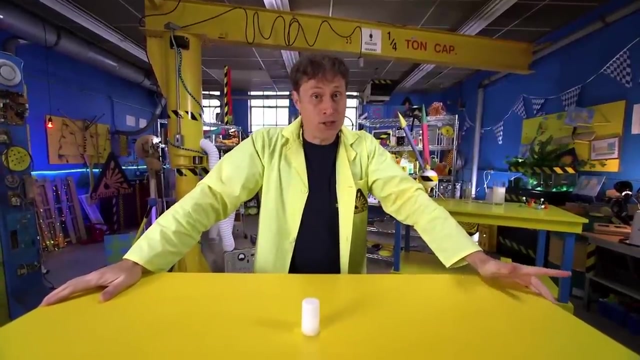 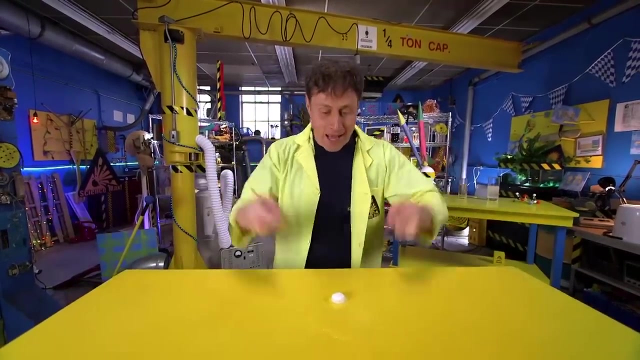 so pour in some water and then put in your ant acid tablet and Snap the lid on, flip it over And wait for the carbon dioxide gas to build up, which will build up pressure, which will Launch your rocket. Haha. So there you go, a chemical powered rocket. Come on, Let's max it out. So first I 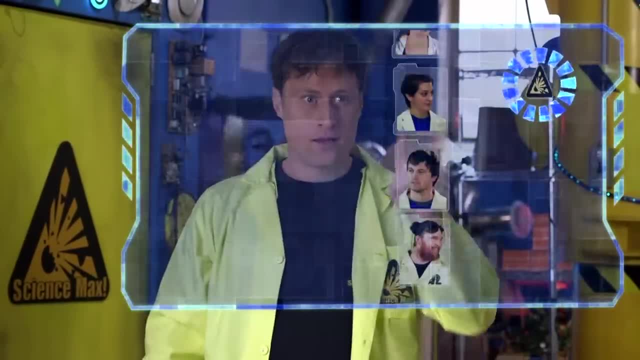 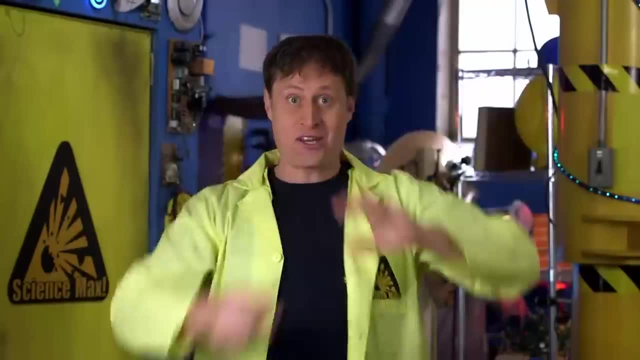 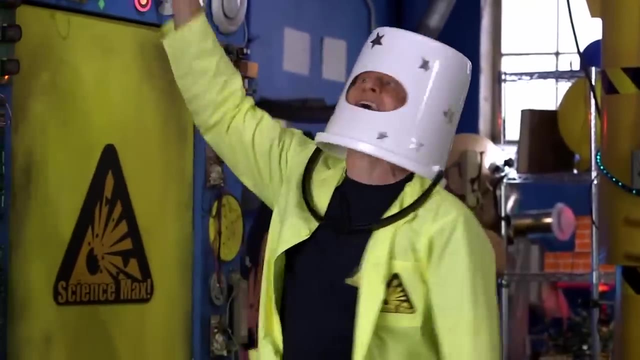 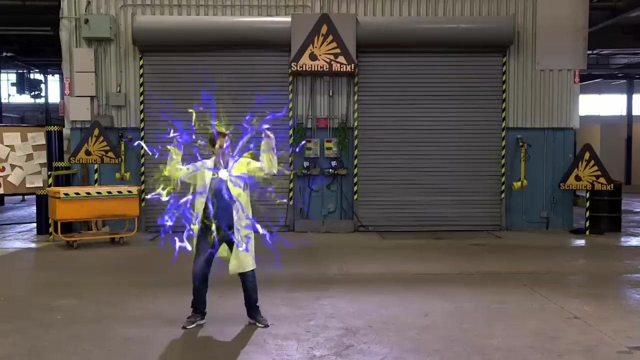 Need an expert to help me? Oh, Lisa from logics Academy, of course. logics Academy people have helped me launch all the rockets on science max. This is gonna be great. Oh, I'm gonna get my helmet first. Let's watch some rockets. Whoa wow, it's really dark in this room. I can't see anything. 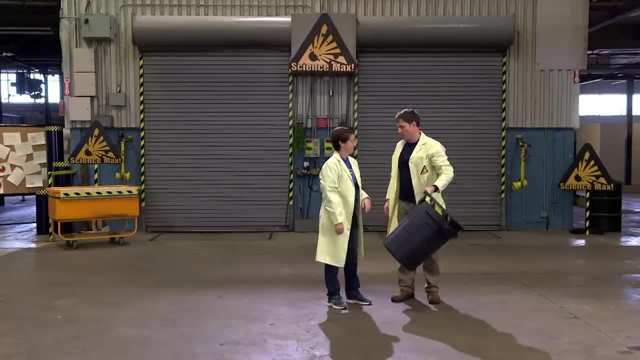 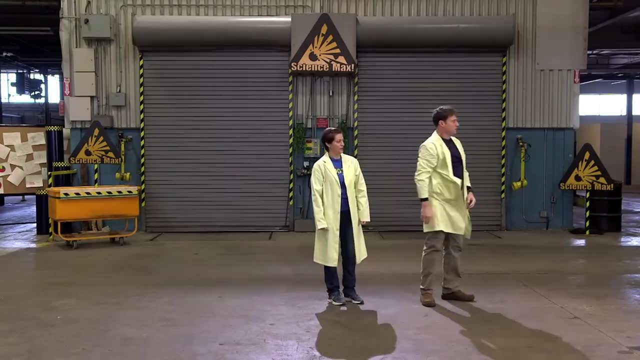 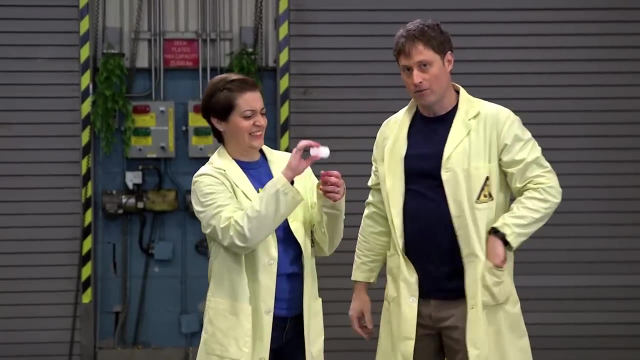 Where did this come from? I Guess the portals malfunctioning. Hey, Lisa from logics Academy, great to have you here. Great to be here. Let's put this over there. We are here to max out the chemistry rocket. What is that? It's just a small plastic container, but when we put an ant acid tablet in there and some water, 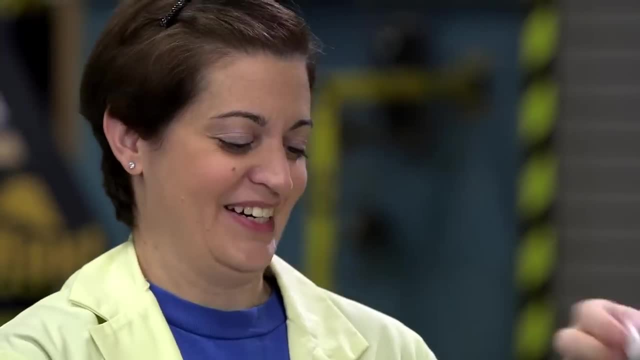 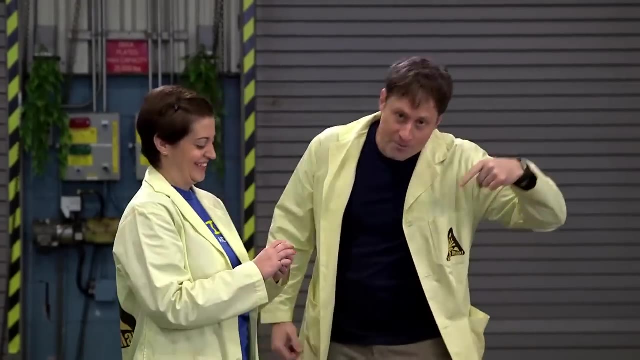 Ah, We get a chemical reaction. We've got a chemical reaction, And so that's what creates the pressure, and then that pops the lid off and we get a little rocket. Oh, but now we're going to max it out, get a bigger container. Oh wait what? 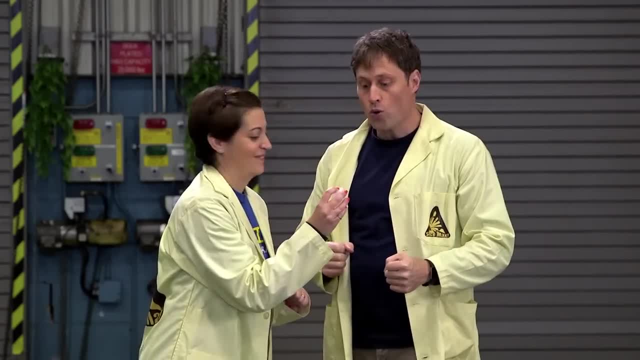 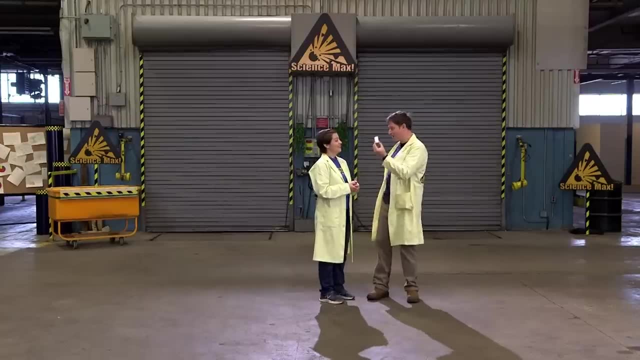 How about if, If we launch a whole bunch of them? Oh, so we just get a lot of the small one and we launch them all at the same time, Exactly, Okay, great. So we just need a whole bunch of these and a whole bunch of- and a whole bunch of science- ant acid. 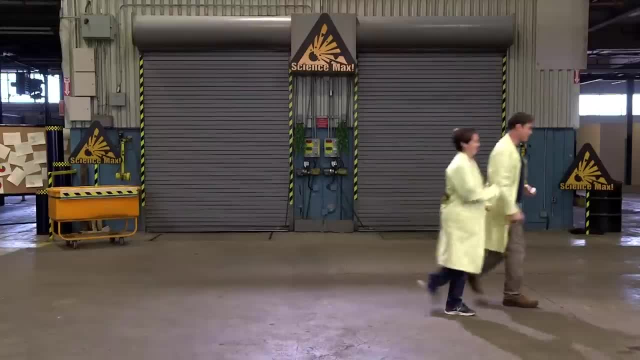 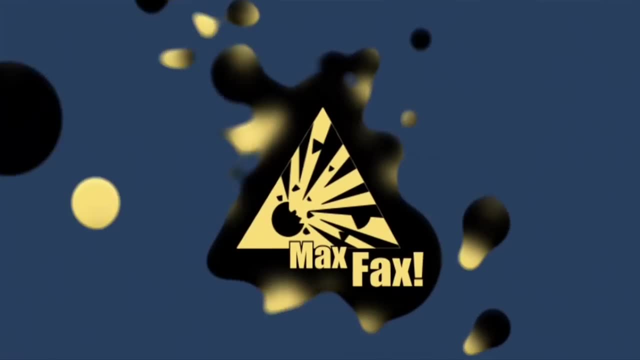 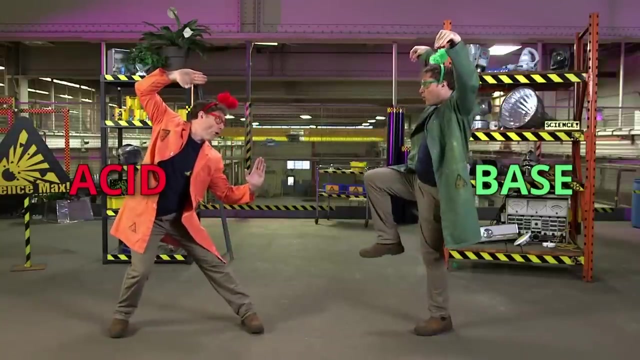 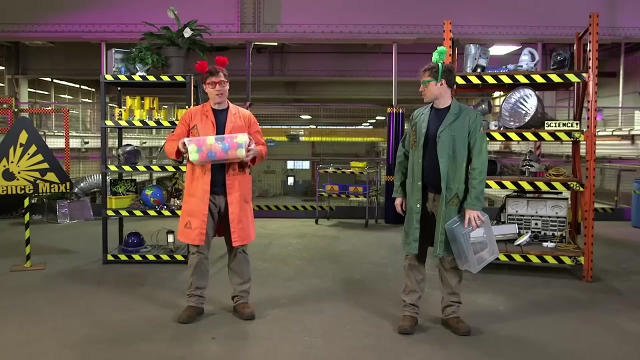 Yeah, well, that's okay, I get them both in bulk. Come on, let's go put it together. I'm an acid and I'm a base and we are enemies. Oh well, we're not really Enemies. Yeah, that's true. It's all about how we react chemically. You see, as an acid, I really want to give protons away. 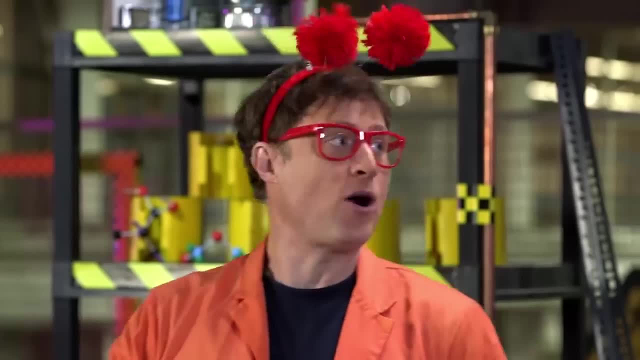 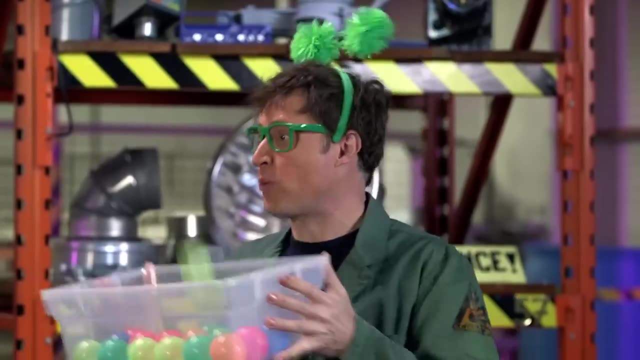 Protons: who needs your protons? get your protons here. protons: I got more than I want, I don't need them anymore. and bases: We need protons. We'll do anything to get them. protons, You can protons away, I'll take some. I'll take some protons. 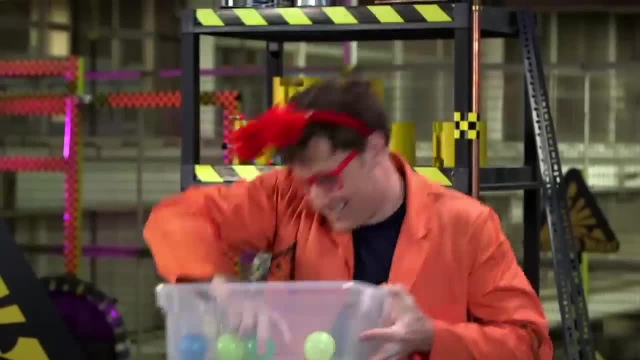 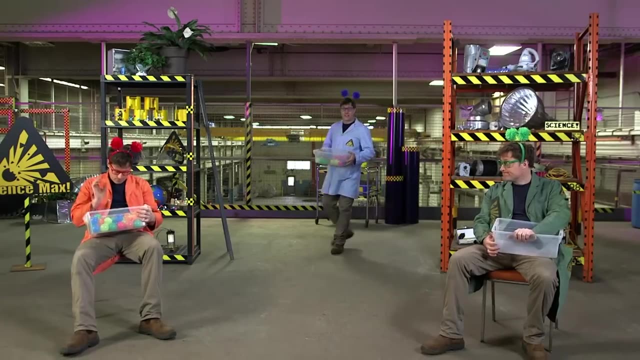 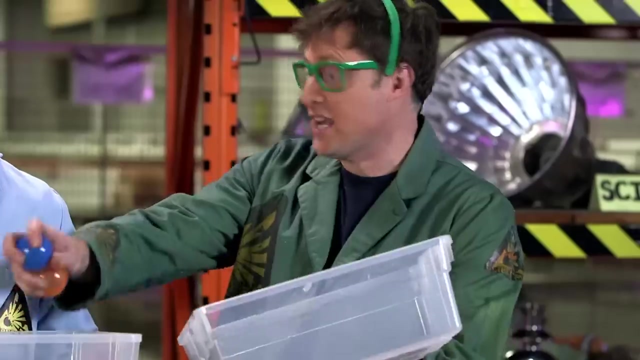 Do you think that when you get these two together you'd have some pretty great chemistry? but the truth is, when they're together, They often don't react. That is until water gets involved. once you have water, acids and bases react. Here, take some protons, all your base, up along to us. 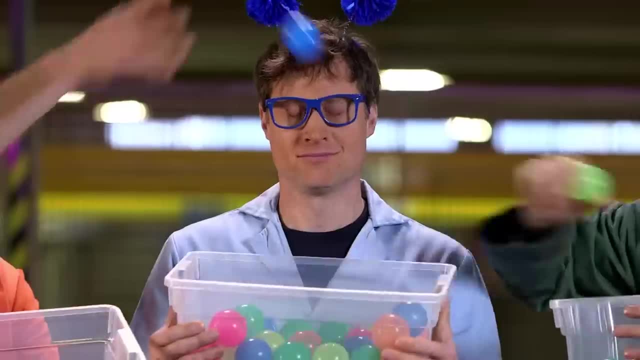 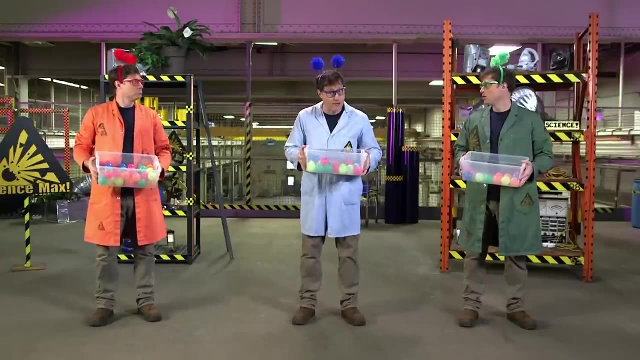 Here. water is a solvent Allowing the chemical reactions to take place. Depending on the strength of the acids and bases, That reaction can be mild. Would you like a proton? Oh, no, really, I could please. please take it. Well, Thank you. 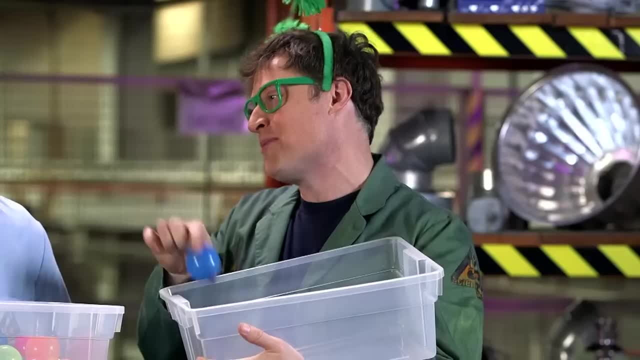 That's very generous. have another, oh, perhaps. Maybe I wish I had more protons, not the olun. Maybe I wish I had another potassium atom. Here's one, Maybe just one. But if the acids and bases are strong, the chemical reaction can be really extreme. 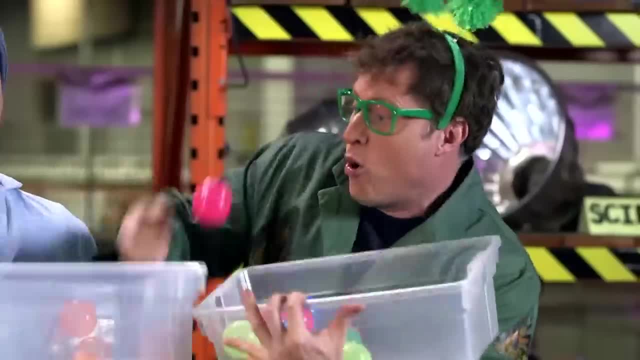 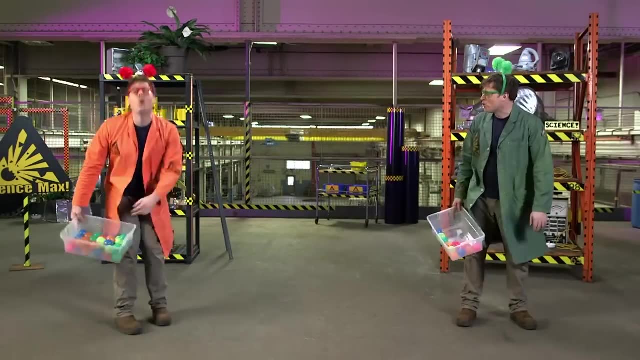 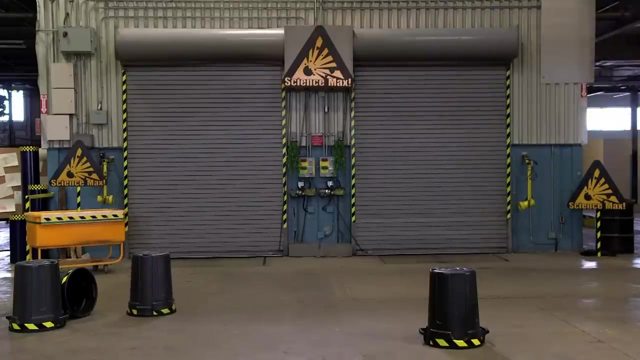 This is what's going on in the antacid tablet And why, without water, nothing happens. Oh, water, Come on. What'd you do? And that's the last one. Lisa and I are maxing out our chemical-powered rocket. 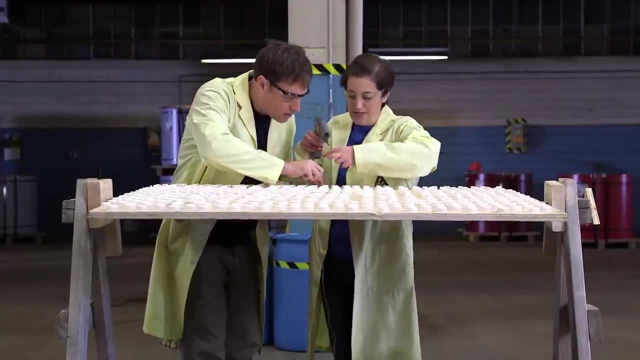 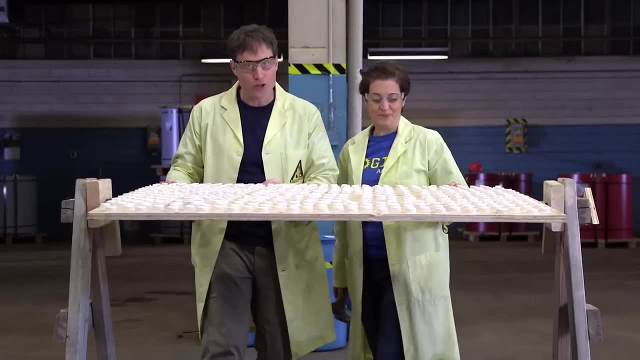 not by making it bigger, but by making more of them. How many more? 400 caps all glued down, 400 antacid tablets, or part of all glued down, and they're glued on this fancy-pantsy spinning surface. 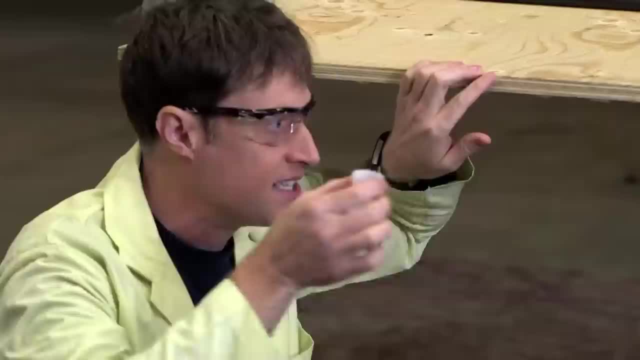 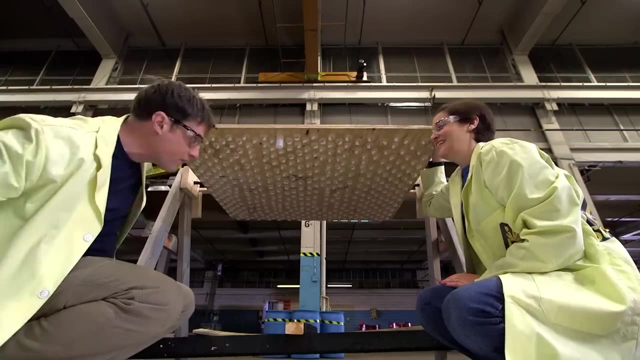 So we rotate this part upside down. We fill each container with a little water and snap it on underneath. This way, the antacid tablet and the water don't mix until we flip it back over. It also allows us time to snap them all on. 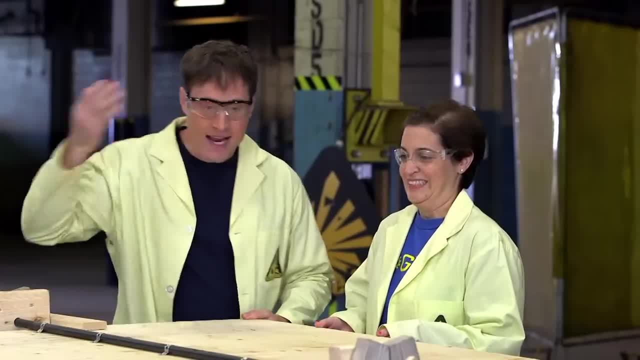 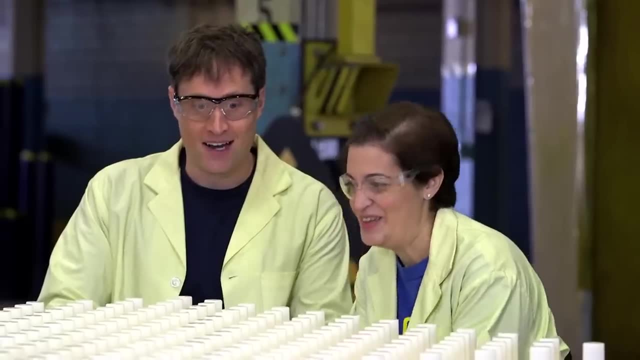 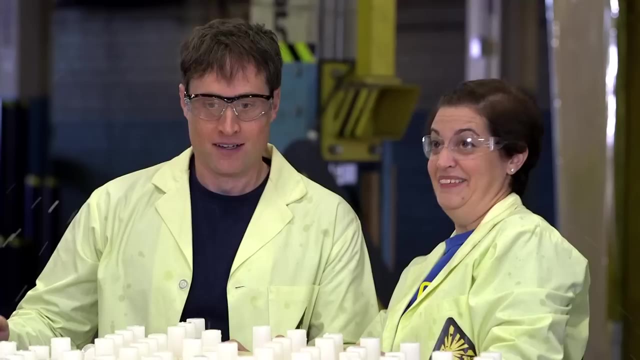 Okay, ready, Ready, All right. 400 containers. Here we go, Let's do it. Once we flip the board back over, the reaction started taking place, building up carbon dioxide gas and increasing the pressure until Whoa, Whoa. 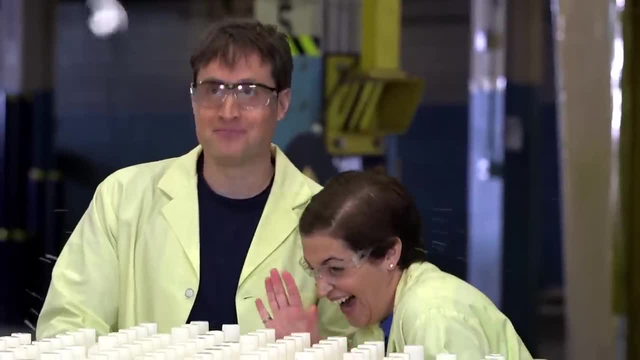 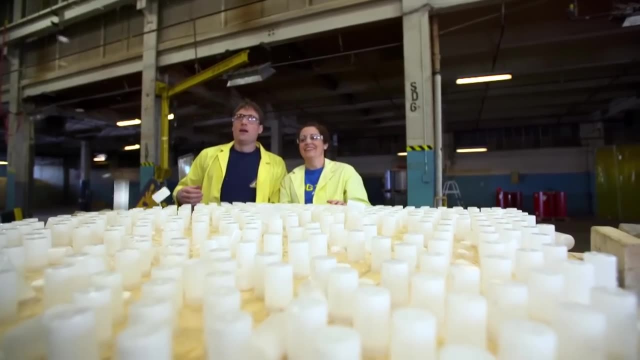 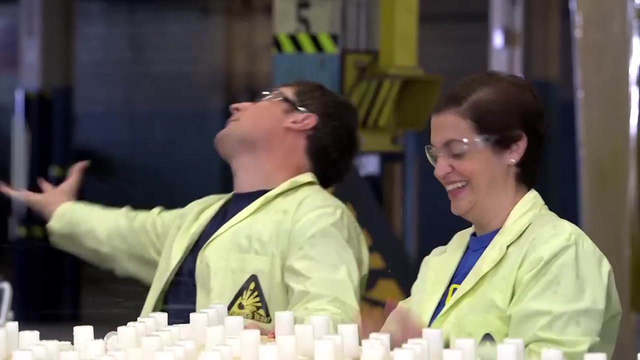 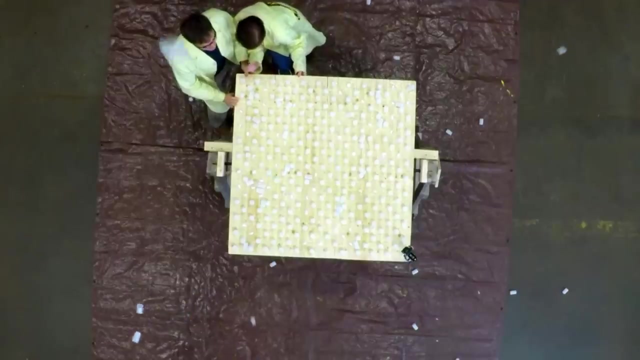 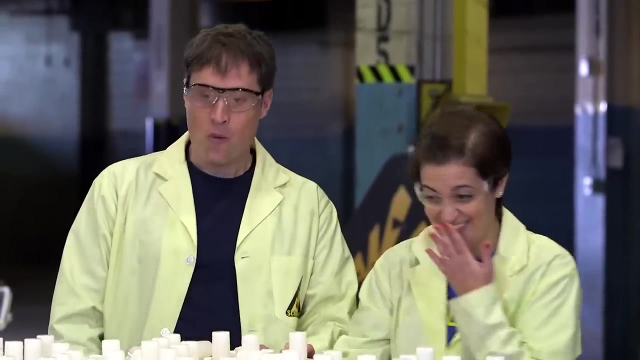 Oh yeah, Oh yeah, Oh, my goodness, It's good luck if you catch one. Whoa, Whoa, Whoa. Wow, that one looks really hot. Oh Awesome, That totally was great. Wow, Okay, so high-fives on that. 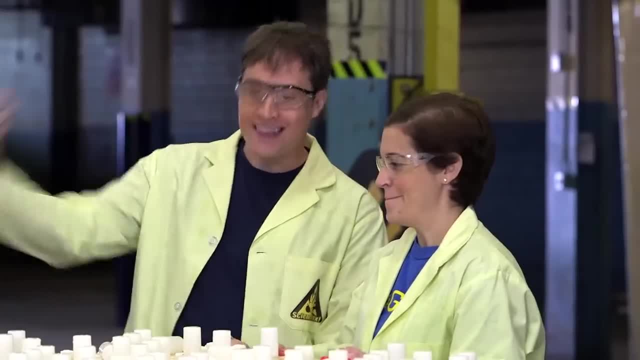 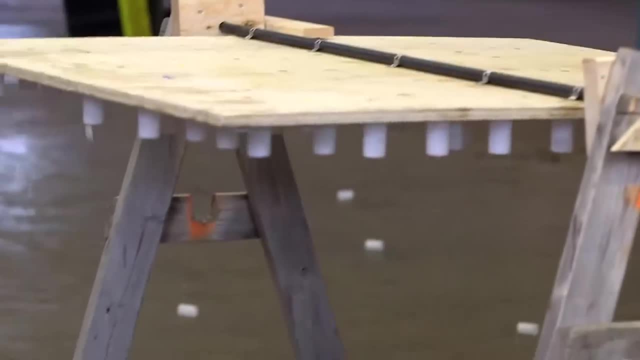 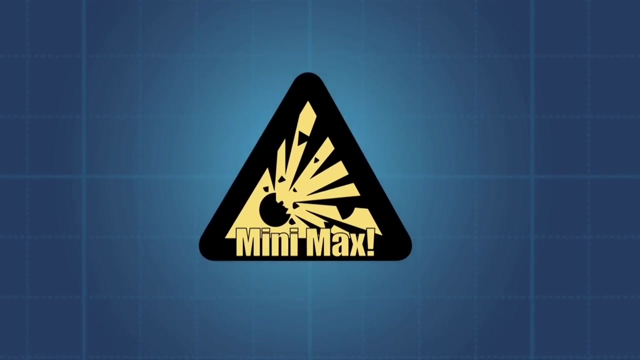 That worked spectacularly. That was awesome. So we've done this. Let's go bigger. Let's go bigger. Okay, Let's do it. This is a balloon and this is an orange, And together a chemical reaction happens. 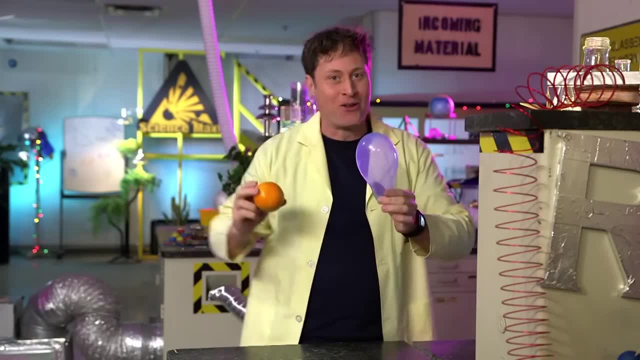 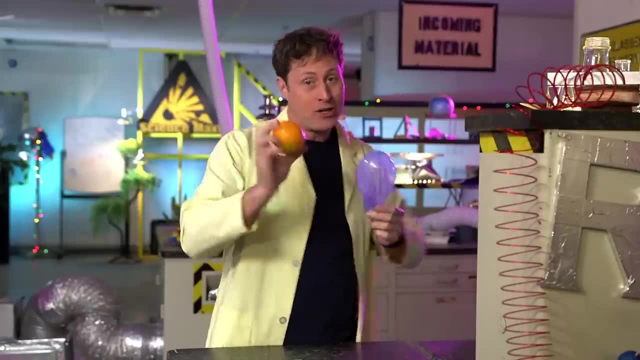 How'd you go in there for a minute, didn't I? No, No, All right. Well, you can actually do a chemical reaction between a balloon and an orange. You see, balloons are made of latex, which is a kind of polymer. 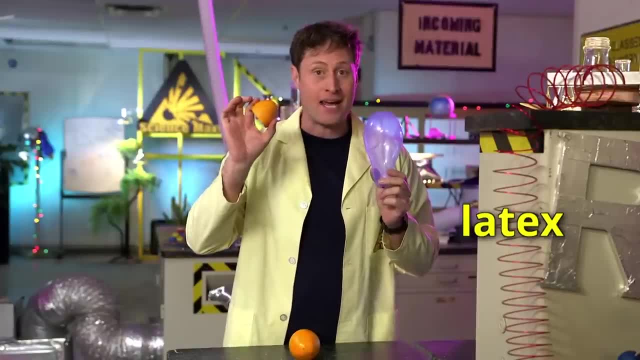 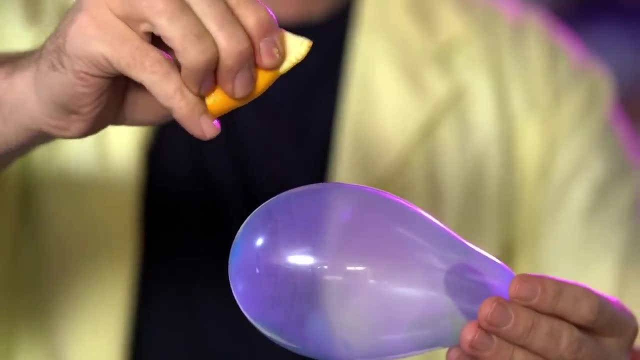 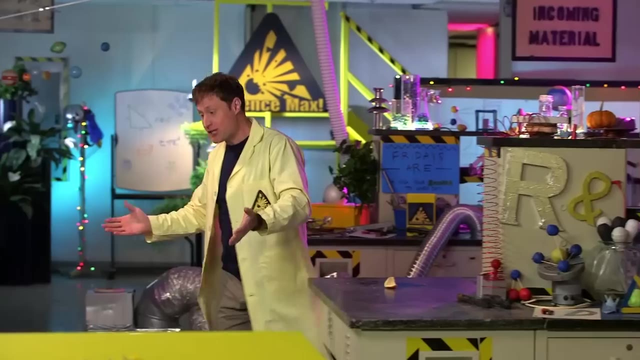 that's very, very stretchy, And orange peels contain a chemical called limonene. Limonene breaks down latex. So we have three questions. The first is: why does this happen? Well, like I said, it's all chemistry. 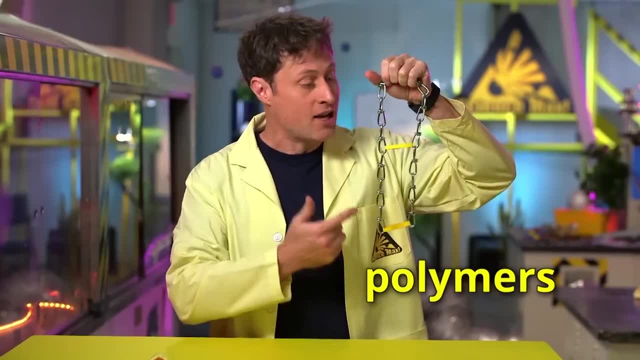 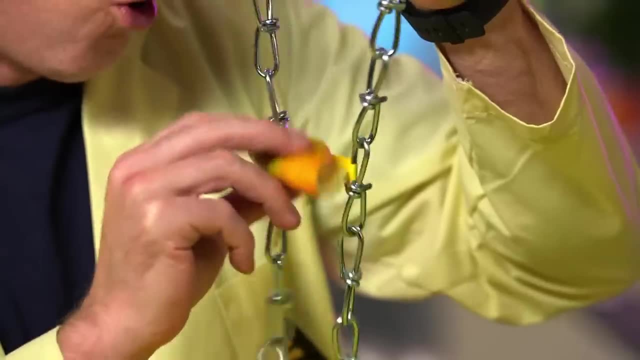 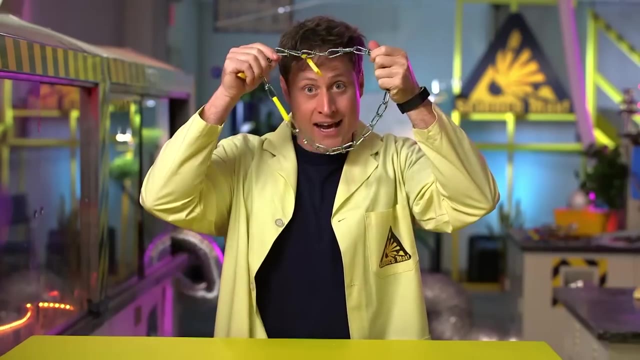 You see, balloons are made of polymers, chains of molecules held together by chemical bonds. A limonene molecule attacks those bonds- Om nom nom nom, Om nom nom nom, Delicious- And breaks it. That separates the polymers and that pops the balloon. 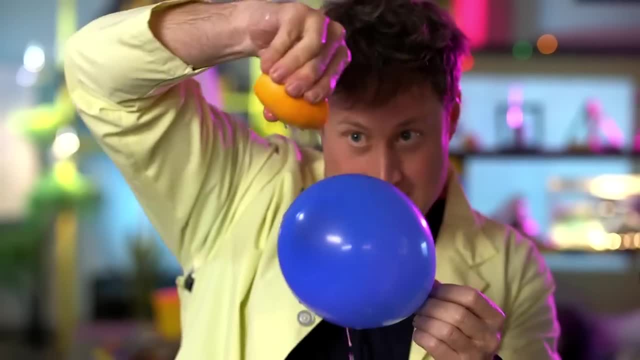 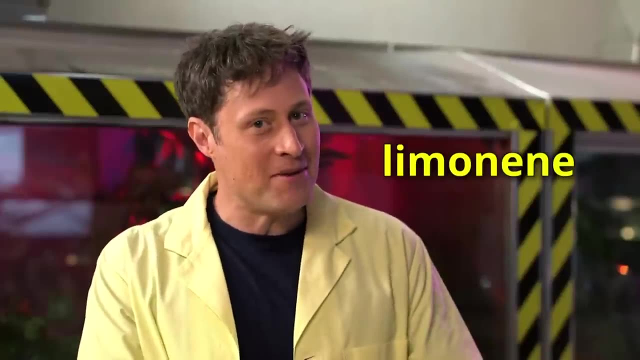 But remember, it only works with natural latex, So make sure you're using natural latex balloons. Second question: why do they call it limonene when it's in orange peels? I mean, yes, it's in lime peels. 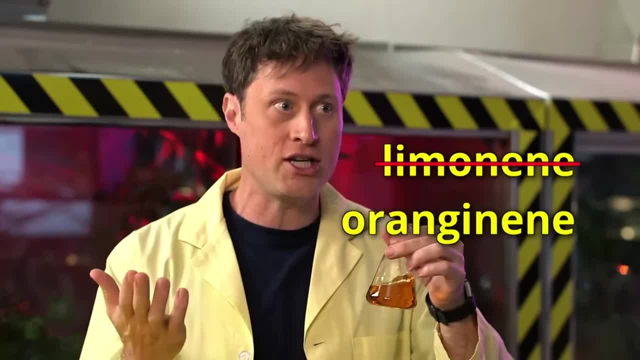 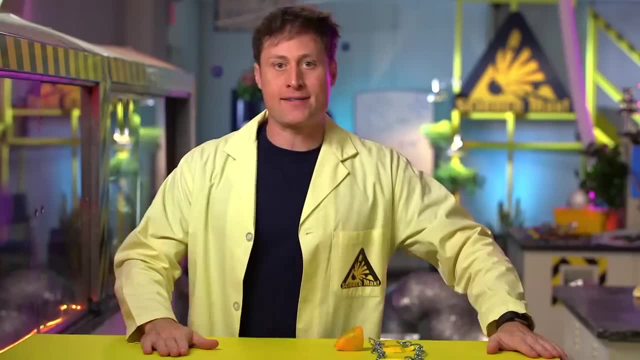 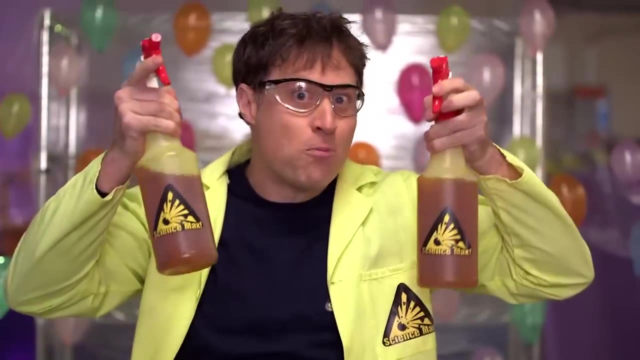 and lemon peels, but the chemical itself smells like oranges. They should call it orangenine or citrus frutenide oranyway. Should we max it out? Of course, we should Come on 200 balloons versus two bottles of limonene. 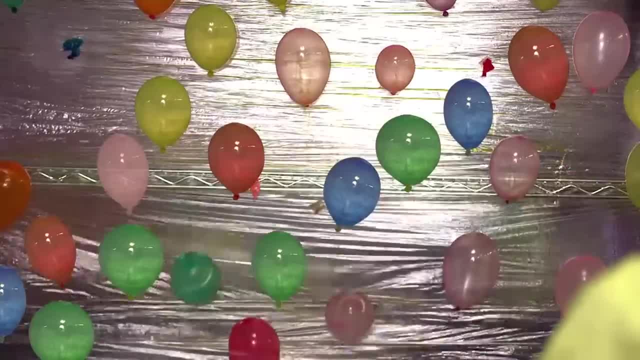 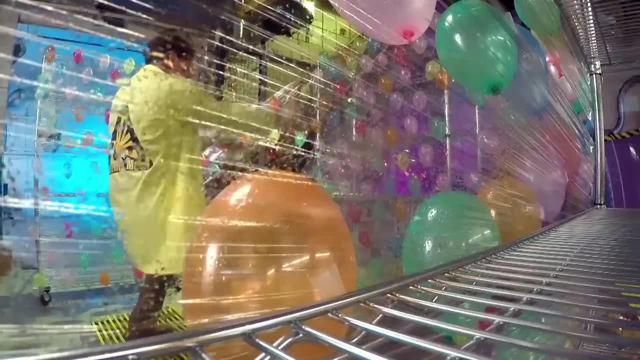 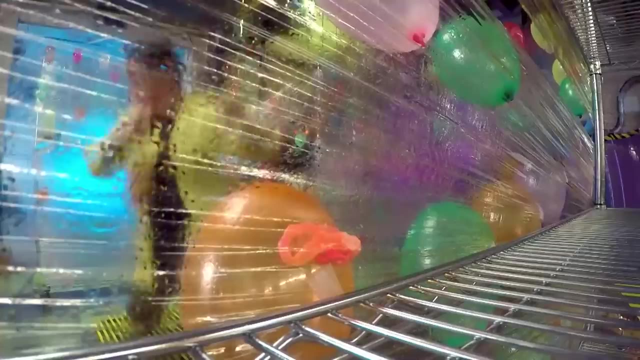 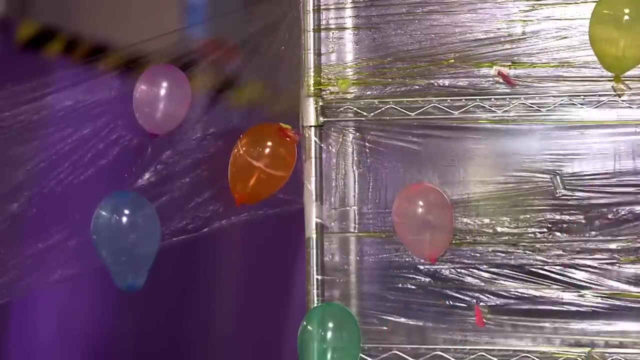 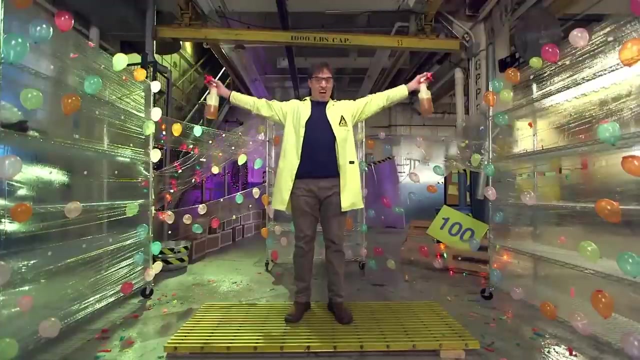 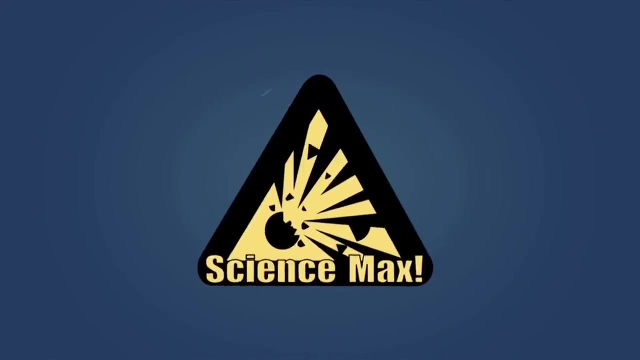 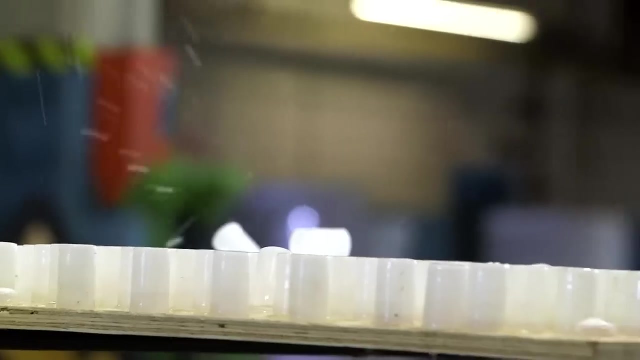 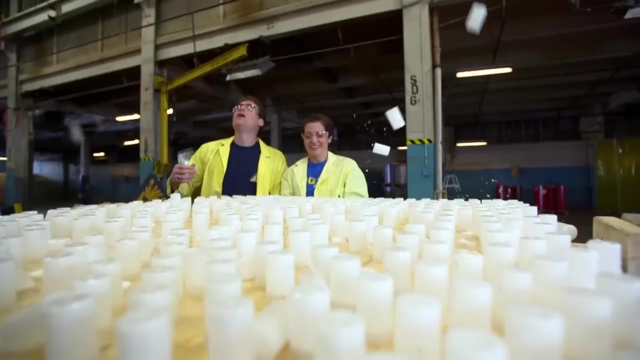 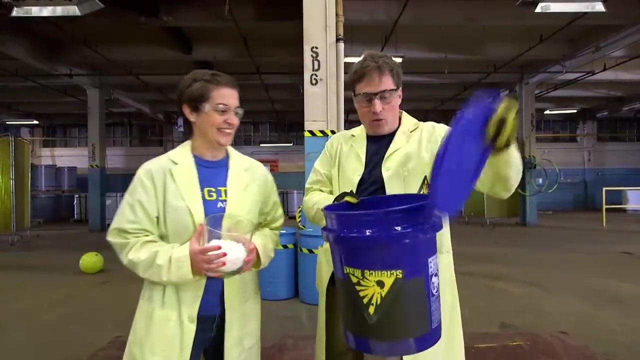 Ready Go Science. Our first attempt to max out our chemical rocket was 400 plastic containers. Oh yeah, That worked well, but now it's time to make the container larger. Whoa, Giant, maxed out chemistry rocket canister. I have a big plastic container with a 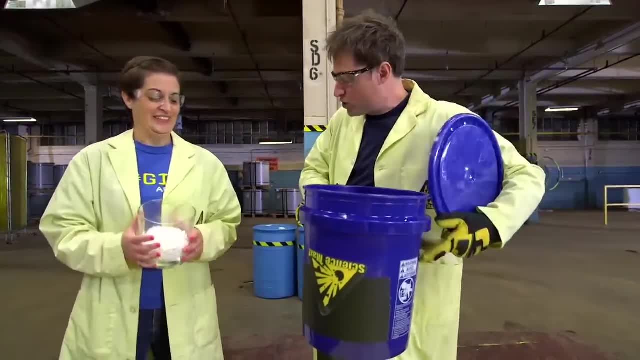 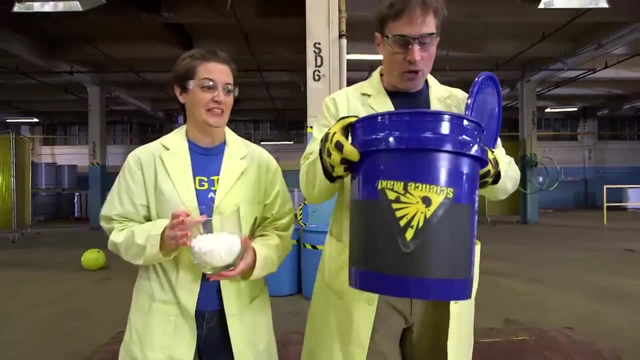 groovy lid that sits there on airtight, which is great, And I have a giant jar of antacid. It was like 60 antacid tablets or something At least. This works exactly the same as our smaller containers. We dump the antacid in, seal the lid airtight. 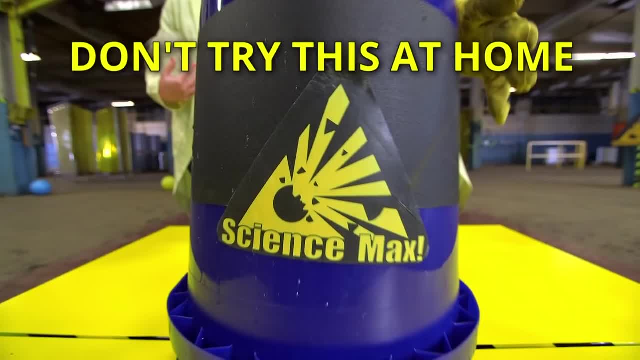 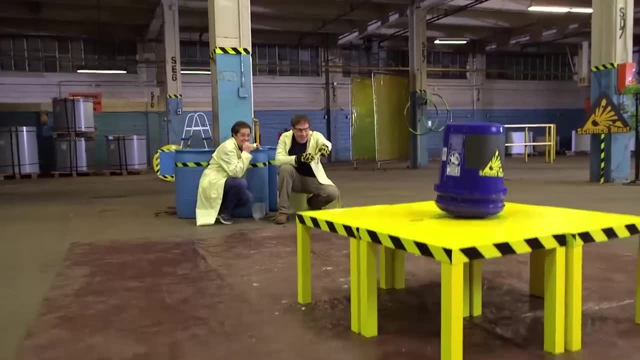 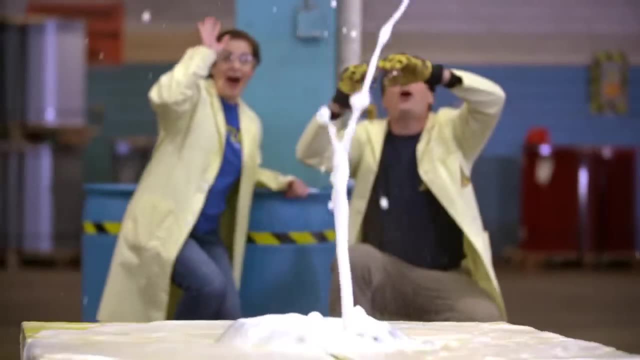 then flip it over, And now would be a good time to mention that we made this at home. Okay, Oh, it's not going to take long. All right, So that was the canister version. Now we need the pop bottle version. 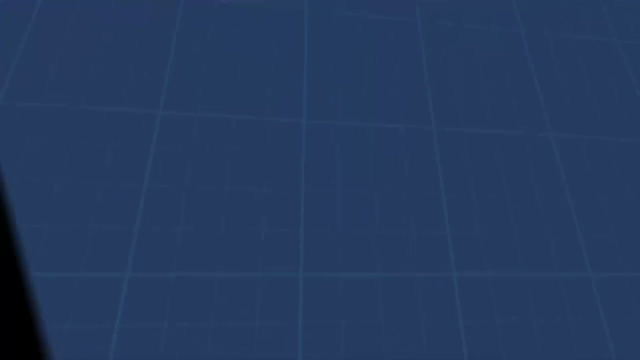 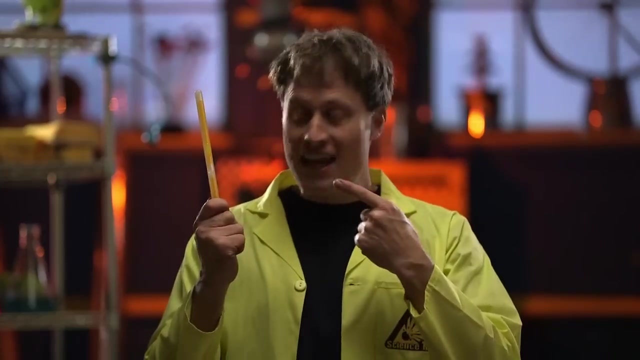 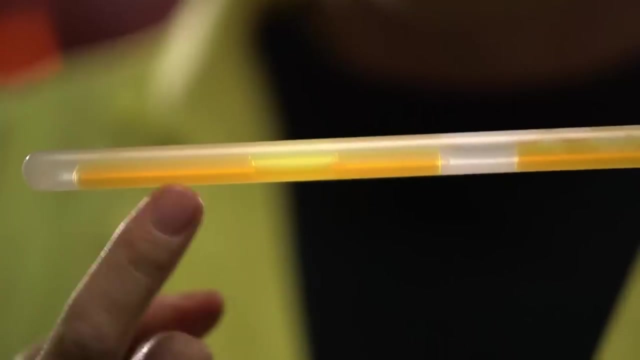 The rocket version. Yes, Okay, let's go make that. Let's do it. This is a light stick. It creates light using a chemical reaction. There's a liquid chemical inside and also a glass container that holds another chemical When you bend the light stick. 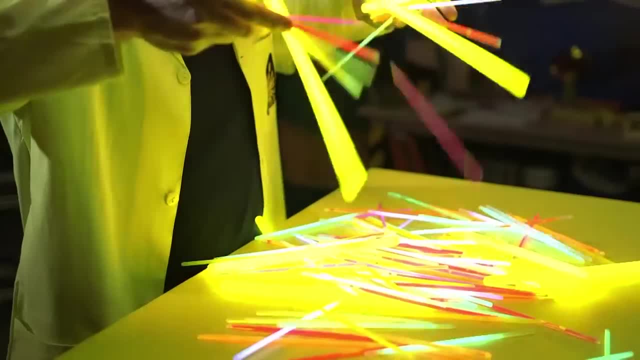 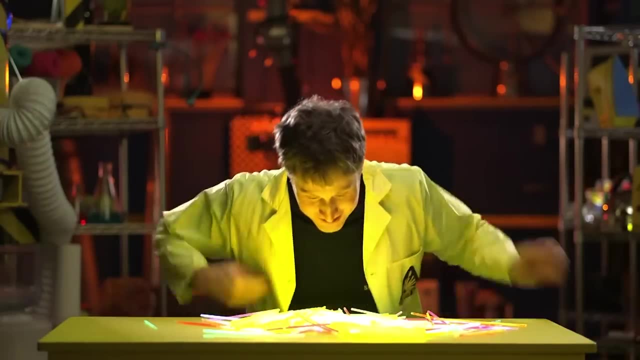 you break open the container and the two chemicals mix, creating light. There you go, Light sticks, Chemical reaction And yes, of course we're going to max it out. This is a whole bunch of the two chemicals in a light stick. 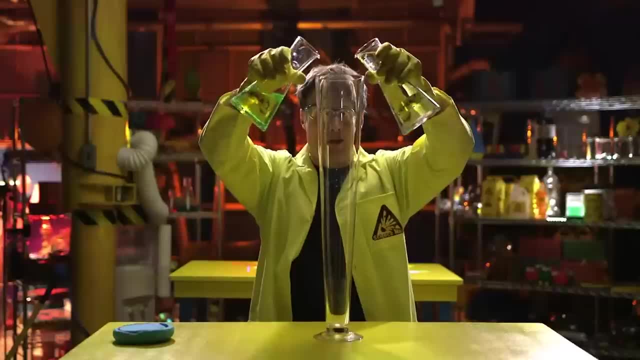 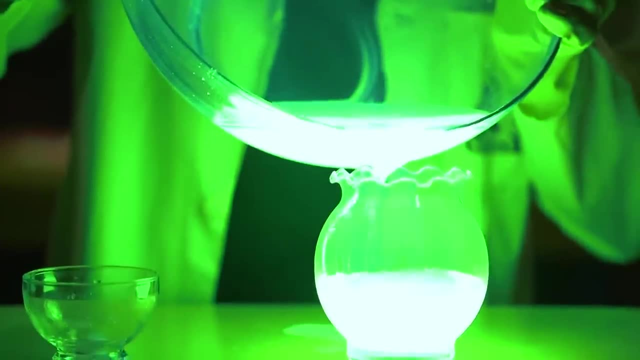 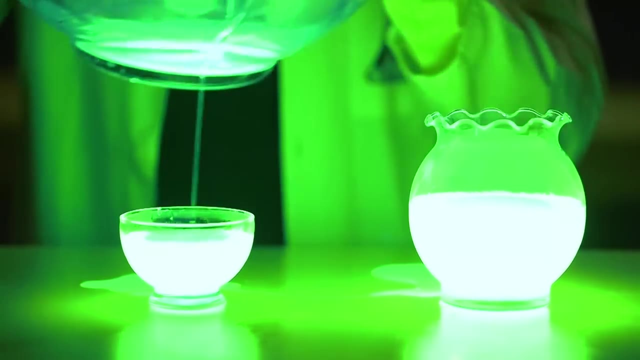 Let's max it out. So how does a chemical reaction produce light? Well, a lot of chemical reactions produce energy. You might think of a chemical reaction producing heat. Well, heat is a kind of energy. This chemical reaction also produces energy. 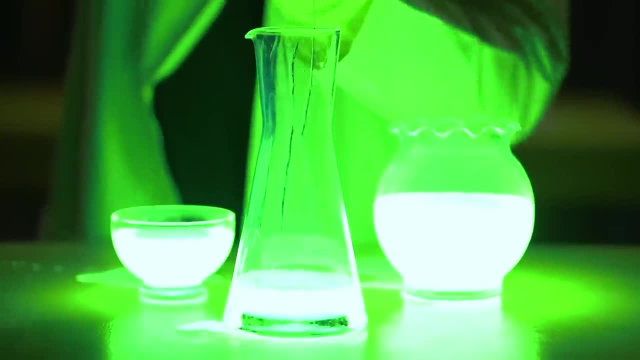 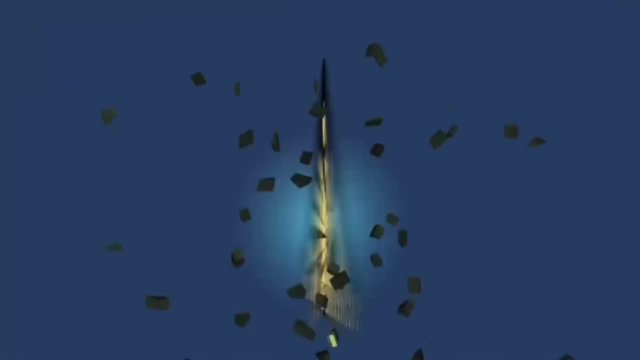 just energy in the form of light. It's just a different kind of energy. Whoa Maxed out light stick And now for a Science Max quiz: Chemical change or not? What's a chemical change? Well, let's demonstrate. 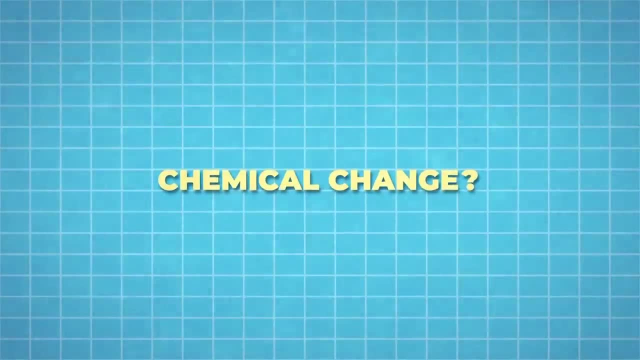 Look at this: It's a happy little molecule of iron. And here's another molecule of oxygen. If they were to have a chemical change, they would react and form different molecules. Look, It's a molecule of rust. Rust is a different chemical. 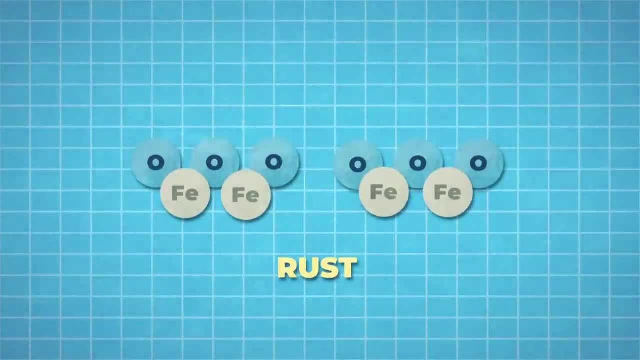 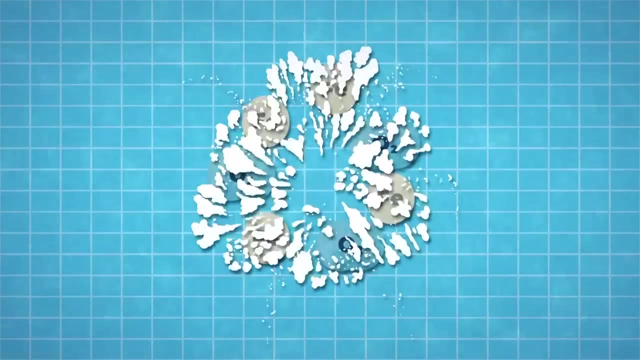 than either iron, or iron Or oxygen. It's a chemical change. Now, if these molecules mixed and did not change, then it's not a chemical change, It's a physical change. Sometimes it's hard to tell if it's a chemical change. 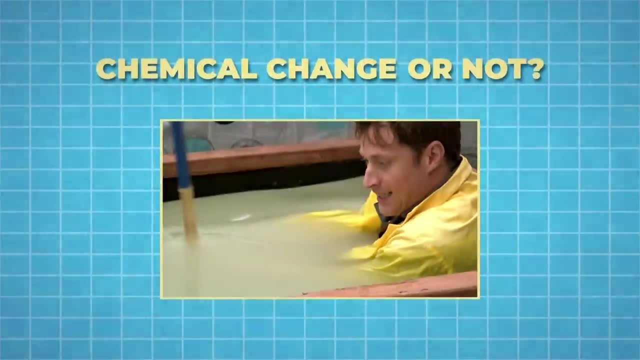 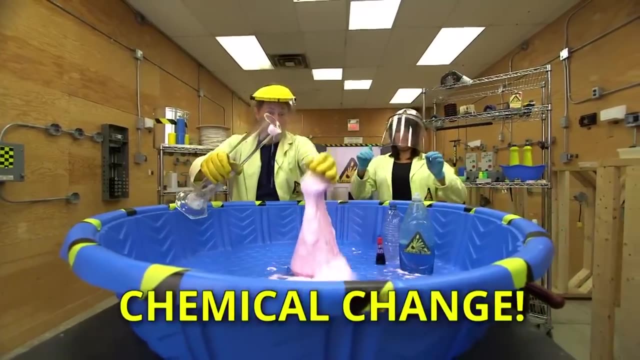 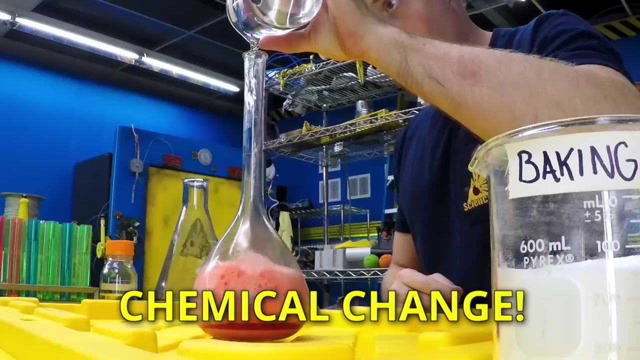 just by looking. But asking what kind of change it is leads to good science. So let's look at some examples: Vinegar and baking soda. Is it a chemical change? Yes, Vinegar and baking soda react to form different chemicals. Sodium acetate- that's the white stuff that's left over. 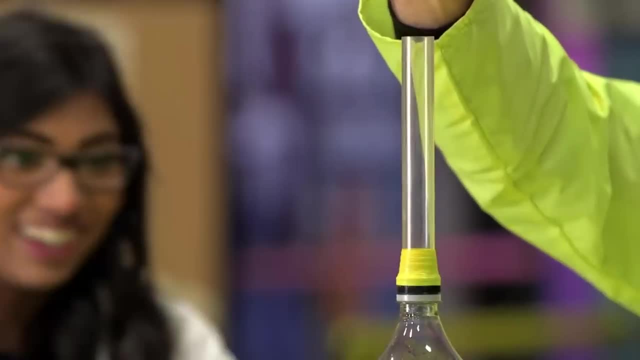 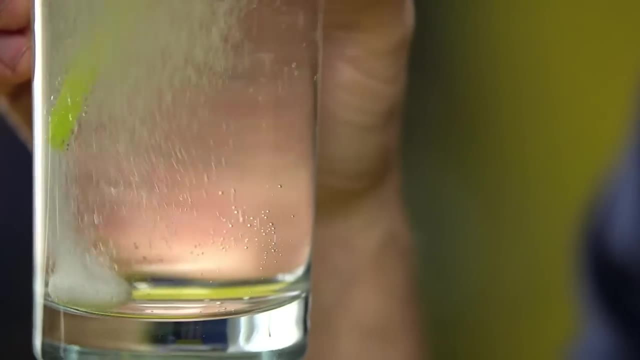 is a chemical change. How about a nucleation fountain with diet cola and mints? A lot of people think that's a chemical change, but it's not. The mints cause carbonation, the bubbles to escape faster, But in the end you still have cola and mints. 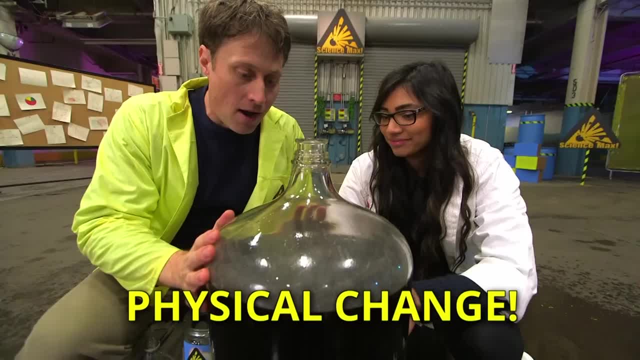 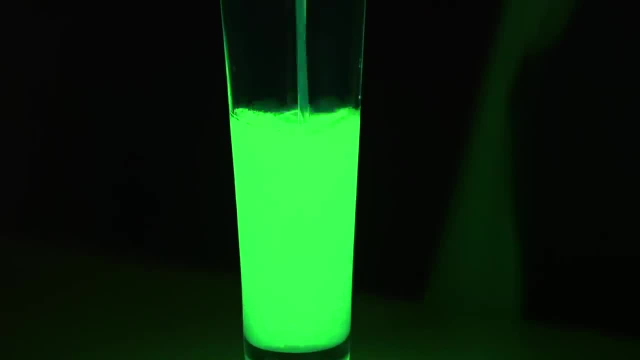 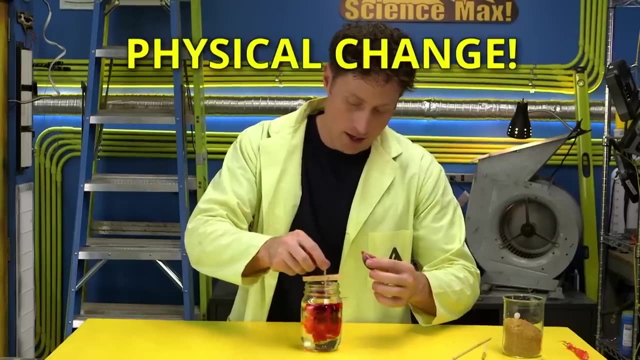 No new chemicals And without the carbonation nothing happens. So it's a physical change. Take a guess at this one: Glow stick chemicals. Well, producing light or heat is a chemical change. How about mixing sugar and water to make a sugar pop? 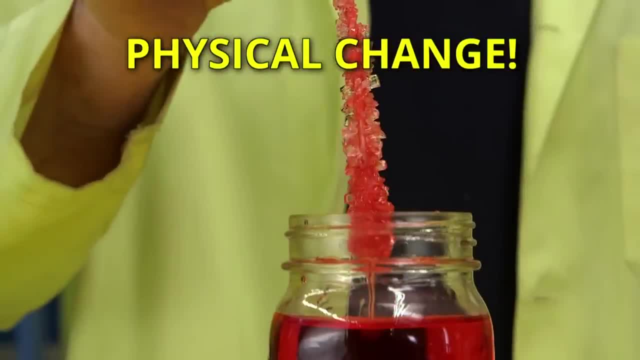 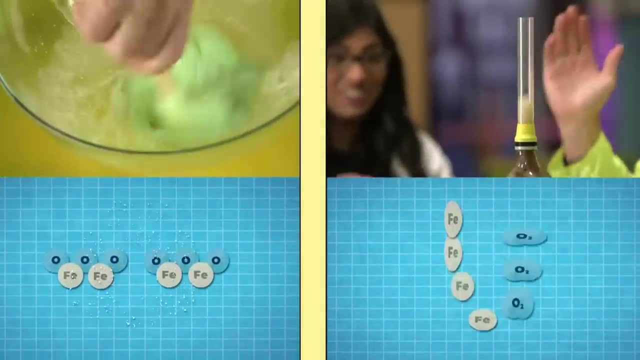 That's a physical change. You start with sugar and water, you mix them and when you have a sugar pop, what chemicals are you left with? Well, sugar and water, So no chemical change. It can be hard to tell sometimes. 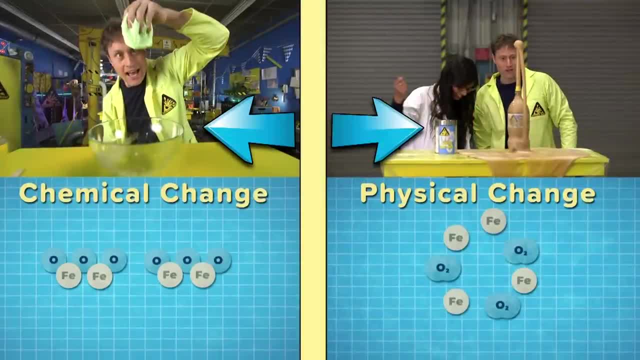 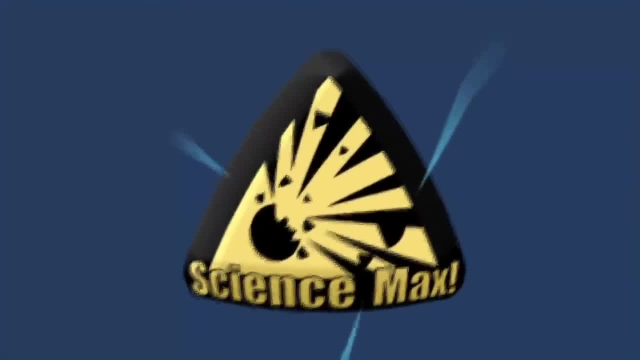 but whenever two things mix, think to yourself if it's a chemical change or a physical change. and now you know it's either one or the other, And that's the first step to good science. Our maxed out rocket worked great. Now to make it look more like a rocket. 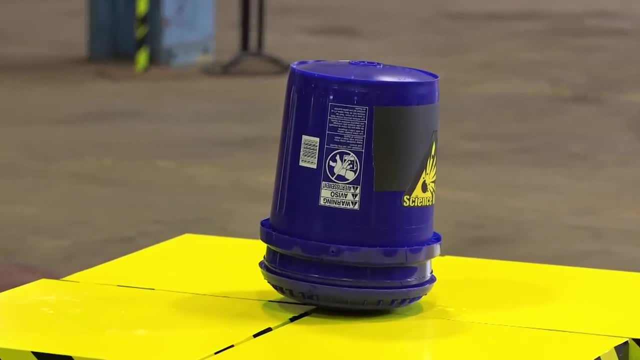 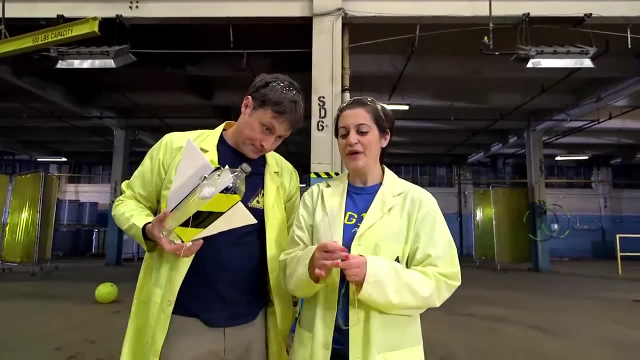 So we have a mesh bag here to put the antacid in Right, And we have some paper clips attached to it. And what are the paper clips for? Well, Phil, we have a magnet, Ah, And so the magnet sticks to the paper clip. 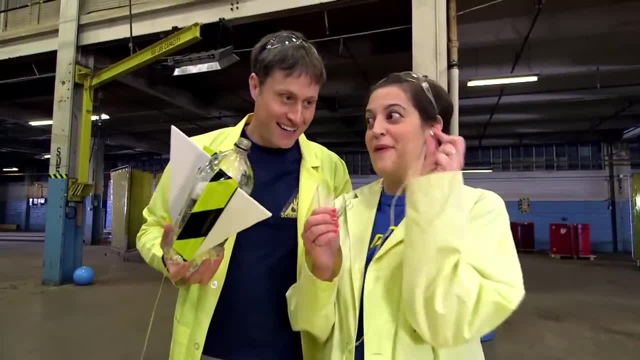 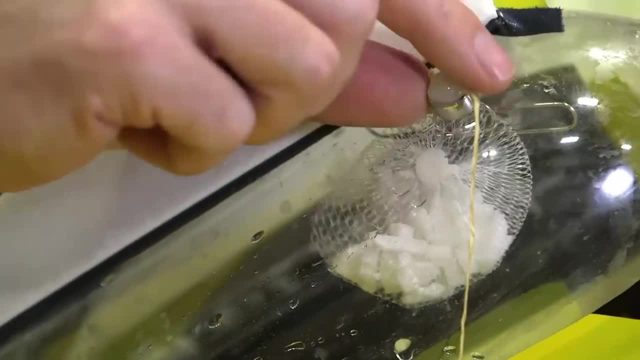 And so that's what we have here. You see, the bag is full and the paper clip is attached to it. And what are the paper clips for? Well, Phil, we have a magnet. We have a bottle of the antacid tablets. 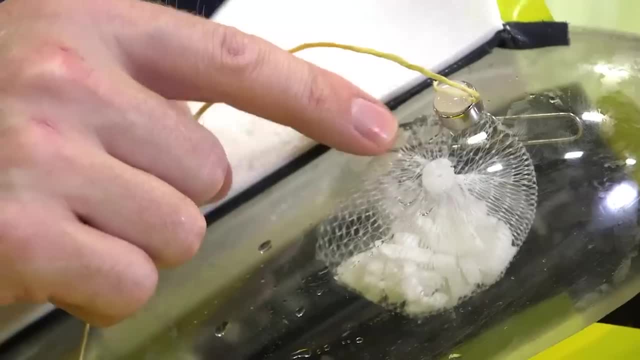 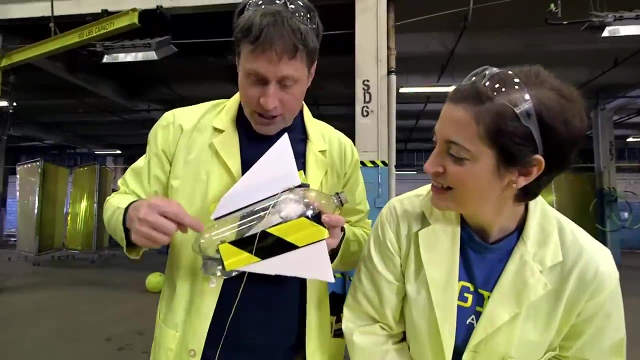 which we put through the mouth of the bottle, and the magnet is holding the paper clips on the other side of the plastic so we can sort of move it along, So we can start with the bag over here where the water's down there. but now we attach the launcher. 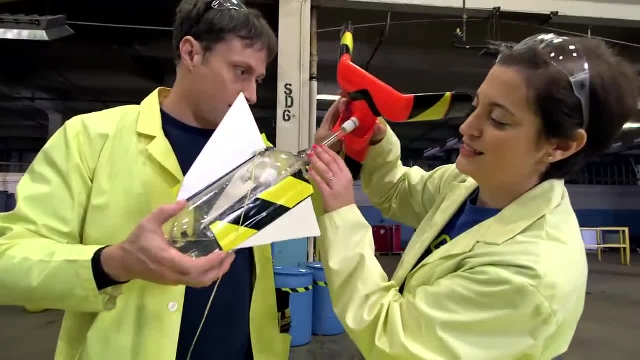 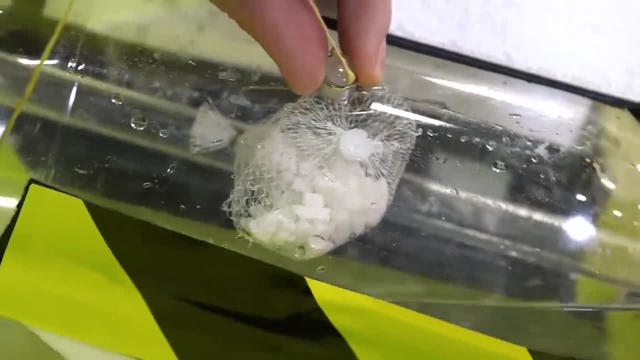 like. so All this effort is to keep the reaction from happening until the bottle's on the launcher and we're ready to go. And then, as we pull the bottle over, we bring the bag up this side, and there the water and the antacid have never touched. 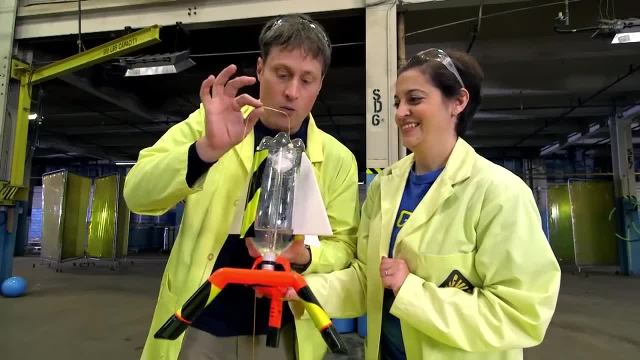 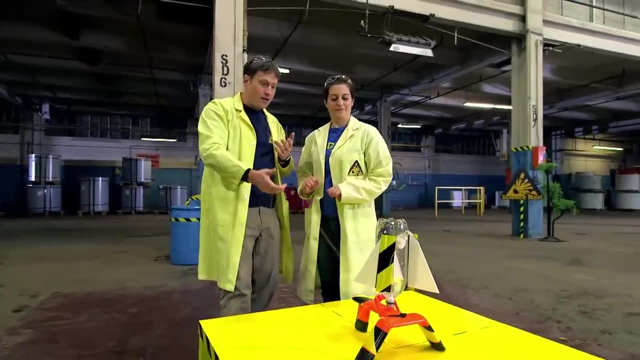 No reaction. All you need to do now is just we pull this magnet away and the bag will fall into the water, and then we will have the launcher down here and we pull the release and the rocket will go. We add some weight to the launcher. 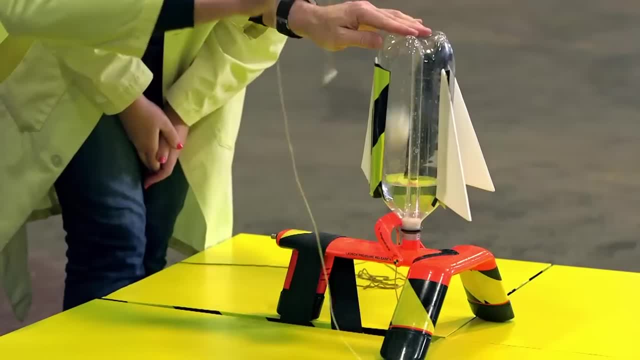 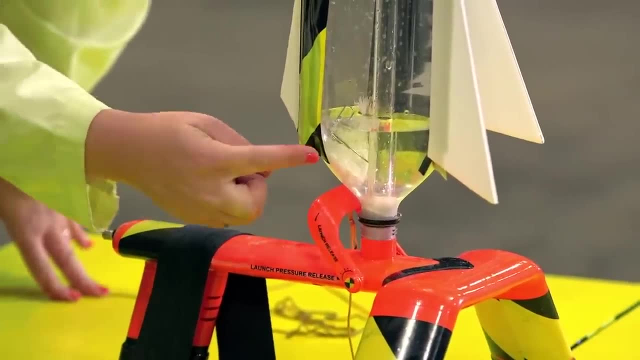 to help keep it in place. Okay, ready. And then we pull the string with the magnet that drops the bag of antacid tablets in the water and starts the chemical reaction. Because we have a latch holding the bottle down, we wait until the chemical reaction happens fully. 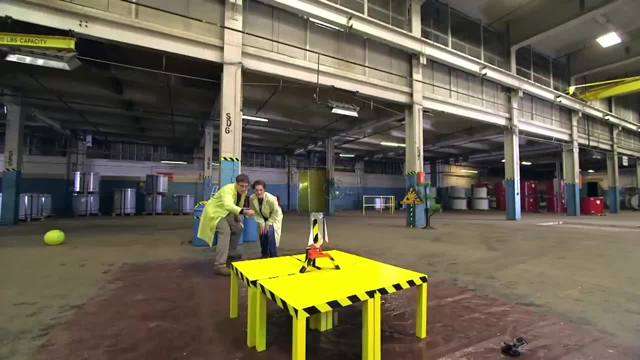 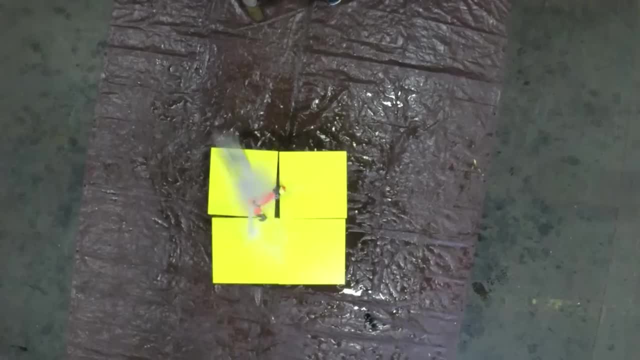 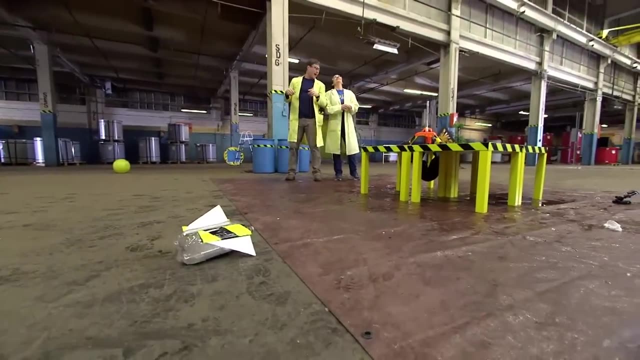 and there's a lot of gas pressure in the rocket. before Three, two, one Run. That worked. Yeah, I hit the ceiling. I think we need to do this outside. Yeah, I think we definitely have to do it outside. 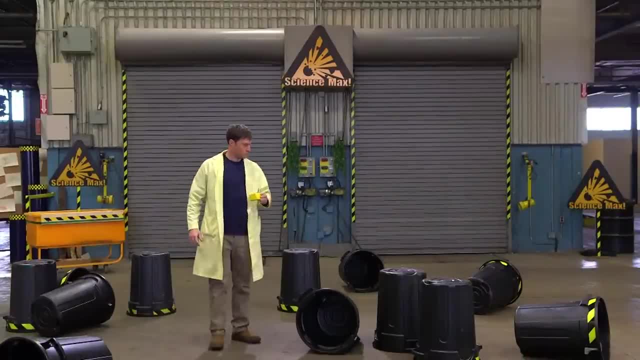 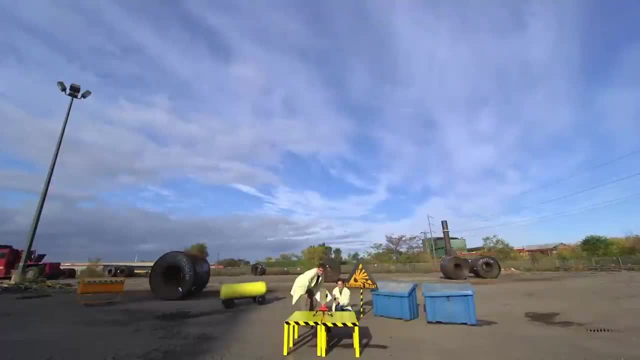 All right, totally great. Weird. We should put three or four, Three, two, one go There it is. Yeah, We tried it outside and it worked great. The only thing left was to max it out even more. 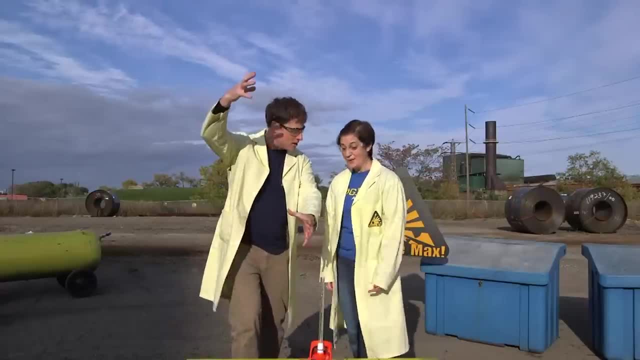 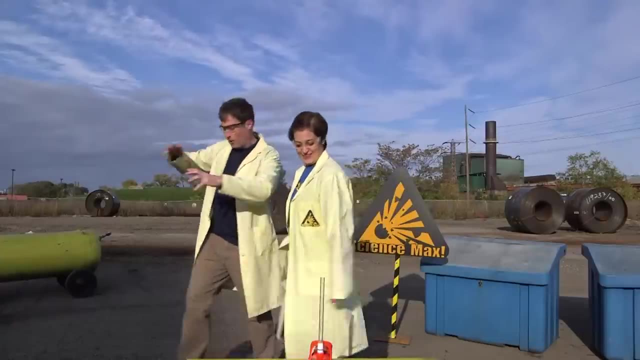 So: larger chamber, Yep, more antacid, More antacid, more air, more water, Absolutely Bigger rocket. Okay, so you know what? We can put two bottles together and we can increase the size of the chamber. 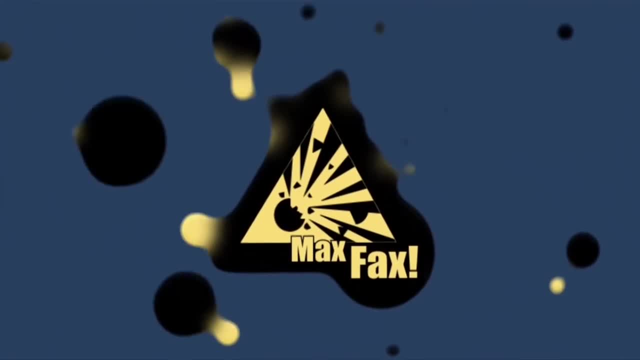 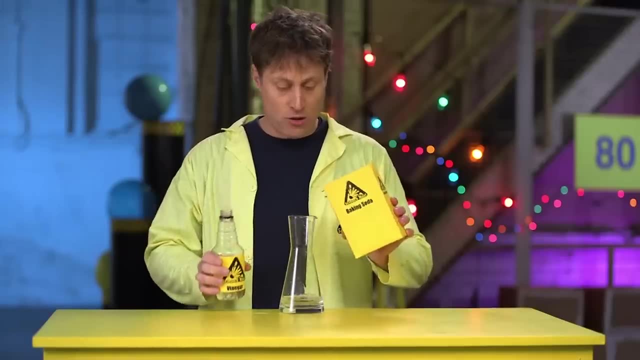 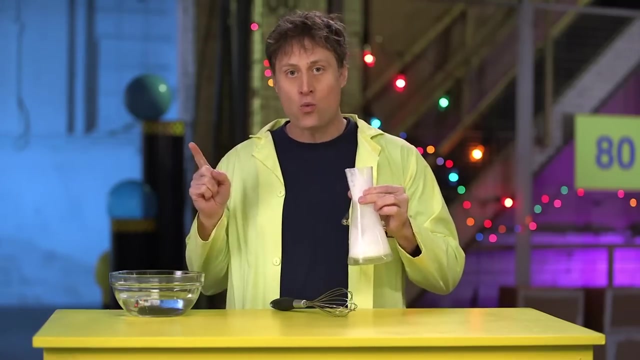 All right, This is sodium acetate. How do you get sodium acetate? Well, when you do a vinegar and baking soda reaction, what you have left, once the reaction is finished, is sodium acetate. It's a crystal and you can do something fun with it. 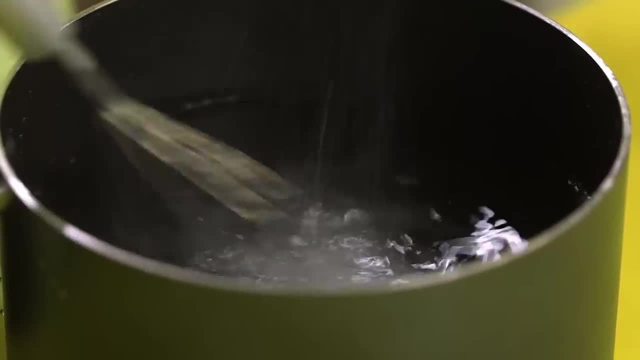 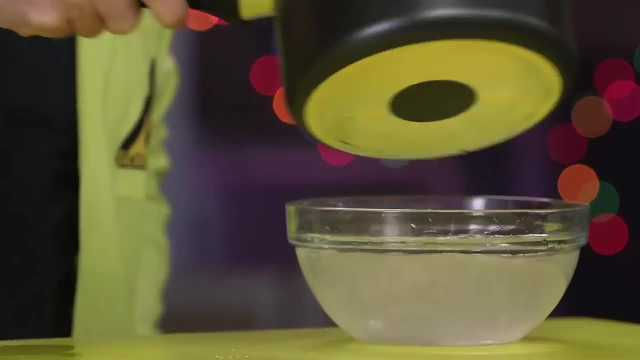 that may seem familiar. You make a supersaturated solution of sodium acetate by heating water and dissolving as much as you can, and then, when it cools, you can get the crystals to reform. Now, if you did this with sugar? 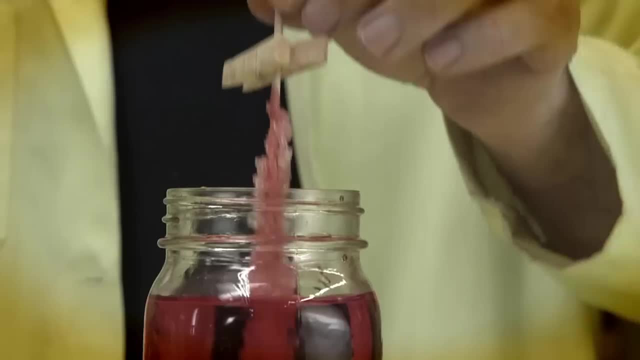 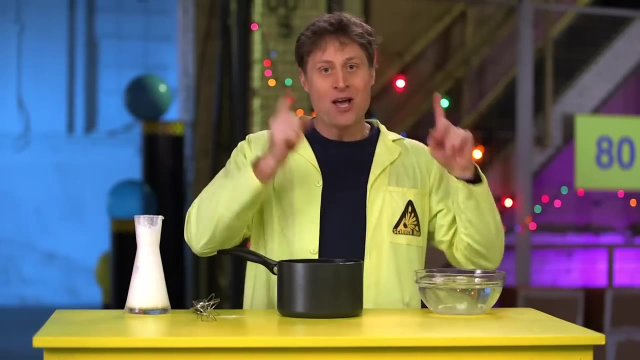 you could make a sugar pop, which we've done before. If you do it with salt, you could make a salt pop, which is less appealing, And if you do it with sodium acetate, you can do this Just like with the sugar pop. 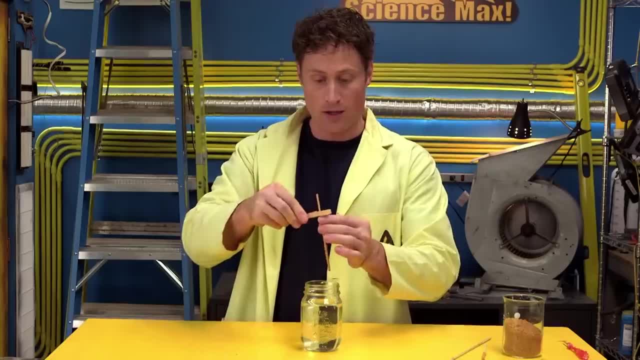 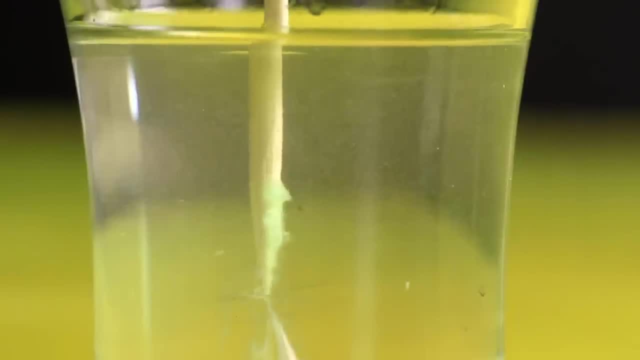 all it needs is a seed crystal to get the crystals to reform. But unlike sugar, which takes a few days, sodium acetate recrystallizes right before your eyes. Because we heated the water, it allowed more crystals to dissolve in it. 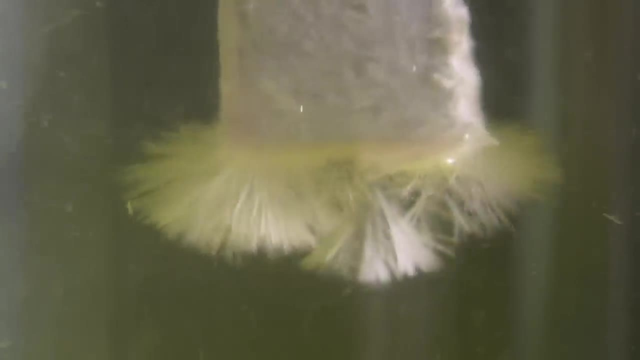 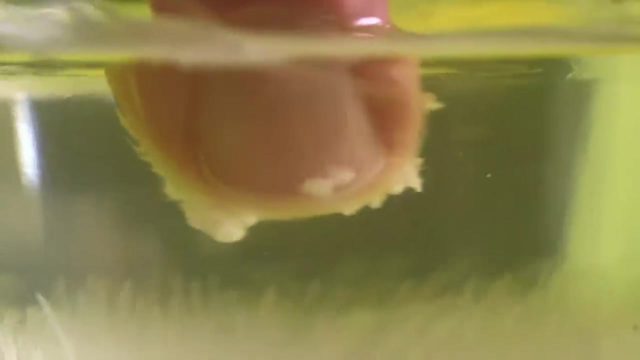 Ooh, But then it cooled down afterward. There's more crystals sitting around in this water than there should be at this temperature. They want to turn back into crystals, and all they need is something to start them going. I've colored this one green. 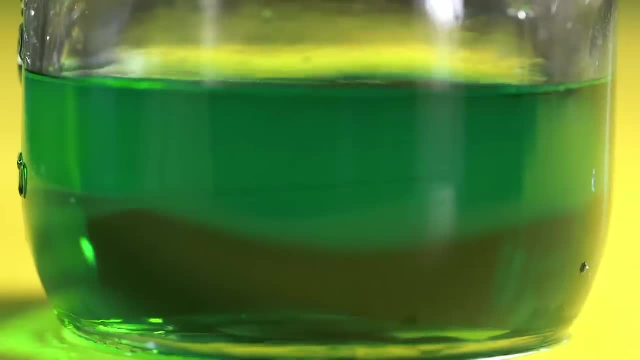 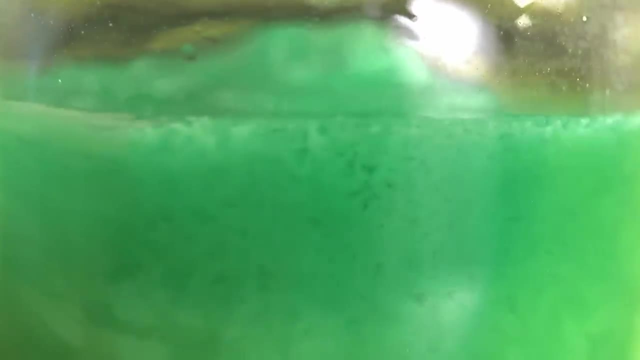 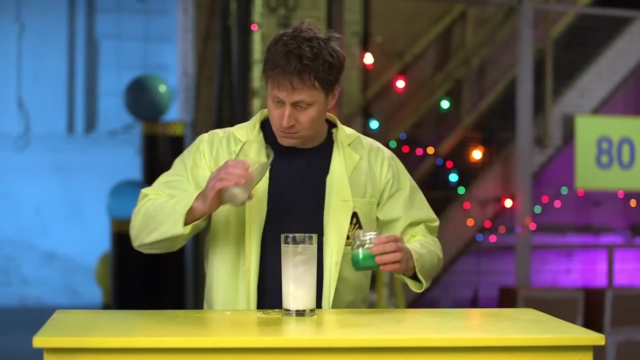 because I don't know science. Maybe it'll look cool. A tiny crystal on the end of the stick is all we need to start the reaction happening. Whoa, Wow, And there you go: Sodium acetate. Hmm, That one wasn't done yet. 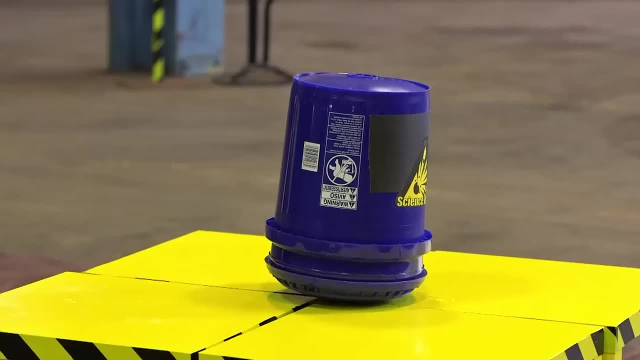 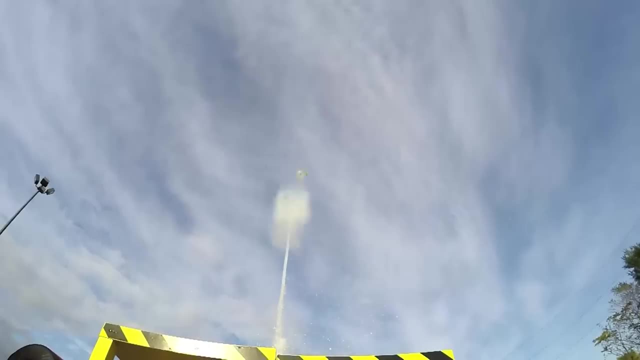 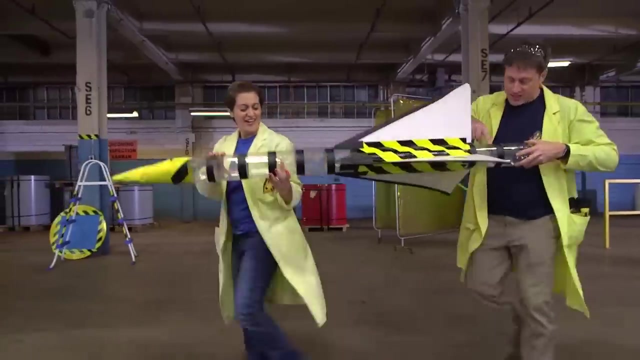 We've gone from small containers, Oh yeah, to a large container, Whoa. to a rocket, Yeah. So what's next? Super maxed-out rocket, 12 two-liter bottles all spliced together to give us a very large chamber. 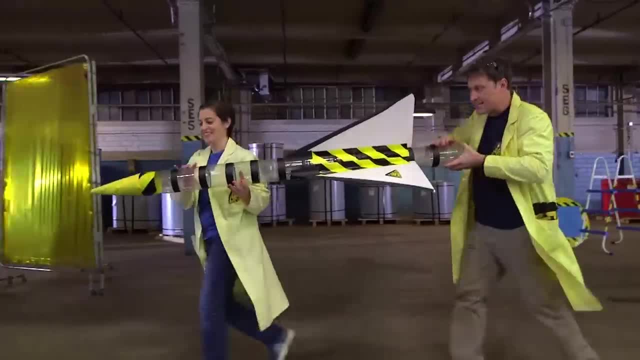 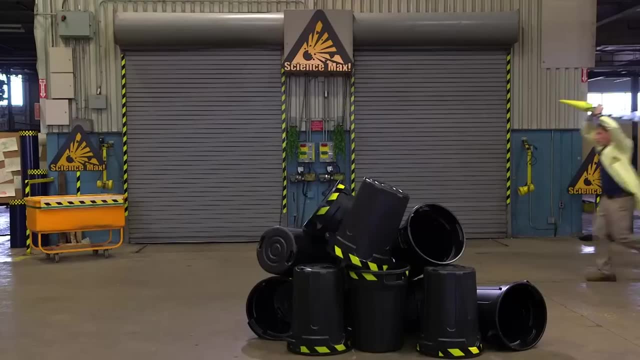 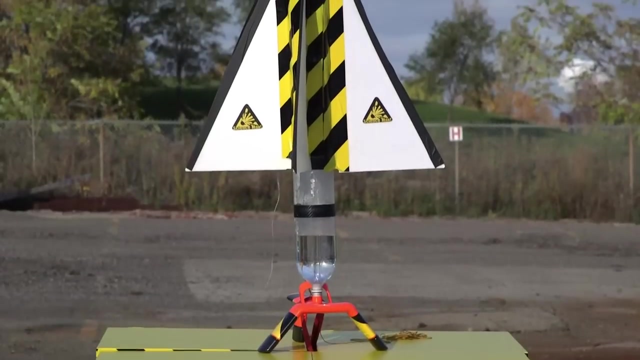 to build up pressure with. So the chamber is all the same. So it's all one big hollow tube and now we're going to fire it off. Let's go. Awesome rocket. Yeah, Lisa, and I follow the same procedure as before. 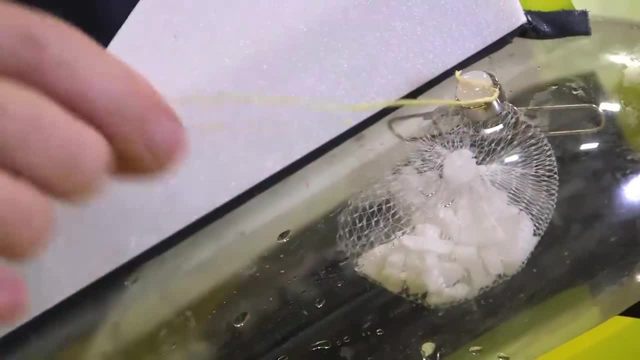 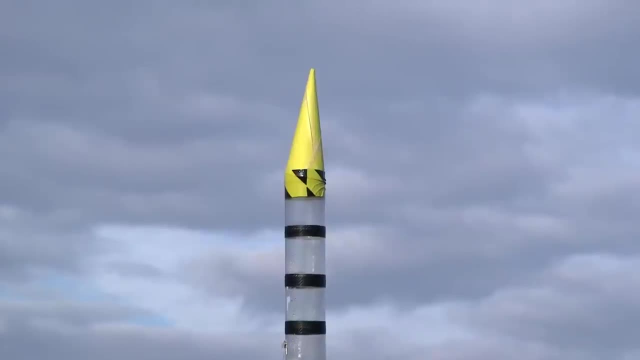 We use a bag of antacid tablets held up inside the rocket with a magnet And once it's sealed on the launcher, we pull it off. let the antacid mix with the water, let the chemical reaction happen for a while to produce enough gas pressure. 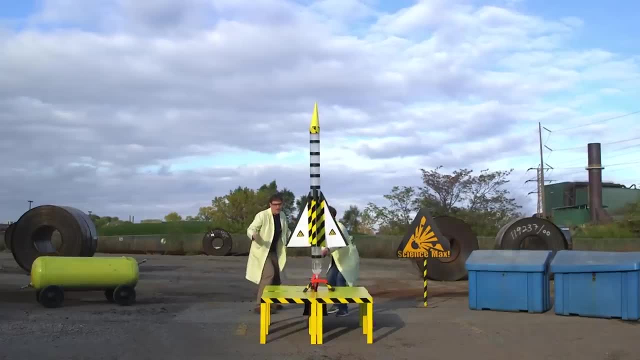 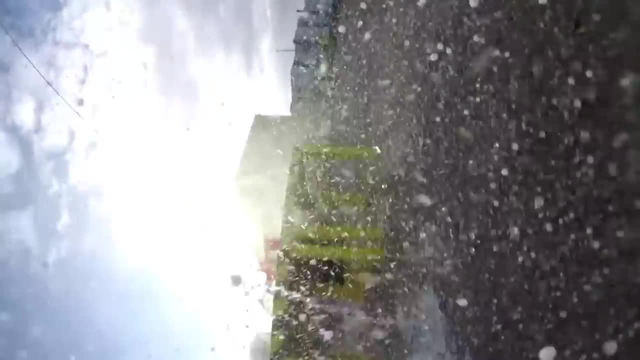 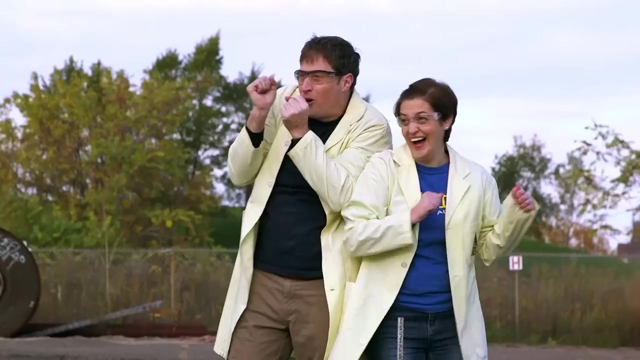 and then we fire it. Okay, here we go. Three, two, one go. Oh my gosh, Whoa. Oh my gosh, Oh no, Oh no, Oh no, Whoa. That is the highest I think you've ever shot. 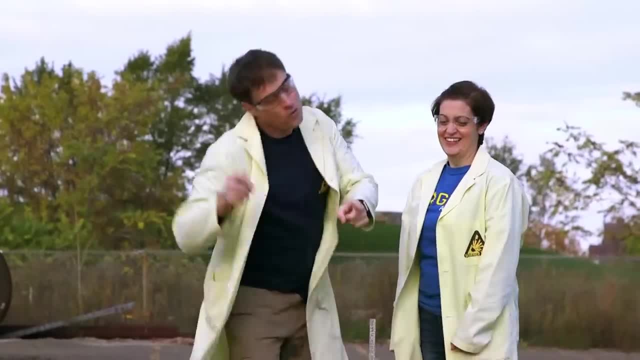 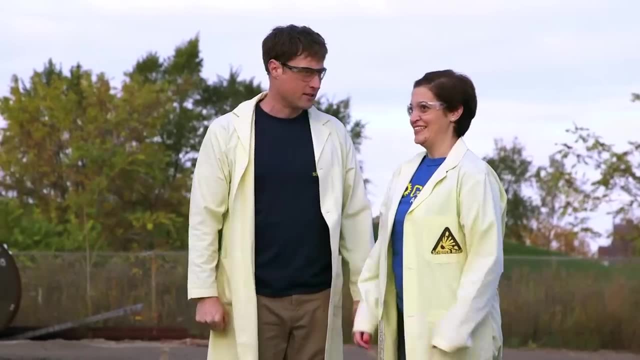 a rocket on Science Max. That's amazing, Well done Chemical reaction rocket. Thank you very much for joining us on Science Max Experiments At Large. We should build another rocket. I think so Because that one is probably broken. It's done. Okay, let's go, Let's do it.